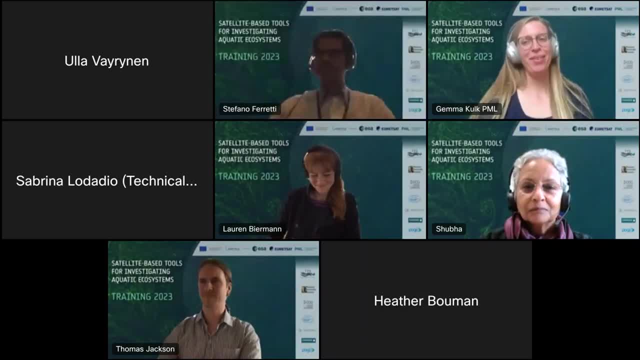 I'm going to start with welcoming everyone to the first lecture of the third module on ocean ecosystems and climate, So this is a new topic We're starting today. as usual, Please post your questions in the chat during the lecture and we will collate them, as as before, and ask the questions after the lecture, during the Q and a session. 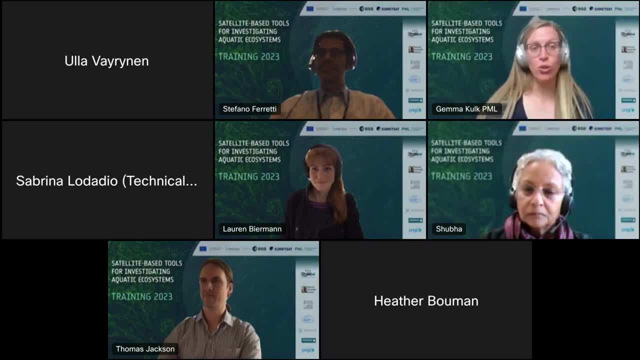 I would also like to remind everyone that we have a YouTube channel with all the lectures on there. You can subscribe to that and then you receive notifications whenever a new lecture is available, And I will post that link in the chat once we start it. So I have the pleasure of introducing Dr Marie-Helene Rio from the European Space Agency, who's about to join us. 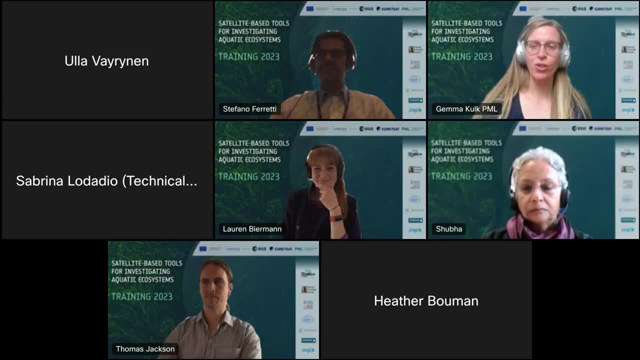 Marie-Helene has a background in space and she's going to tell us a little bit about what she's going to talk about today. Marie-Helene has a background in space engineering and ocean, atmosphere and biosphere sciences, and obtained her PhD in physical oceanography from the University of Toulouse in France. 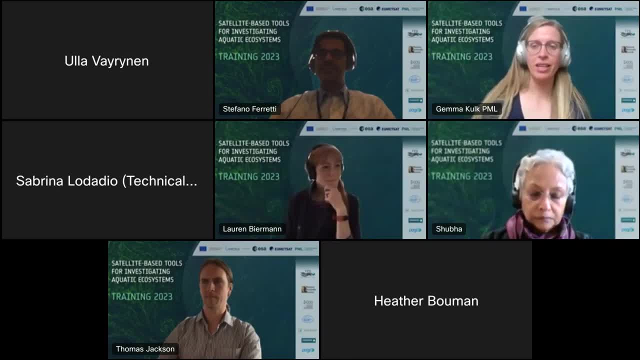 She has worked as a research scientist at CLS and at ESA and has received a Marie Curie fellowship to work at the Space Oceanography Group at ISAC-CNR in Rome. Marie-Helene is internationally known for her work on topography using altimeter and gravity data, and she also has a lot of experience in ocean color data for better retrieval of ocean surface currents. 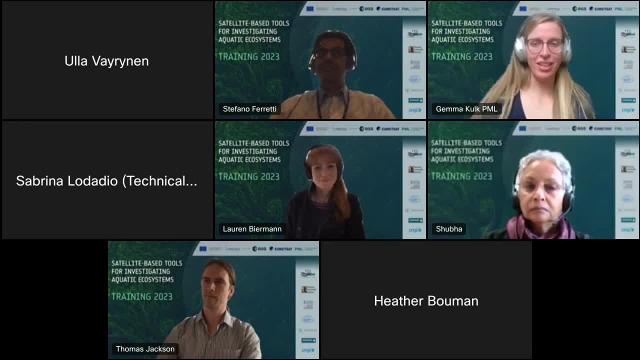 She will be introducing the activities related to ocean ecosystems and climate of the ESA's ocean science cluster, And I'm hoping that she will now come online. The meanwhile, maybe, while we wait, you can introduce Tom, Of course. so, while we wait, I can also introduce our presenter, our lecturer of today, who's Dr Thomas Jackson. 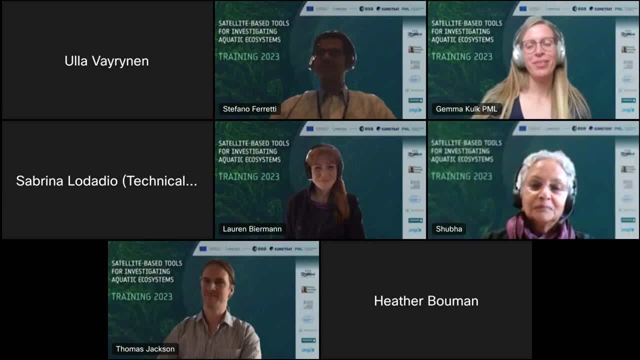 We call him TJ. TJ is a senior scientist at Plymouth Marine Laboratory since completing his PhD in earth sciences from the University of Toulouse in France, So we're very excited to have you on the itinerary from the University of Oxford. TJ has spent the last decade working on the creation and use of 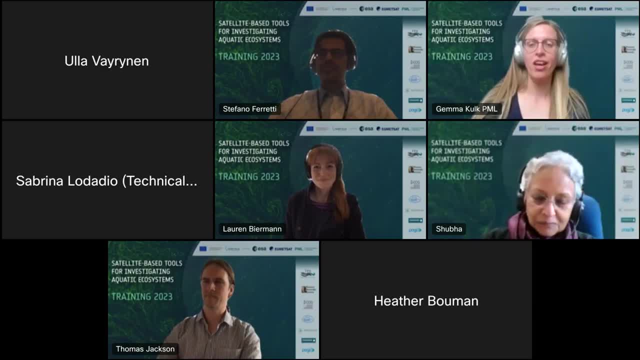 remote sensing data for ocean and climate science. This has included work on the generation and validation of ocean color products, the improvement of bio-optical algorithms and primary production models, product uncertainty characterization, the response of phytoplankton, climate forcing and the end-to-end processing and quality control of data for open climate data records through. 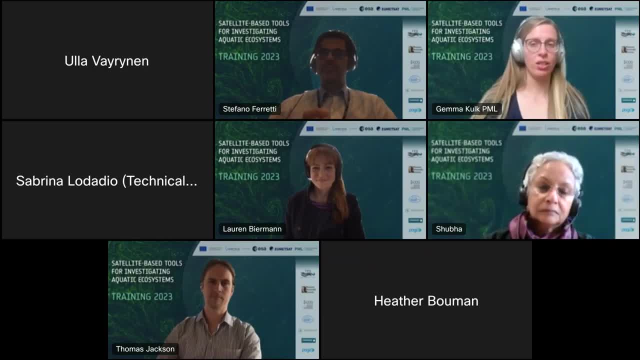 international projects such as the ESA Climate Change Initiative and Copernicus Climate Change Service. I see that Marie-Helene has not joined us yet, so what we could do instead is that we would have TJ's lecture first and the introduction by Marie-Helene after that. 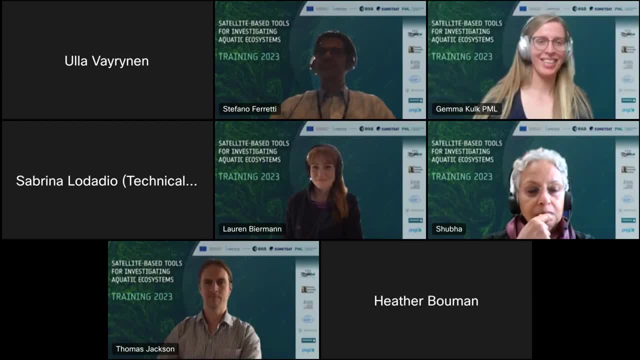 Okay, one second only. Okay, Okay, if Thomas can start, then she'll. as soon as she manages to get into the WebEx, she'll. then when, after Thomas she will, We'll do hers. okay, Okay, perfect. 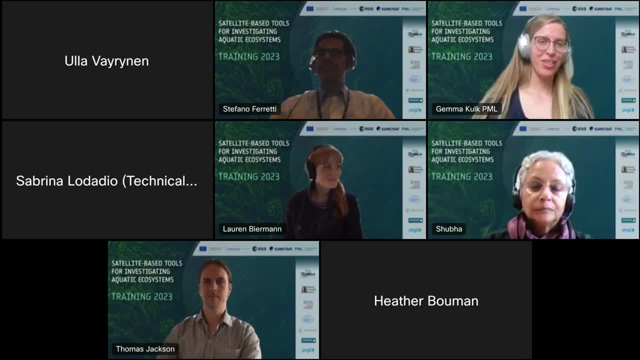 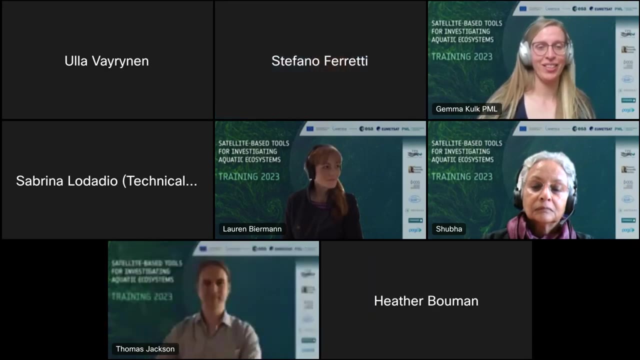 Thank you. So just to let everyone know, TJ will give his lecture first, and then Marie-Helene will follow up from the ESA site, and then we'll continue to Q&A. So, Thomas TJ, the floor is yours. 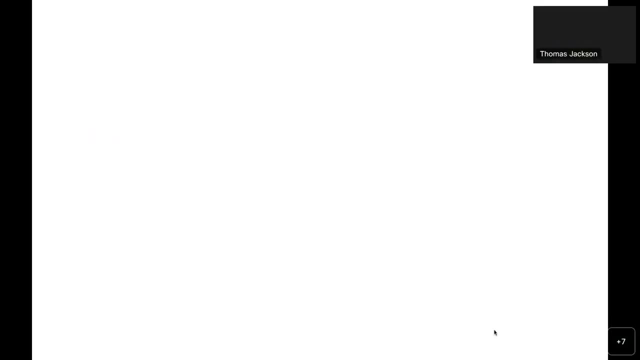 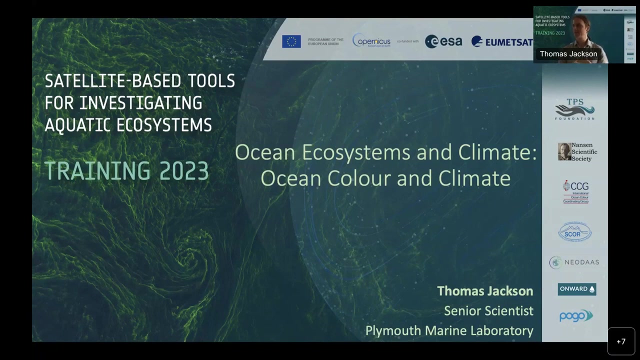 Okay, So hopefully you will all see, Okay, the correct screen. There we go, Right, So thank you very much. So, yeah, this is the first lecture in the new series of this set of four lectures on ocean. 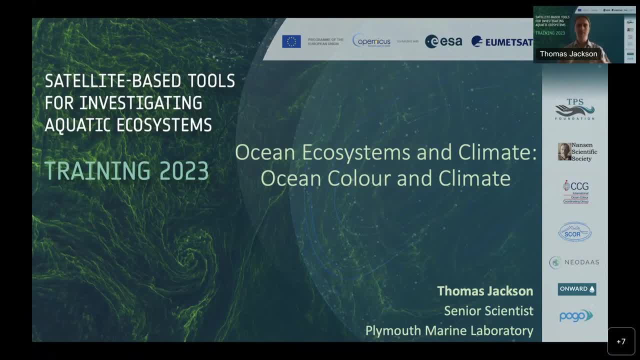 ecosystems and climate. So I'm Thomas Jackson from the Plymouth Marine Laboratory and although I'm giving the talk, there's a huge amount of work in here. I think if I put the full list of people that have been involved in all this work, it would fill. 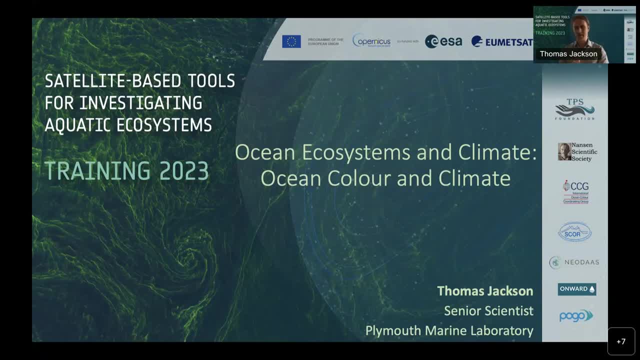 probably more than a slide, A full slide, But all the references that I give for the work and things I discuss I'll provide at the end in a big list so you can go and do further investigations and read a bit deeper into all of the material. 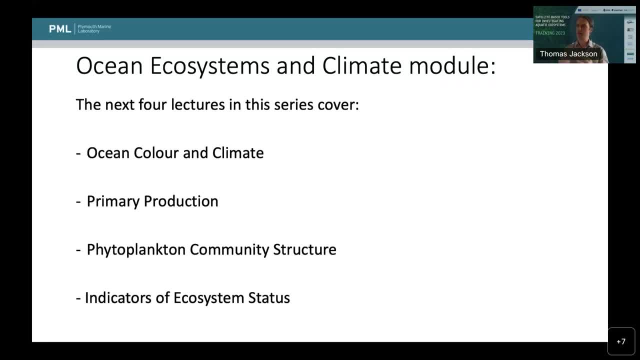 So quick overview of that, this module, this set of four lectures first, and then I'll press on with the main body of this lecture, So the next four lectures. we have ocean ecosystems, We have ocean color and climate, primary production, phytoplankton, community structure. 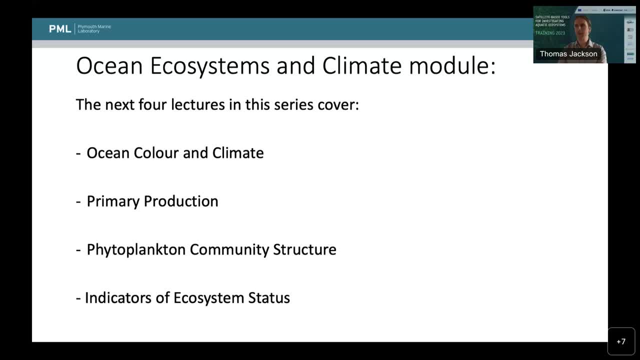 and indicators of ecosystem status. So this lecture is on ocean color climate and that I'm going to mostly focus on what it means to have a long data record, how you generate those climate quality data sets and then give a few examples of using those for what we might consider climate change. 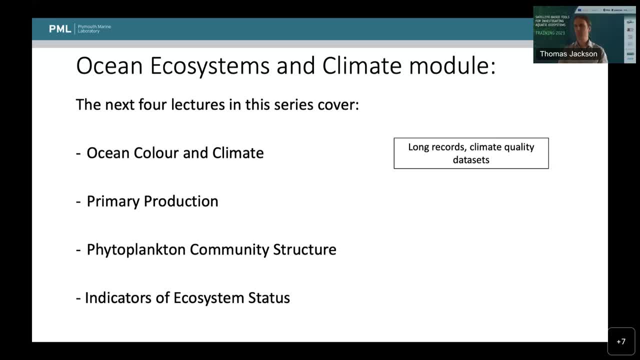 or climate investigations. The second lecture is on climate change. So the second lecture, following this one, will be from Bob Bruin and that's on the carbon cycle. So he'll talk about the carbon cycle from the perspective of ocean color and also look. 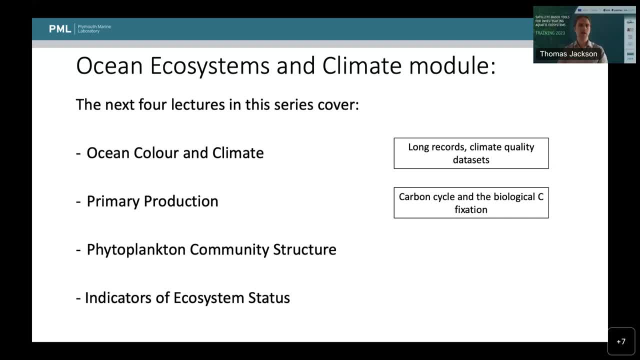 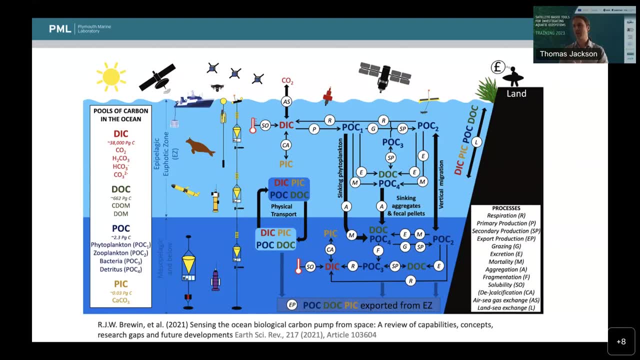 at biological carbon fixation in the ocean. So just a little teaser for that. It's quite a complex system. There's a lot of different pools of carbon in the ocean and they have it's got quite a rapid turnover from the biological side, which he'll go into a lot more detail about. 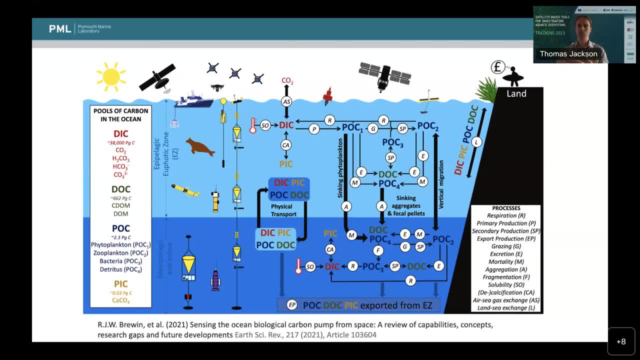 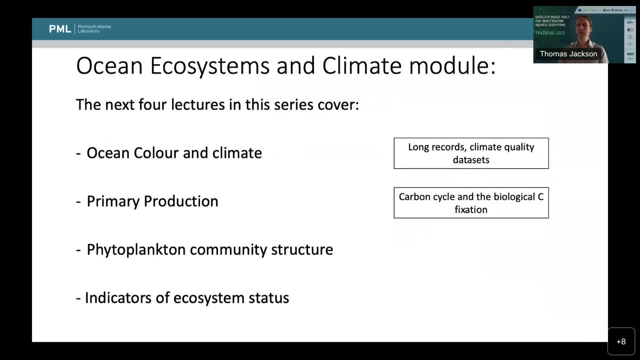 but anything where I mention primary production or carbon fixation. you can expect to get more information in next week's lecture. The third lecture will be from Dr Heather Bowman and that will be focusing more on the diversity. So once we've looked at climate first and then the carbon cycle, then we'll drill a. 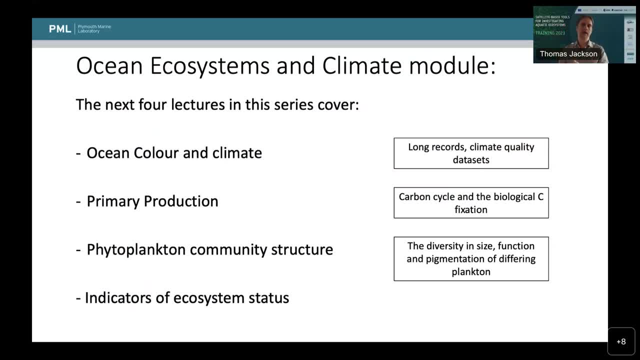 bit further down and have a look at the diversity in the size and the function and the pigmentation and characteristics of plants. So there's a lot of different types of plant and that make up this community structure and how that varies across the globe and in different environments. 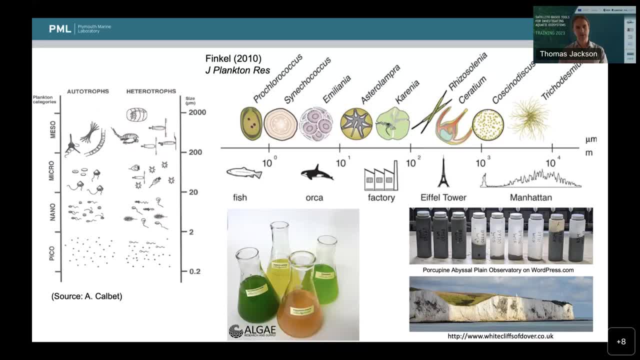 So one part of that is that the algae have different colors, as you can see in the bottom figure here with the different vials, but also looking at things like the enormous range of sizes that you get in phytoplankton, So from things like the cyanobacteria which is Prochlorococcus, here on the left of the 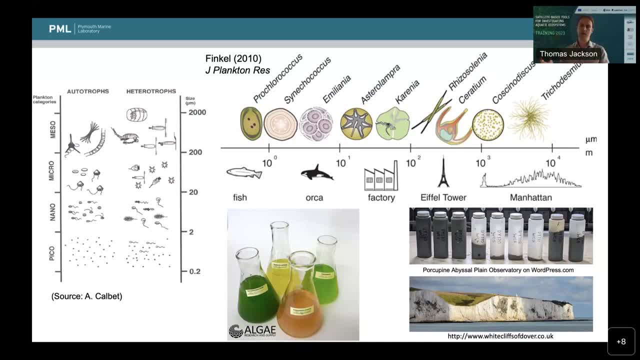 top figure And then through to things like Trichodesmium, which are colonial. there's four orders of magnitude or five orders of magnitude in size, And that's the same as going from a single fish to the city of Manhattan. So it's really you can't consider these organisms often as a single type. 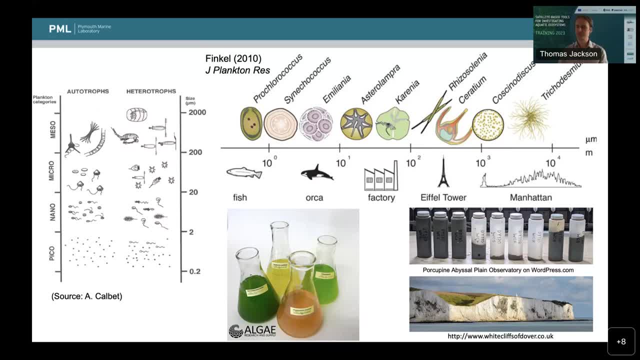 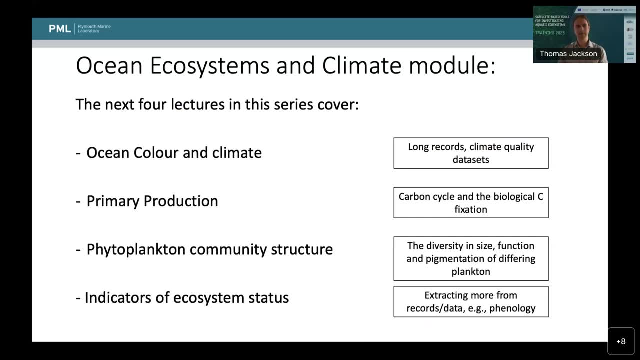 We have to segregate them in different ways. So, then, the last one in the series will be from Dionysus, and that's going to be looking more into once we have these records And we understand what's going on in them in terms of carbon or in terms of phytoplankton. 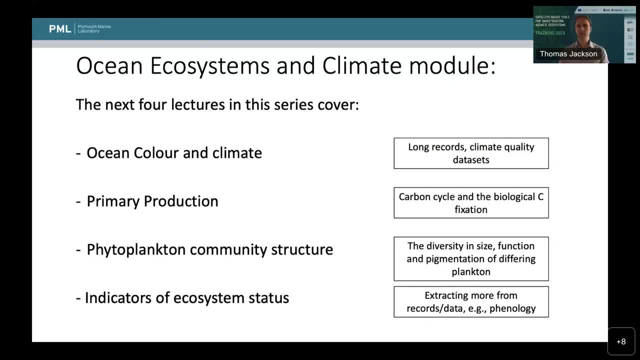 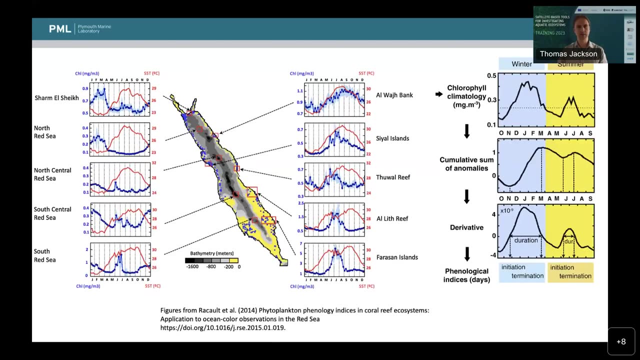 groups or functional types or biomass. How do we extract a little bit more information from those records? So that will be things like E-metrics or phenological indicators and getting a bit more information out of the time series records. So here's an example from some work that Dio did with Marie-Fanny Racot, and this was: 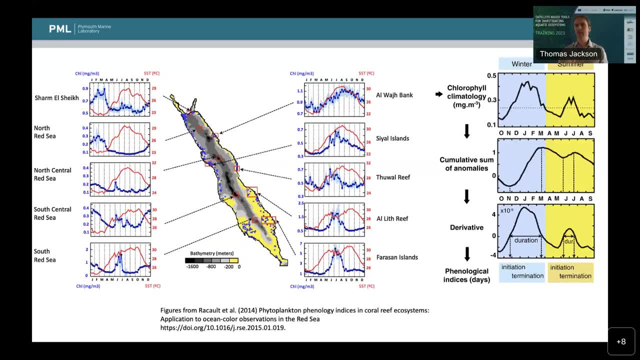 looking at the Red Sea And you can see in the left side of this we've got just regional extractions of time series. The red is temperature and the blue is chlorophyll And you can see that they have some seasonal cycle across the year. 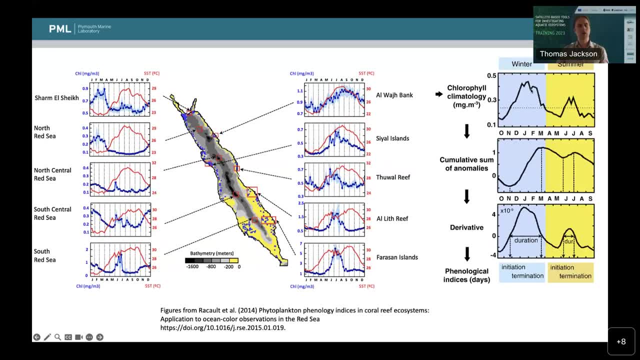 And then, when we talk about phenology, what we're doing is we're trying to extract metrics which represent those sorts of features in time, So that might be the duration of event, The peak Amplitude of an event, Or the timing of an initiation of an event. 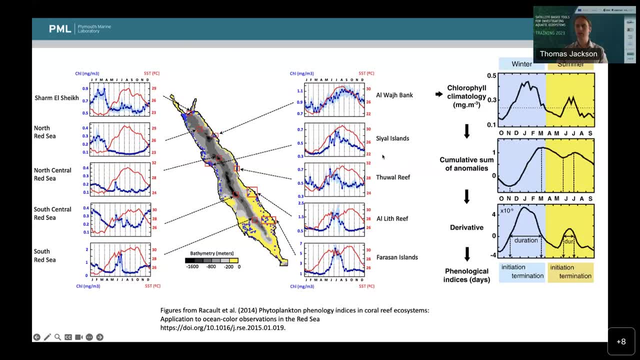 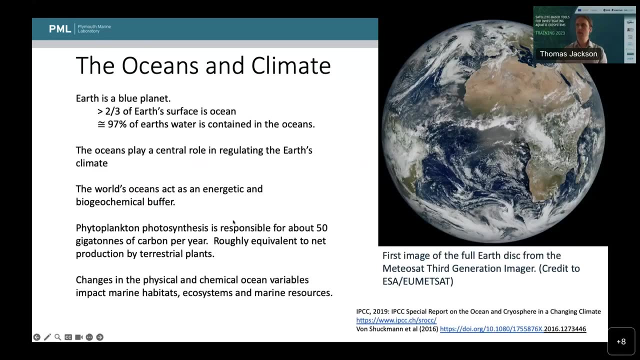 And so Dio will dig a lot more into that and also relate that onto things like fisheries and higher trophy levels. So back to the oceans and climate, which is the main topic of this lecture. So the Earth is a blue planet fundamentally. 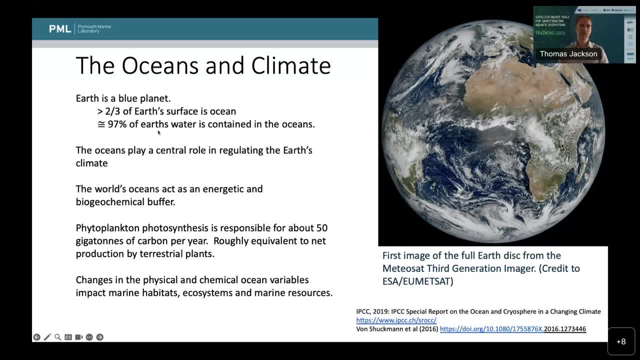 It's two-thirds covered by ocean And around 97% of all Earth's water is in the oceans, And the oceans play a key role in regulating the Earth's climate, So not just in terms of them being a huge source or vector for heat. moving from the 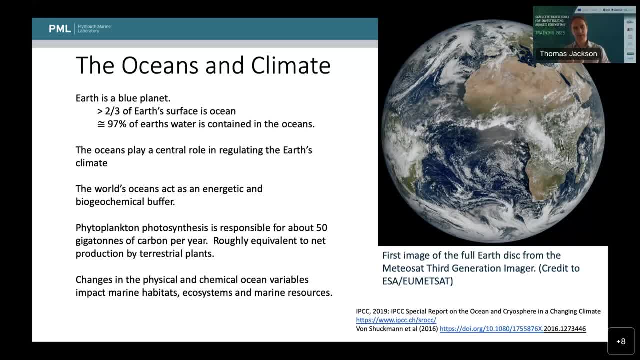 tropics to the poles, but also with things like dissolved gases. They really are kind of a buffer. They're a key player in the whole system. So over the last 50 years, although there's been a lot of warming and there's been quite 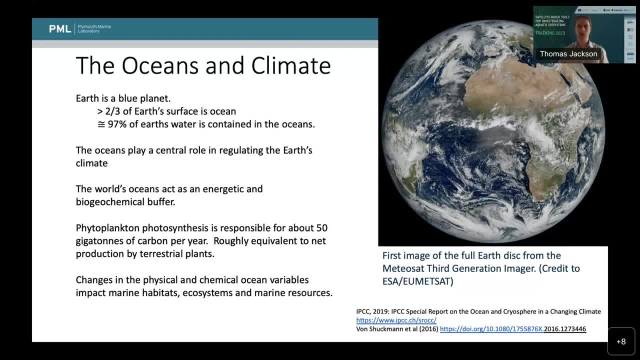 a lot of interest in, say, air temperatures over Europe or Africa or other areas of the globe. 90% of the excess heat from the warming of our planet has actually gone into the oceans, not the atmosphere, And during that time they've also absorbed around 30% of the anthropogenic CO2. that's 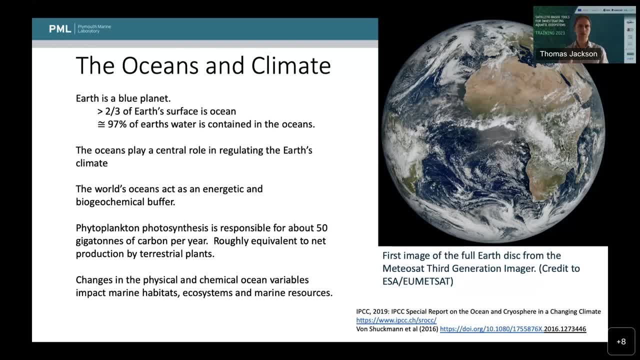 been emitted. So without the oceans having this buffering effect, temperatures would have risen much more in the atmosphere and the CO2 levels would be even higher than they are now. Additionally so, beyond just the physics and chemistry of the gas exchange and the heat, 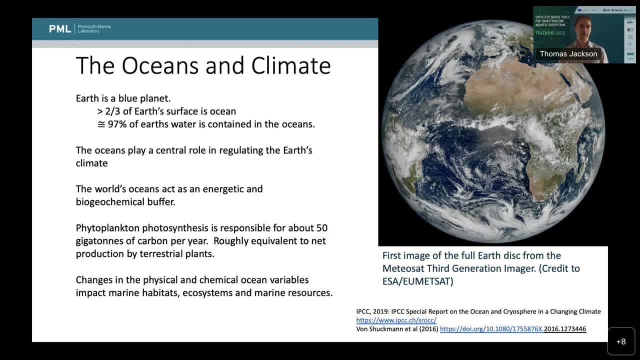 transport. phytoplankton in the ocean are responsible for roughly half of the primary production on the globe, So they are equivalent to all of the terrestrial plants Basically- I believe Schuber mentioned this before- And so any changes in the physical and chemical ocean variables can impact on the marine habitats. 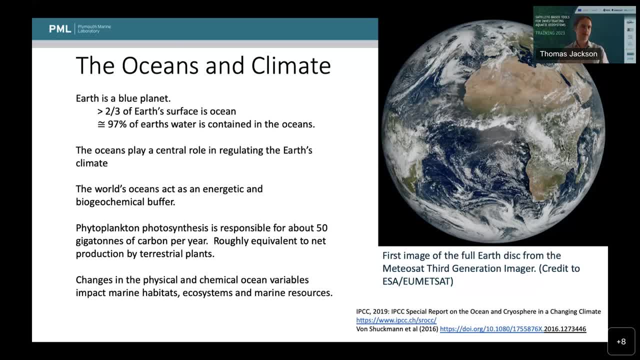 So we know that things like increased temperatures or increased acidification of the oceans have direct impacts for things like coral reefs, but they can also have impacts on other marine ecosystems and marine resources, And we know that there can be large variations of phytoplankton production in the geological 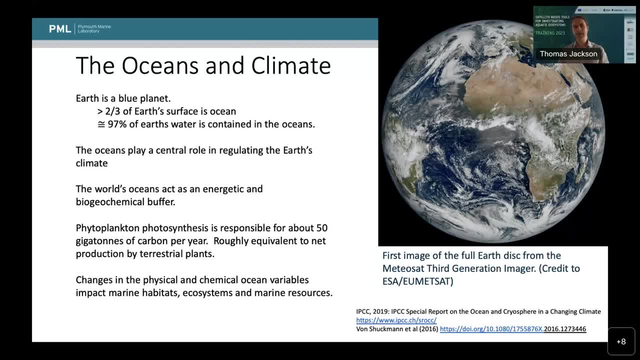 record And in fact, when we think about carbon on very long timescales, on geological timescales, pretty much all of the oil that we're currently extracting as a fossil fuel originally is sourced from plankton that were buried in the oceans And this is a beautiful picture on the right here from the ocean. 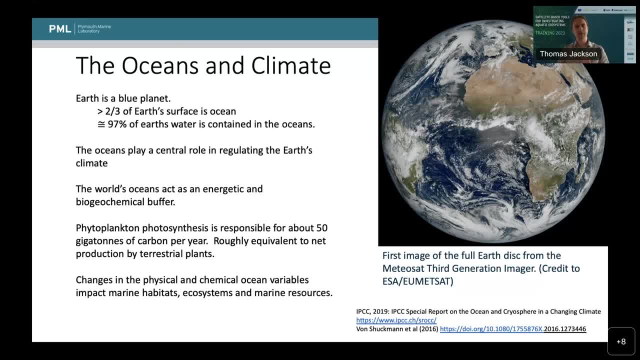 Meteor stats showing Africa and Europe and a large section of the Atlantic. But I'd also like to just show another image from the Pacific, because this is the European or the Eurocentric view, is one that many kind of have stuck in their mind as a vision of Earth. 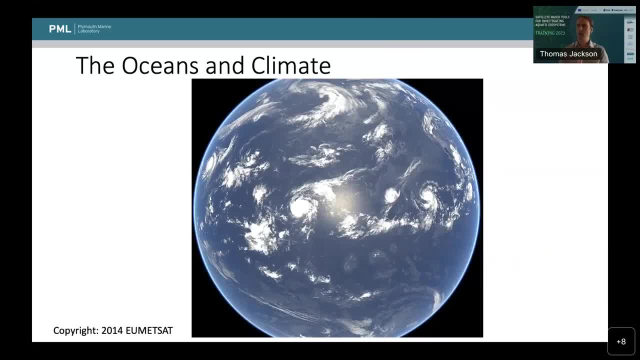 But really, if we look at it from the Pacific, you can have a hard time here trying to find where the land actually is. So you can just about see California over on the top right here. But really this is much more of a representative picture of the blue Earth. 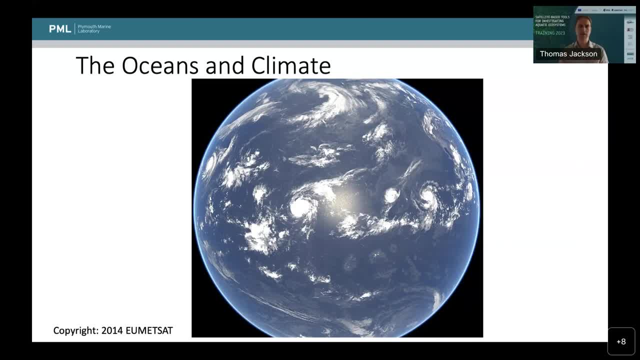 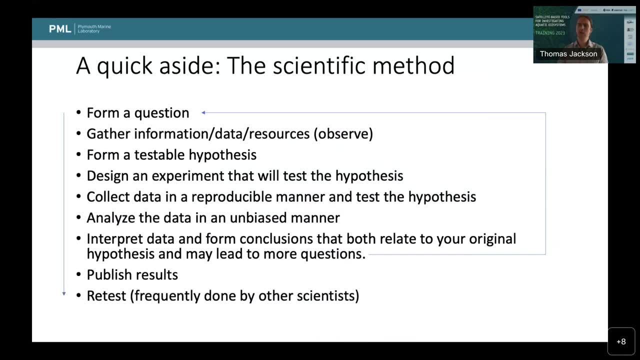 So the Pacific centric view really showing how much of the surface is covered by ocean. So, before I really dig any further into that and we start to look at how we might create climate data records, I think whenever we're asking questions- and we've seen this through- 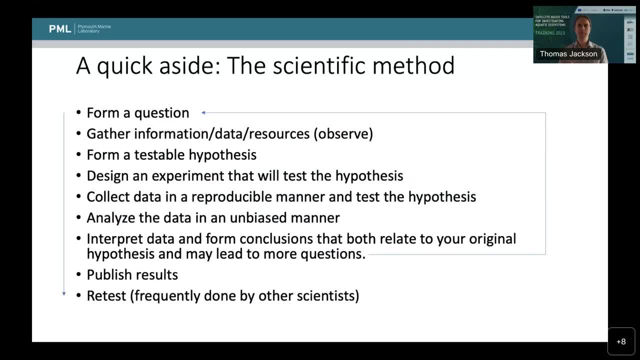 all of the lectures in this series so far, Where we have questions coming into the chat as we go through and also in the Q&A session at the end, We have to think about how we form questions and then how we answer them. So the scientific method in general starts with questions. 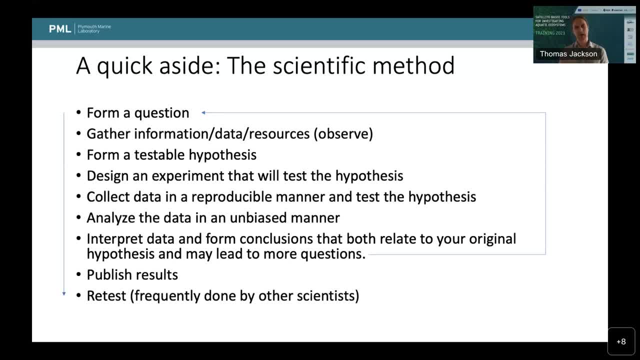 We have a question that we don't know the answer to, We have to go and gather information form some sort of testable hypothesis, because if it's not testable we can't get a truth or increment towards the truth with our investigation. 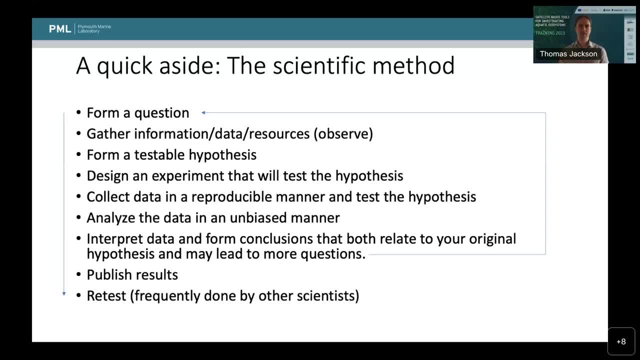 Usually that involves designing some sort of experiment- or, if not an experiment, some exercise- as a testable objective, And then you go out and you test your hypothesis And once you've got your data and you've analyzed it, ideally in an unbiased manner, you interpret: 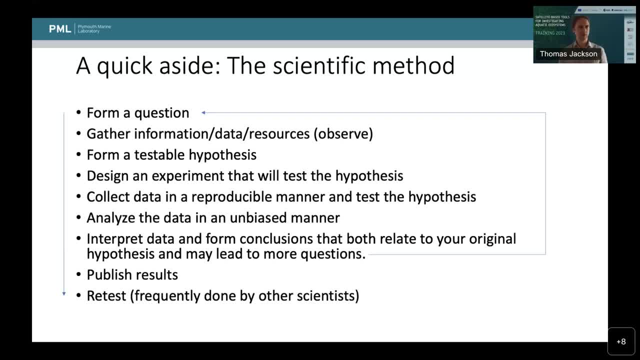 that data and form conclusions that you can share with the rest of the community, And often that's the point at which you just have more questions, And that's part of the joys of science: With every answer, sometimes you have another thought and another question. 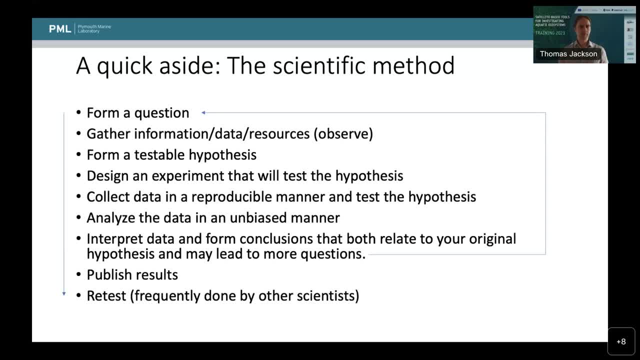 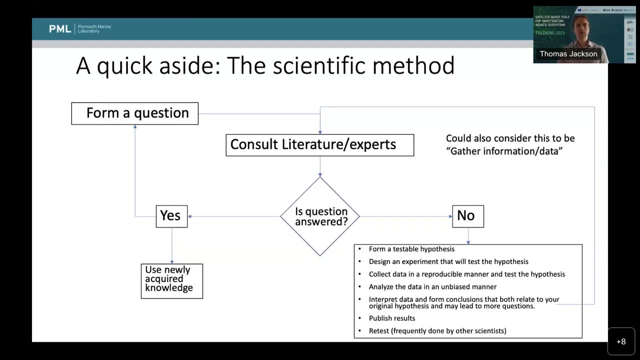 And you can go around that loop a number of times. Ideally, you can publish your results and then your results can be retested by the rest of the scientific community, adding credence and validity to those results. So really, by joining and coming to these lectures, you're already in part of this flow. 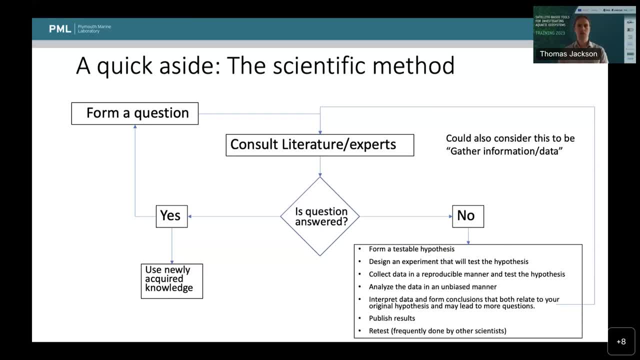 You have questions, You are consulting questions, You have questions, You are experts And through the lectures that we give, seeing summaries of the literature and the current state of the art, And hopefully that's answering some of your questions. So then you enter the yes and you can go and use that newly acquired knowledge. 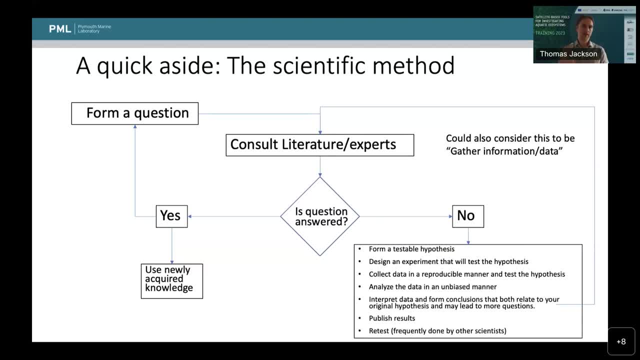 And ideally, you know, when we get to the end of this whole series, you'll feel empowered to go and form new questions and really push things forward in your own areas of interest, And ideally that means you'll end up going down the no path here. 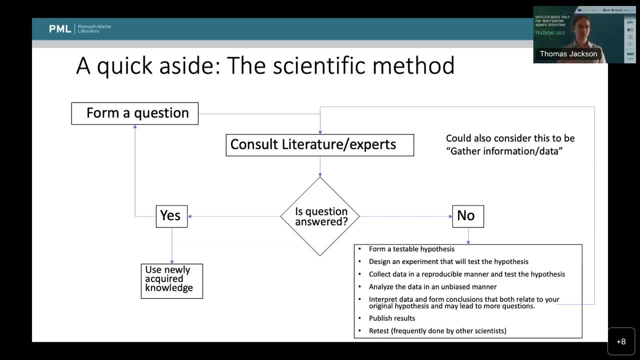 You'll have a question that we haven't been able to answer, but we've tried to provide the tools for you to answer that yourself. So in that case, you would then follow on down the path of working out how you might test your question, or test a hypothesis about a question, and get to some results. 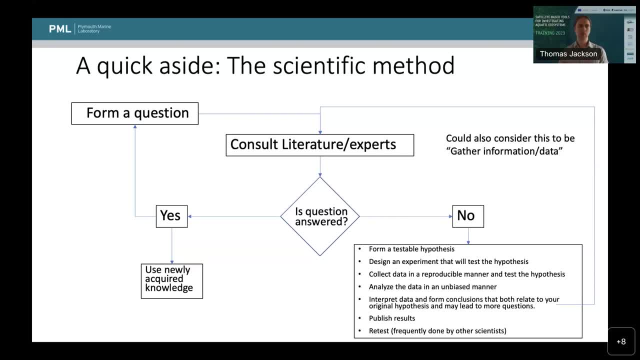 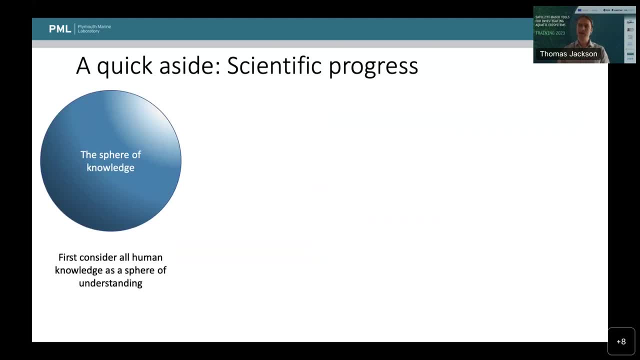 And we'll go over that process later with a few worked examples in the climate realm. And really I think I would like to view this lecture series as just helping to kind of expand your sphere of knowledge relative to the total sphere of knowledge. So this is just an aside, but for me it's how I visualize the learning process. 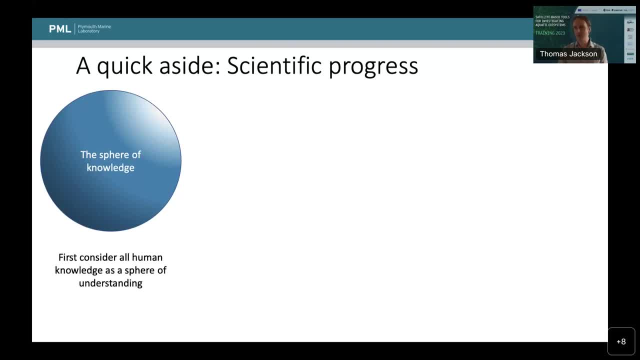 If we consider the whole sphere of human knowledge, at any point within that you can consider starting at the center, knowing nothing, And as you learn more you progress towards the edge of understanding. So that edge of that sphere And the direction that you're traveling in from that center is just a different topic. 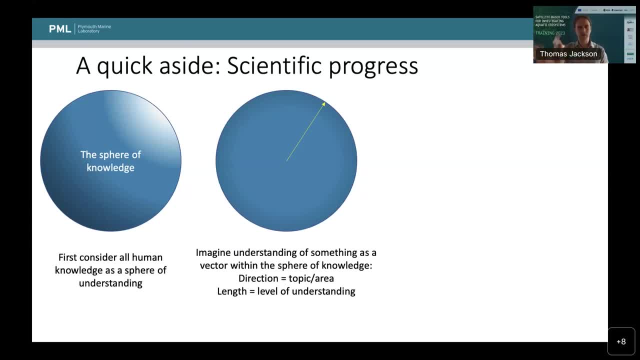 So, whatever you're learning about, you're pushing out towards more and more understanding and the limits of that knowledge. And once you reach the edge, once you get to the edge of that level of human understanding, you work, and you work, and you push, and you investigate and hopefully you push it out a bit further. 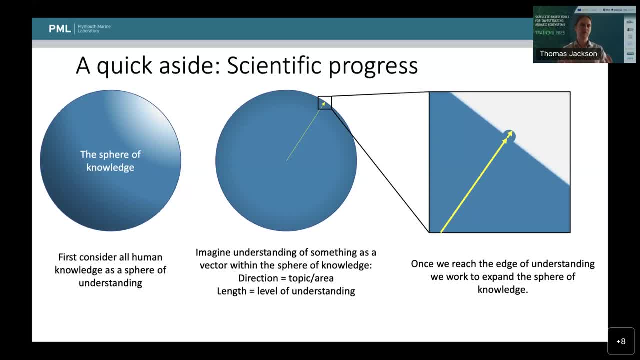 And if everybody does this across all of the fields of science and investigation, then the whole sphere grows increment by increment, piece by piece. But this is not always a linear path. In fact it's very rarely a linear path. Normally you're learning about one topic, say ocean color, and you find out you have to go and learn about something else. 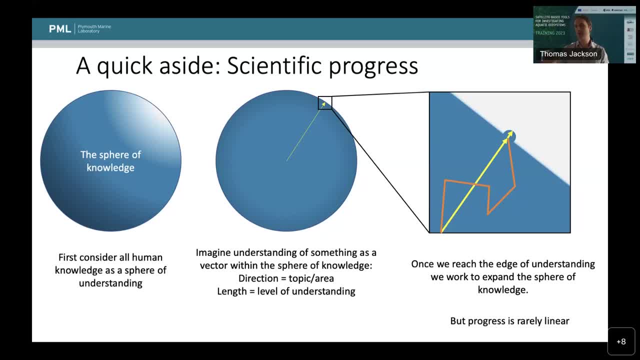 perhaps for your transforms, or sediment dynamics, or atmospheric processes or I don't know, light propagation. There's all sorts of other little things you want to go and learn about, And eventually that brings you to the point that you need to be at the edge of human knowledge. 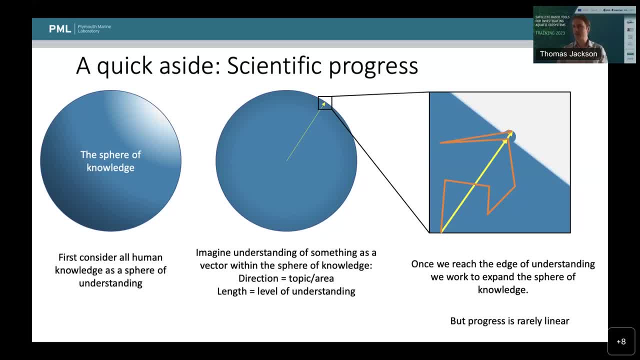 And, through my experience, normally that's the point at which you really have to take another deviation and you're pulling information from a different area of science or from a conversation with someone who works in a related field And that will help you make that bounce, that step out and push knowledge a bit further. 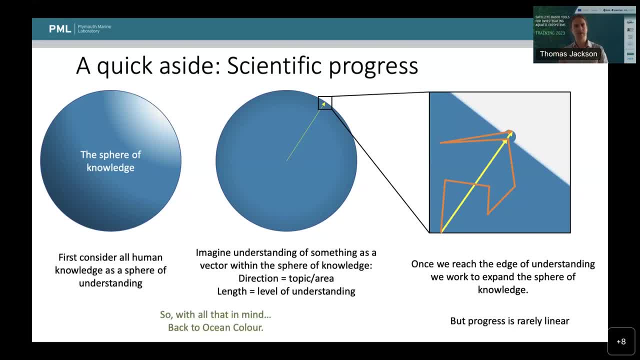 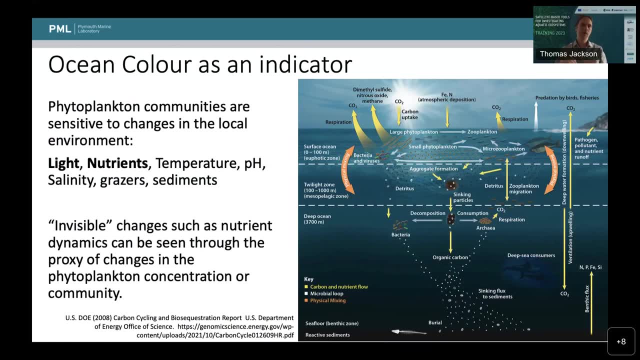 So anyway, with all that in mind, about how we ask questions and how we make progress, back to ocean color. So ocean color as an indicator. Really, this has been mentioned a number of times in the introductory lectures from Lauren and from Anna. 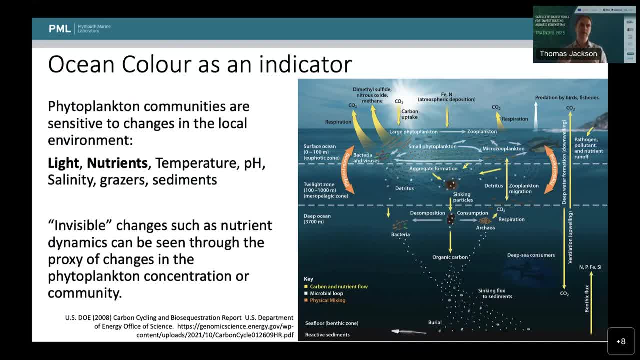 But so phytoplankton are sensitive to their local environment And the figure on the right here shows a lot of connections basically between phytoplankton and bacteria and light and nutrients And all sorts of ocean processes. But the most important fundamental drivers for phytoplankton growth are going to be light and nutrients. 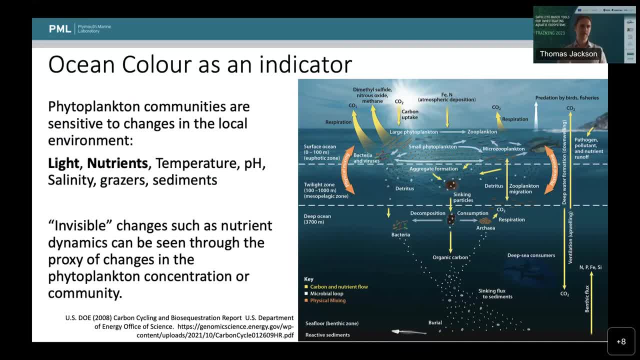 because they're photosynthetic organisms, So they need light in order to photosynthesize and they need nutrients in order to synthesize new organic matter. Once they have those, then factors like temperature or pH or salinity, the presence of grazes or sediments which might block the light, and things like that. 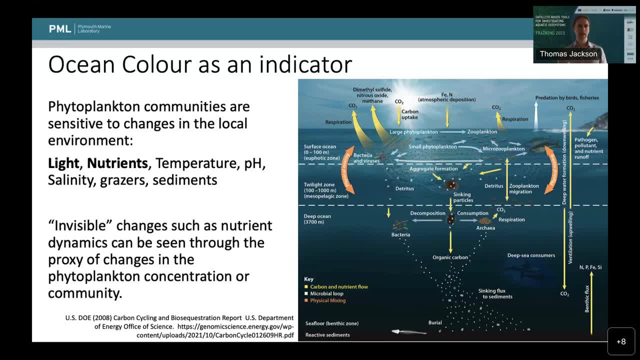 will also have secondary implications And that's going to have impacts on their ability to grow and flourish. But what that means is when they are growing- and we can see them because they have this optical signal- they can be reflecting invisible changes that we couldn't see. 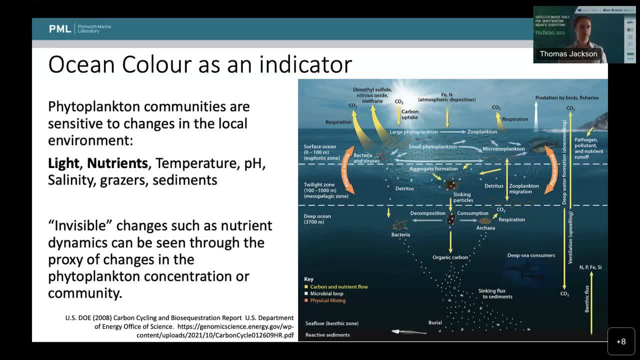 So we don't yet have the ability to map some nutrients from space, like nitrate or silicate, But if we see a particular phytoplankton growing in abundance, then that's probably due to a response that they have to the change in the nutrients. 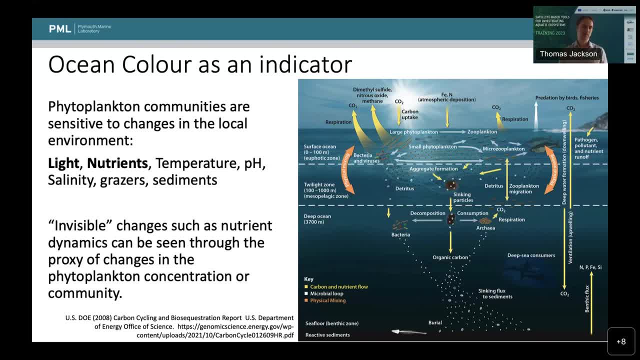 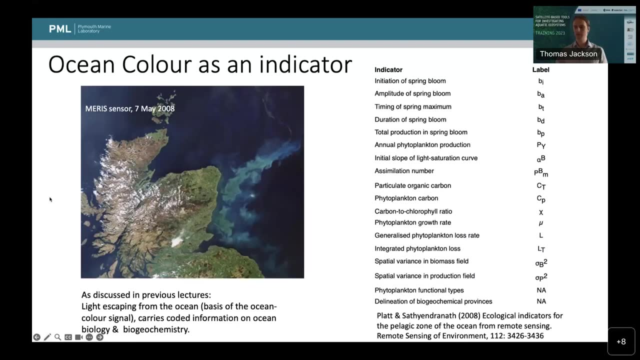 So they can be used as a proxy, And we've talked about proxies in previous lectures. So in that sense the phytoplankton themselves can be an indicator of other change, And there'll be more in the later lectures on phytoplankton production and the carbon cycle. 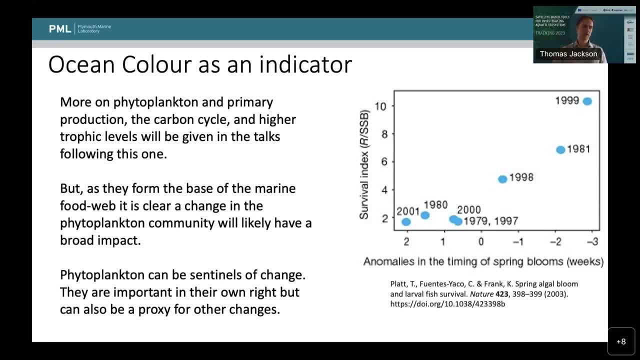 and how that all links into the hydrophic levels. So I'm not going to go too much into the detail on that now. But it's also worth noting that, because they have this, this foundational role in the food web, that any changes we see in the phytoplankton dynamics 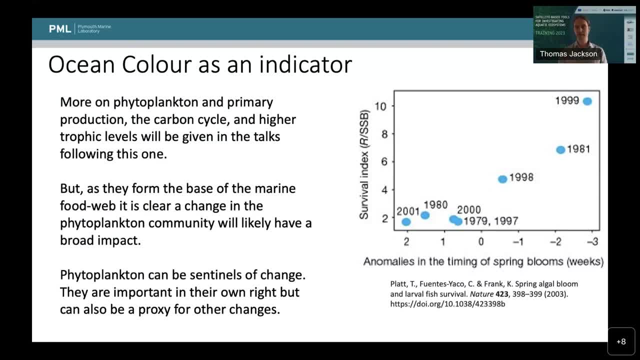 so, whether it's in their abundance, or even which type of phytoplankton are growing, it can have a significant impact on the rest of the marine ecosystem. So sometimes it's useful to think about phytoplankton as these sentinels of change. 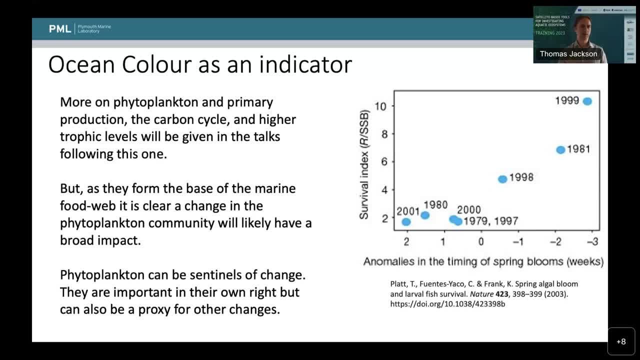 And so they are responding to things that we might otherwise not be able to see. But also they're important And when they change we might see knock-on effects later at other levels within the marine ecosystem, And there's just a nice. so this plot on the right is from a study in 2003 by Trevor Platt and colleagues looking at the spring bloom in the North Atlantic. 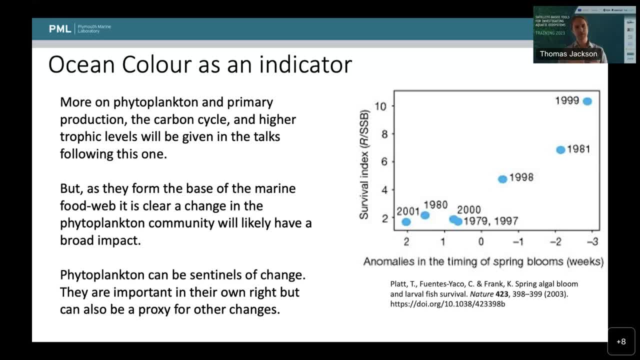 and seeing when that bloom is shifted in time, so early or late. what's the impact on survival index of fish larvae? And so what this means is basically, if the fish larvae aren't lined up in time, they're not there at the same time as the phytoplankton bloom. 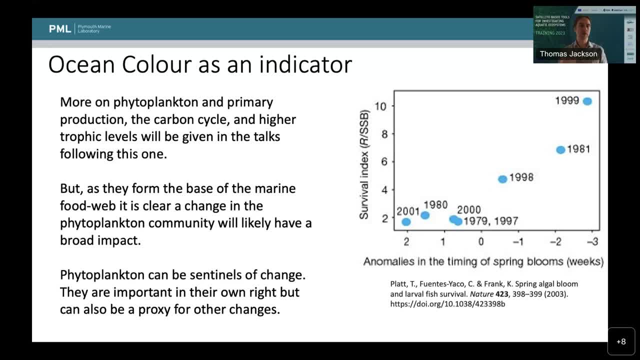 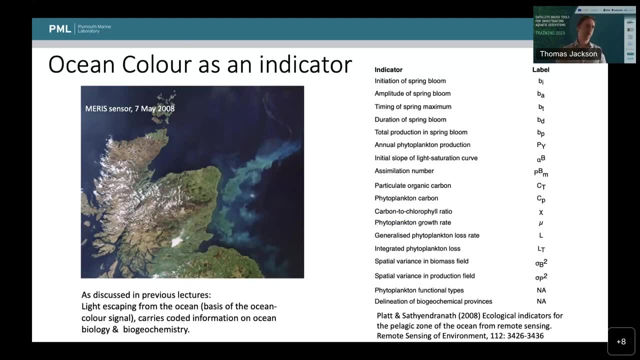 they have a hard time getting enough food to survive. So there we see a knock-on impact from changes in the phytoplankton to the higher levels And I don't think this. the plot here on the chart on the right here has been shown in previous lectures. 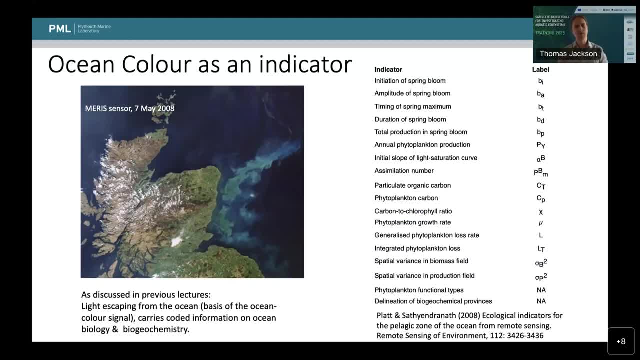 And this is a really nice summary from a paper from Trevor and Shuba, And it was looking at a range of indicators that you can derive from ocean colour. So when we talk about ocean colour in the climate record and things like that, or as an ECV, 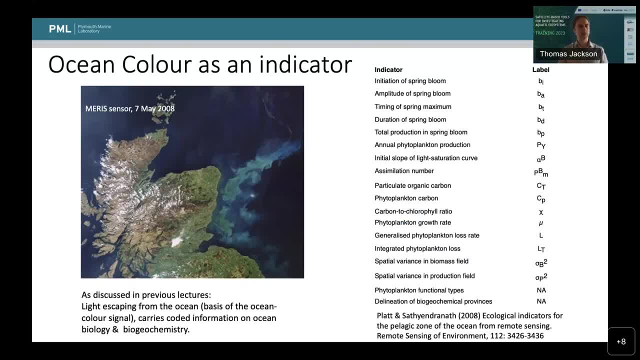 which I'll come on to later. primarily, that's reflectance, and chlorophyll are the variables, But from that we can derive a whole number of indicators. Some of those are phenological, such as the ones at the top about timing of a spring bloom or the amplitude of a bloom. 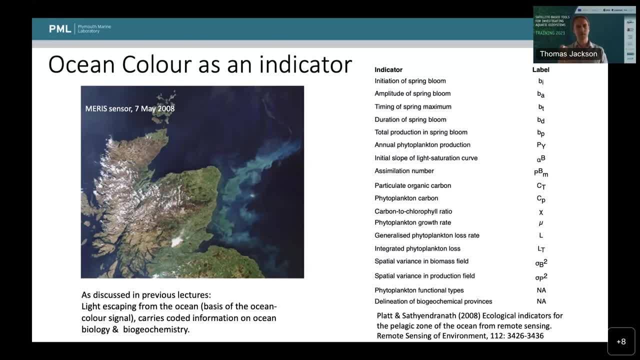 Some of them are more variable based, such as the particular, the particular carbon or the phytoplankton carbon, And some of them are rates, like growth rates or loss rates. So there's a whole number of indicators that we might be interested in when we're trying to look at ecosystem status and function on longer timescales. 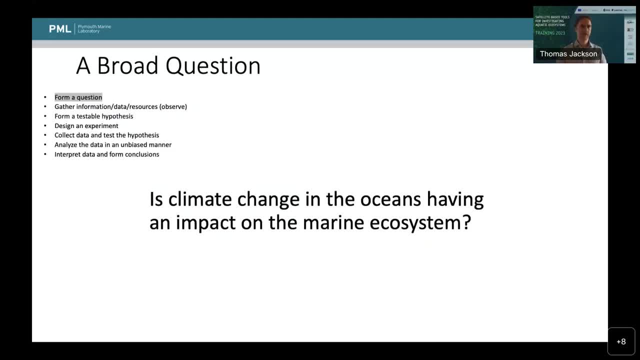 So let's come to a broad question. in our kind of schema of forming questions and testing hypotheses, We can imagine that we might have a question About climate change and the marine ecosystem. So is the climate change that we see going on and how that's changing in the oceans having an impact on the marine ecosystem as a whole? 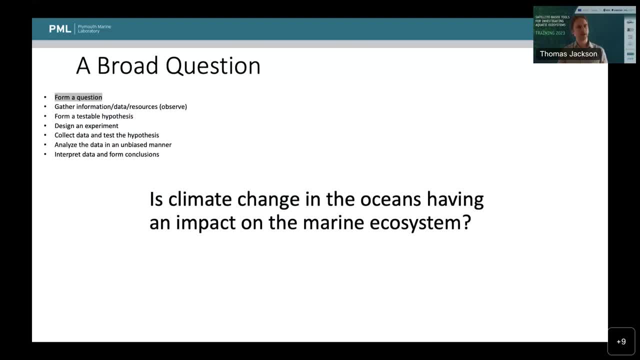 But even here we have to take a hard look at this question and think about what we're actually asking. So what changes do we think of when we say climate change and what's classed as a change in climate? And an important factor on that is: 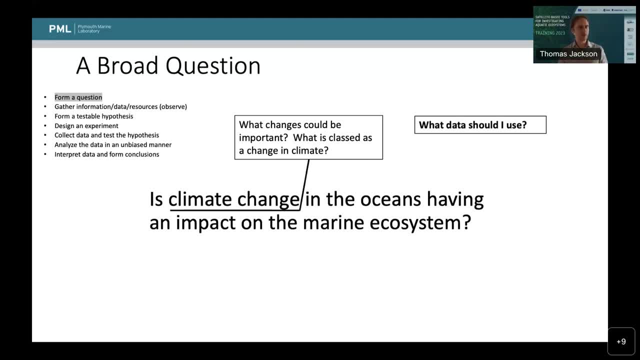 what data should I use when I'm looking at climate change? When we talk about impact, what do we mean having an impact on the marine ecosystem, And are we talking about the whole marine ecosystem or are we talking about a small part of it? 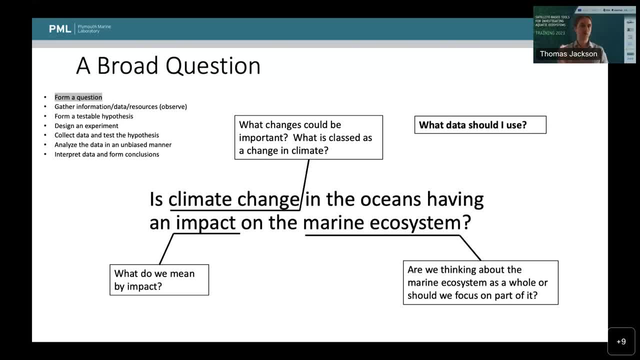 And none of these. if we say we only want to look at part of the marine ecosystem, that doesn't mean that that's an invalid question, but we just have to phrase that question carefully and clearly When we come to forming a testable hypothesis. 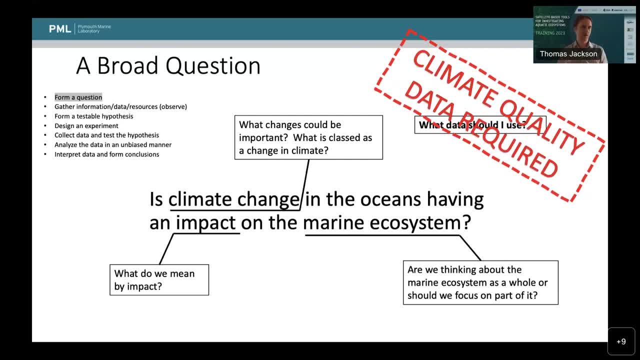 And an important part of this, a huge part of this- is that you have to make sure you use climate quality data whenever you're trying to address questions about climate change and climate change impacts, And I'll get on to what climate quality means, but it's quite stringent. 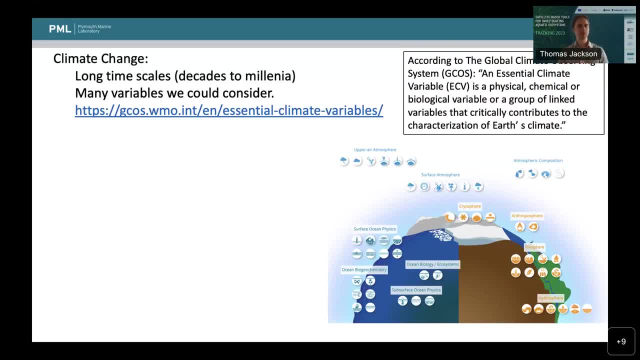 So first let's think of those three points that we were thinking of: Climate, climate change impact and ecosystem monitoring. So climate change is over long timescales, usually from decades to millennia. This is not about whether the level of chlorophyll in the ocean is higher today than it was yesterday. 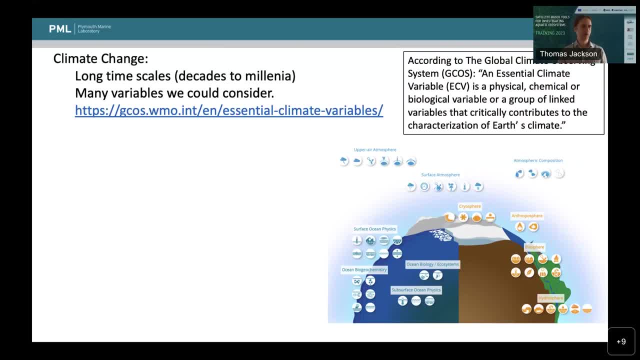 This is about what's happening to the region that you are looking at over much longer scales. So there's a whole number of variables we might consider when we think about climate change, And there is a group called the Global Climate Observing System, summarized as GCOS. 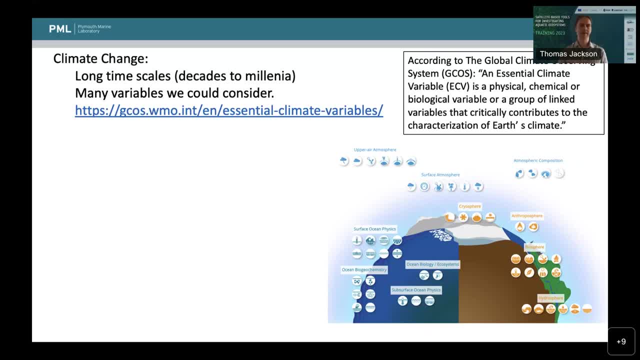 which have defined an essential climate variable as a physical, chemical or biological variable or group of linked variables that contributes to the characterization of the Earth's climate, And they have got a whole list, a whole number of different ECVs. So these essential climate variables that they have separated by, basically, atmosphere. 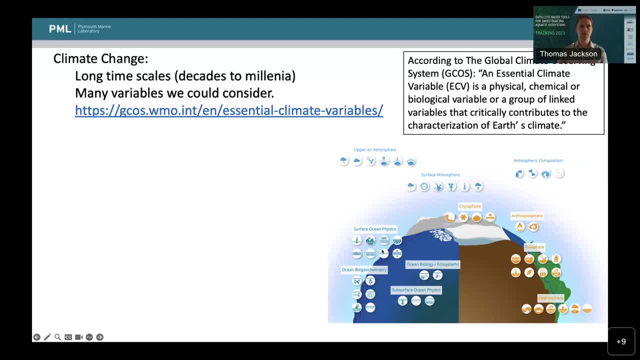 components, land components, water or ocean components. Now I'm not going to go into a huge amount of detail on all of these, but just know that whenever I talk about requirements or quality or I show you the level of detail that's required for an ocean color ECV. 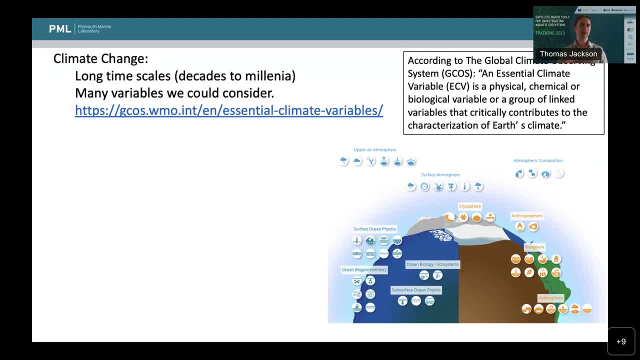 the same is true of all of these, And this is why, when I say when you're thinking about trying to look at climate studies, you have to make sure you're using climate quality data, And that could be temperature of the ocean, It could be temperature of the land. 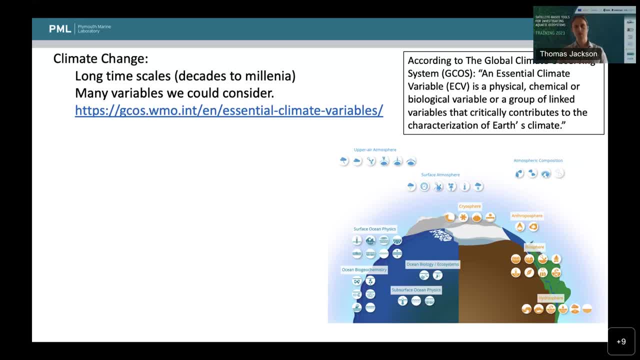 It could be properties of sea ice or all sorts of things, But you want to make sure you're using climate quality data sets. So impact: When we talk about impact, normally we're talking about a change that is detected with a given level of confidence. 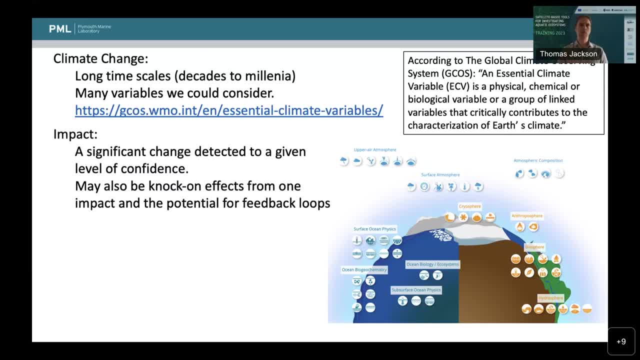 So if we see a change and we can say we are 95% confident that this change is not just an aberration of noise or anomalies, you know, this is a significant change, This is a significant trend or shift And also, when we say, impact, 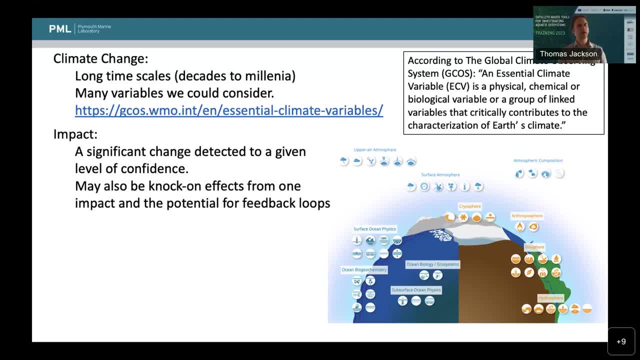 it might be that you have one primary impact, but you could also have knock on effects and feedback loops, So we have to think about those when we talk about the climate system And the marine ecosystem. So rather than considering the entire ecosystem at the minute, 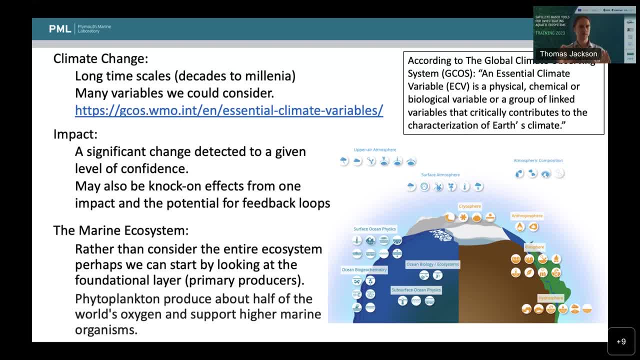 just for this talk, I'm going to focus with ocean color down onto the primary producers, So the phytoplankton, which are a foundational layer And, as I said, because they produced about half of the world's oxygen and support all of the higher marine ecosystems. 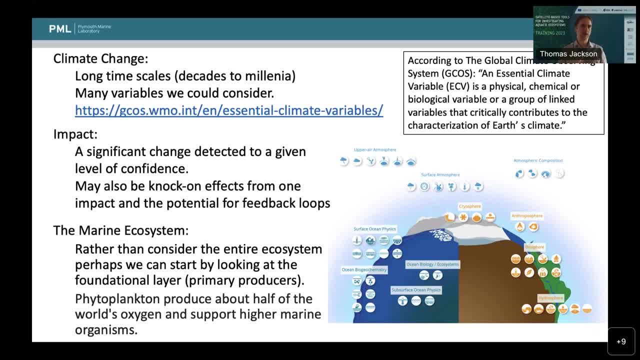 it's actually a very important layer to look at. So if we see changes in that component of the ecosystem, we would expect to see changes elsewhere. So just to show on the diagram, if we zoom in onto the ocean section you can see ocean color is down here. 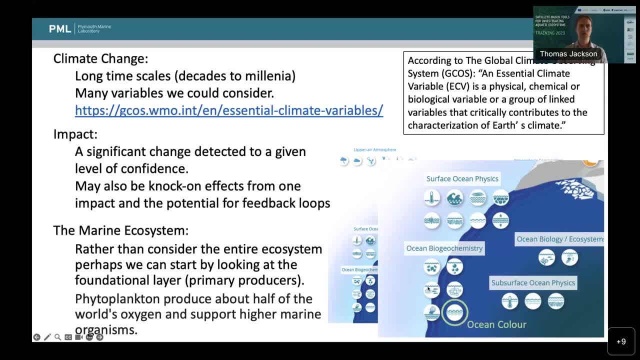 highlighted among the group of ocean biogeochemistry. It's also worth noting that ocean color is the only ECV here which actually allows you to look within the ocean biogeochemistry section. that allows you to look at what's going on biologically. 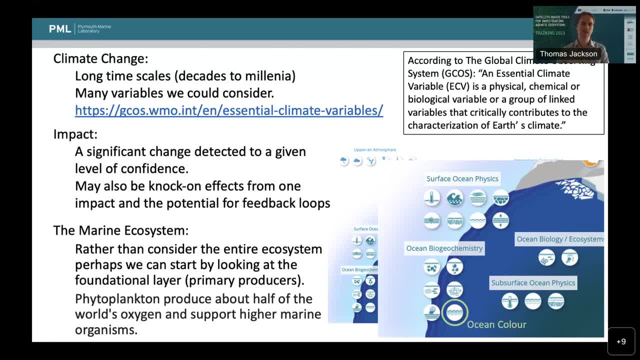 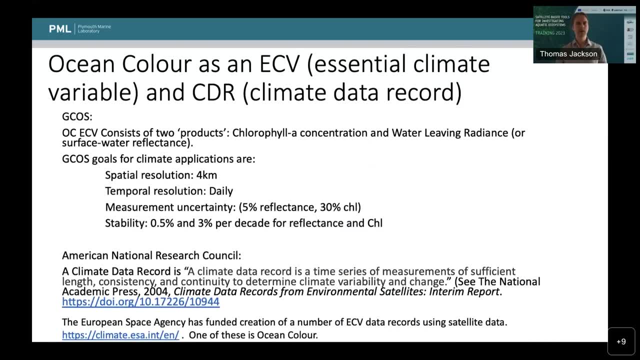 The rest of them are often related to inorganic or chemical processes. So ocean color is an ECV or CDR. So the other term you might hear when we talk about climate records is climate data record. So ECV is the terminology used by GCOS and ESA. 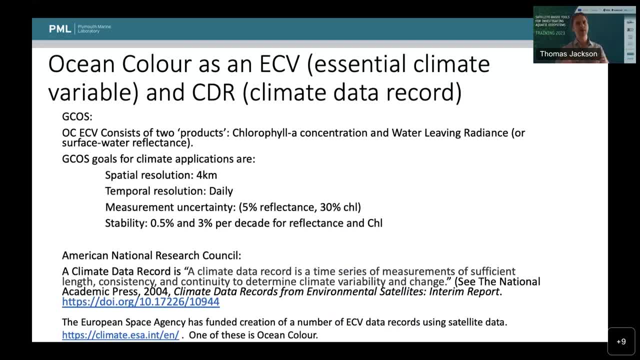 And so that's the essential climate variable, And GCOS defined a set of requirements after discussions with the community around what would actually be needed from ocean color for climate studies, And they have these requirements set out for all of those ECVs that I just showed. 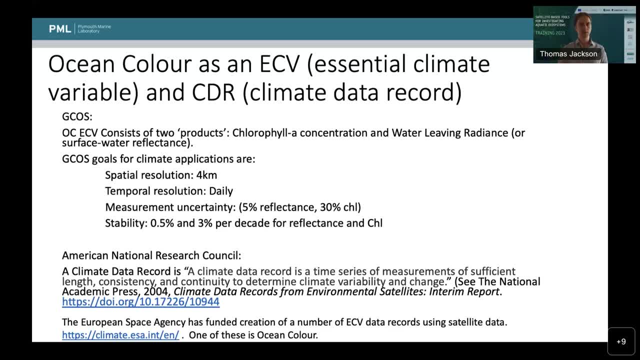 In that diagram, And so if you're interested in a different variable you can go look up what the community requirements for that were. But for ocean color we have a spatial resolution requirement of at least four kilometers or better. Temporal resolution should be daily. 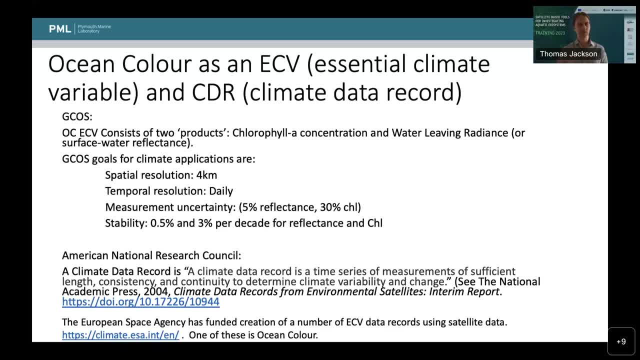 We can then create composites, say a weekly or monthly, but fundamentally we need daily resolution. There is a requirement on measurement uncertainty. So that is 5% for the reflectance product and 30% for the chlorophyll products. 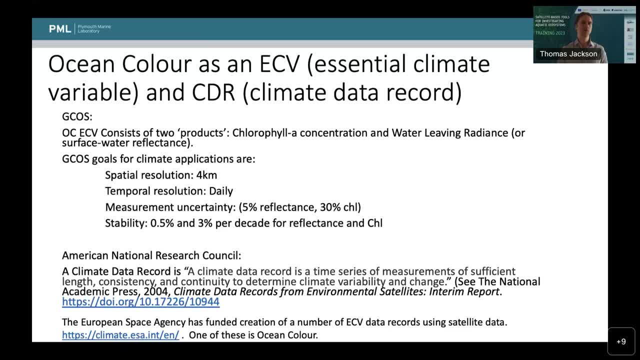 And the requirement on stability, So long term. basically, what that means is that the processing system that you're using to generate the variables is not introducing any trends. So things that you see as a trend, you know are coming from real change and not from an instability in your processing system. 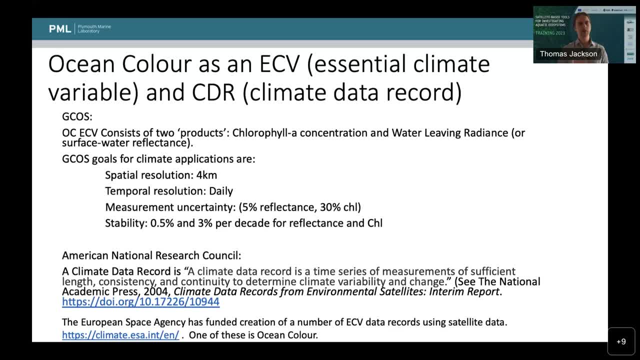 I'll go into that in a minute. So a climate data record. it sounds very similar, So it's a climate data record. It's a time series of measurements of sufficient length, consistency and continuity to determine climate variability and change. So sometimes there is a little distinction between CDR and ECV. 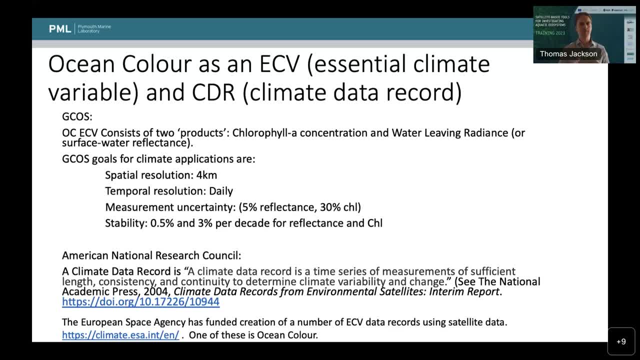 where CDR is the more, let's say, fundamental or primary record. So that might be reflectance, whereas sometimes you might consider chlorophyll as being derived, because we use the reflectance to calculate the chlorophyll And CDR sometimes is thought of as reflectance. 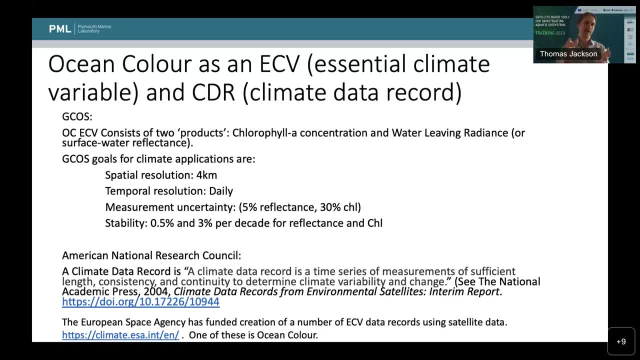 So, anyway, with that in mind, so we have a definition of ECVs and CDRs, and we know that they have to be very high quality. So the European Space Agency, a number of years ago, set up the Climate Change Initiative. 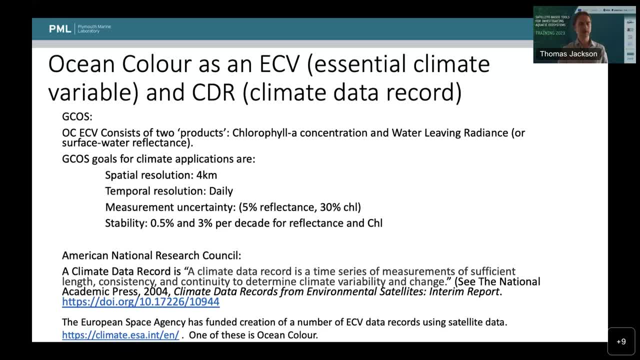 And that was a project- or is a project- it's still ongoing- that was designed to create these ECV records using satellite data, And if you go to the link here, you'll see there's a whole list of ECV data sets. 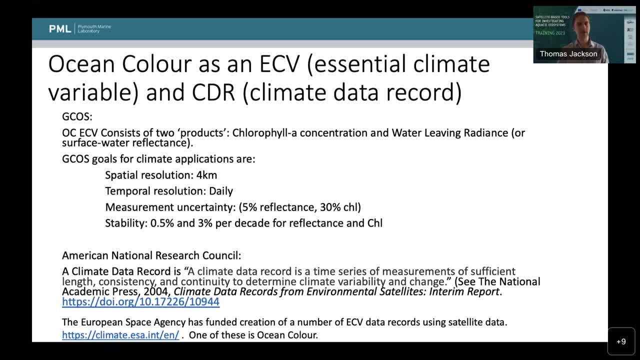 And one of those is ocean colour. So we'll go into that in a bit more detail now. But I just want to stress again these sorts of when you hear things like measurement, uncertainty, stability, consistency, continuity. that's the fundamental properties we have to have in climate quality data. 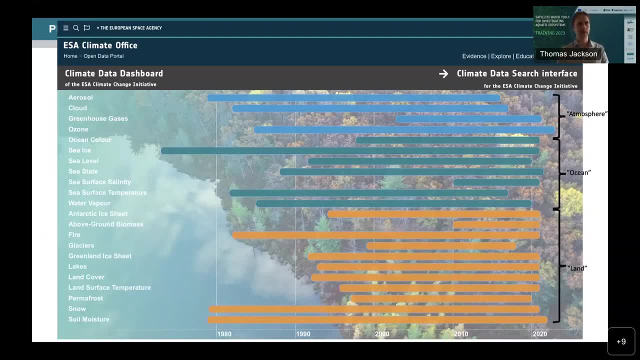 So this is the full set of ECVs from ESA. You can see they span differently, Different amounts of time. That usually depends on which sensors were available to create the record. You can see again they're split by atmosphere, ocean and land groups. 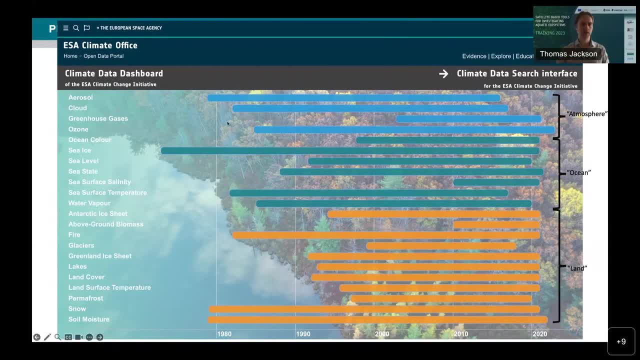 And within the ocean groups, the top one you can see here. this is ocean colour, But if you're interested in any of these, this is a really good place to go and look for data sets And actually it's really nice. 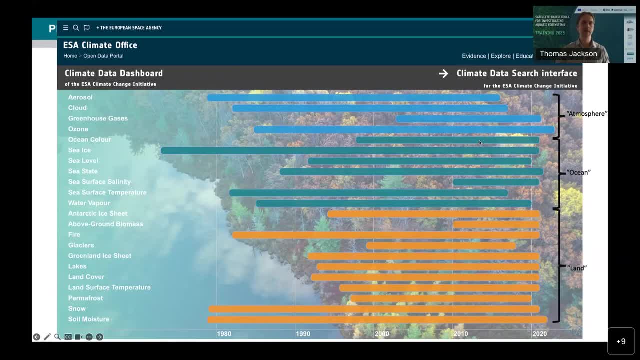 Often you'll find the really interesting science is when you start merging multiple uh data sets into analysis. So if you look at, say, ocean colour in relation to sea ice uh or in relation to um uh, temperature or other things, 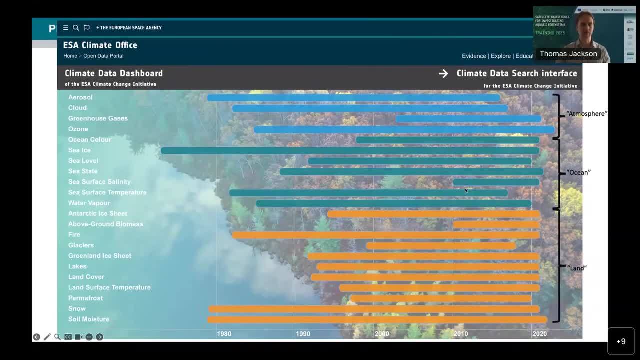 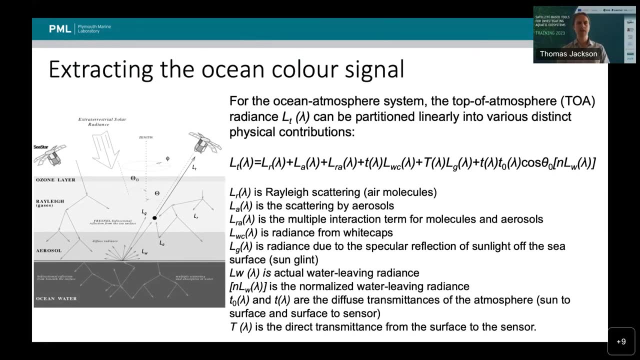 So, um, we'll go into that in a minute. Good, good place to go looking for data. So what goes into generating, uh, an ocean colour, um, CDR, um or an ECV data set? So this plot. 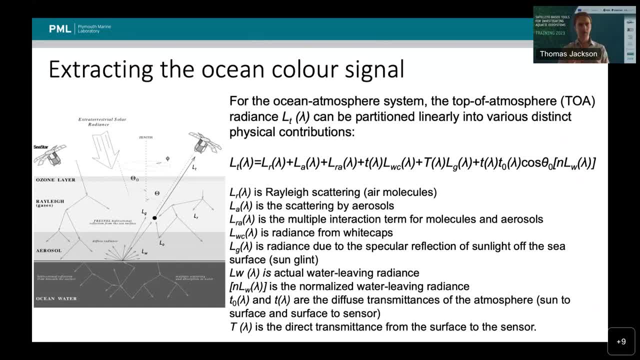 oh, sorry this, uh, I've seen it before when, um, we had the introduction to ocean colour, and I don't want you to have to understand right now every term in here: Um, it's intentionally, um, oh. 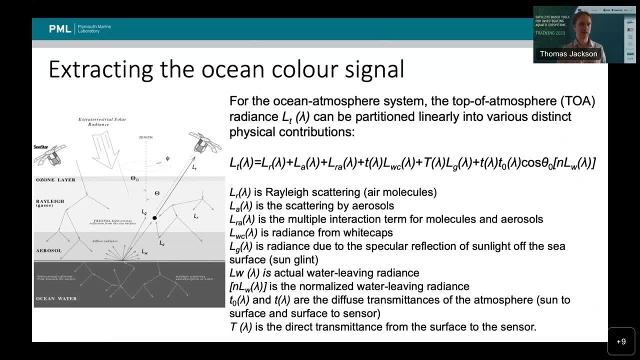 it's a complex equation and that's because the atmospheric correction stage is tough. It's hard to do. We're trying to extract a signal, um, which has a lot of other things in there that we don't want to see, Um. 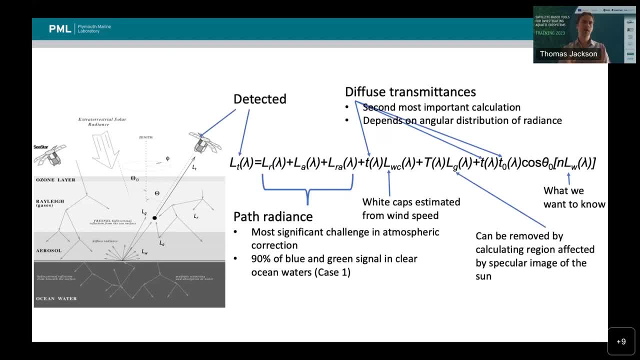 so if I just um skip on here, So on the left we've got LT, which is our top of atmosphere detected radiance uh at the satellite, and right over on the right hand side you can see the LW and that's the bit we actually want from the water. 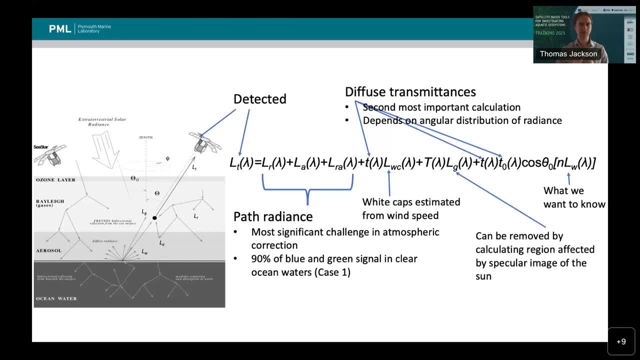 Everything else in the middle is things that we have to remove or correct for during the atmospheric correction process. So we've got path radiances, um, which is about 90% of the signal and needs to be removed. You can think of other things that might contaminate the signal, such as white caps. 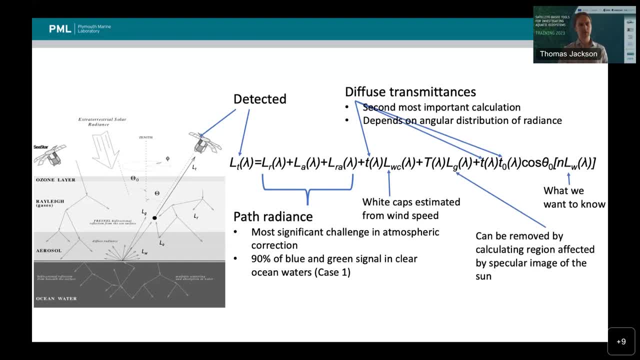 Uh, so when, when the ocean is whipped up by wind, we've got um specular reflection, So glint from the sun, Um, and we've also got to take account of the atmospheric transmittance, Um, so there's. 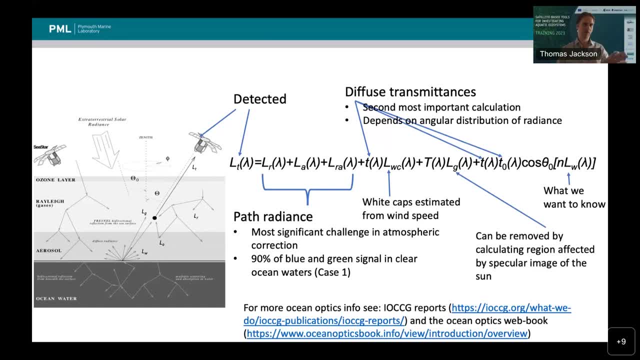 if you to dig into this, we could. I obviously I'm happy to answer questions, but if you want to do more independent reading, um, I would recommend going and having a look at the ICCG reports. um, for all the fundamentals of ocean color. 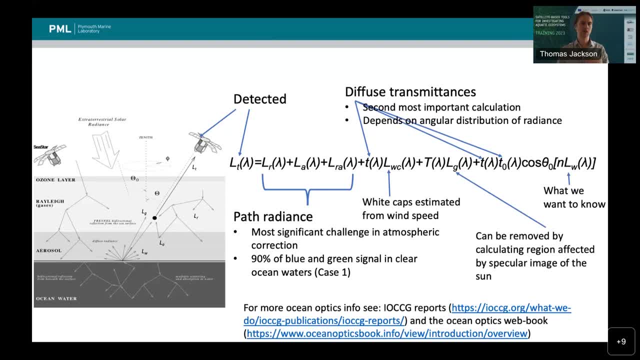 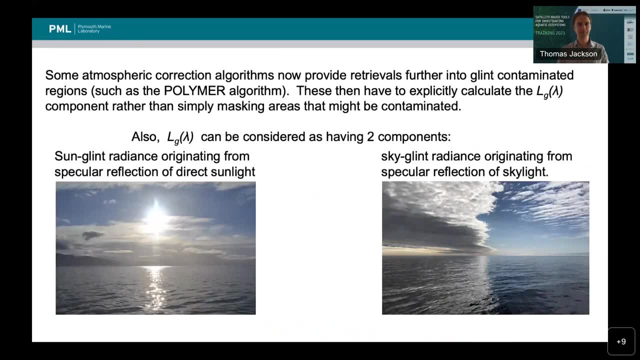 Um, the ocean optics book um has a lot of useful information on um solving radiative transfer equations and things like that, So really good resources there. Um, this is just what I wanted to highlight, um, because it's a really nice. 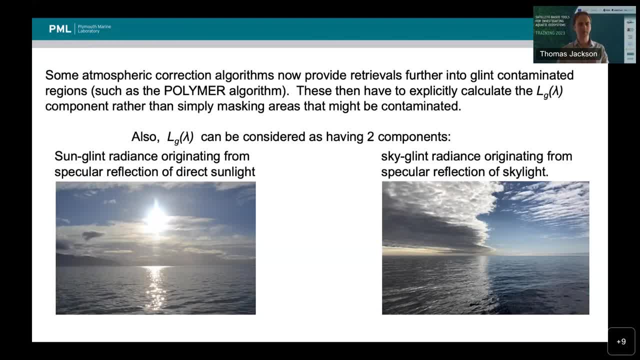 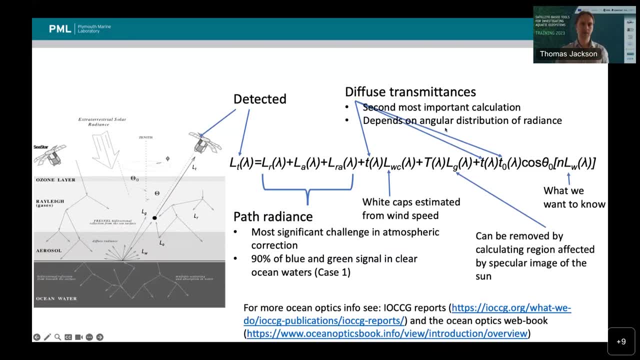 um example of of what we mean by um corrections. So, uh, when we talk about the LG term, so here in the middle, um, you can see, uh, this specular reflection, LG, um, and this is a problem for. 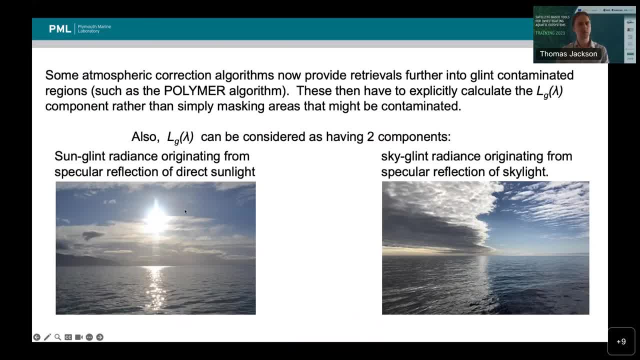 uh satellites because it's extremely bright. Um, it used to be that we would just mask out, uh any area that, from the viewing geometry, we thought would be contaminated by glint. Um, but actually, more recently, uh the. 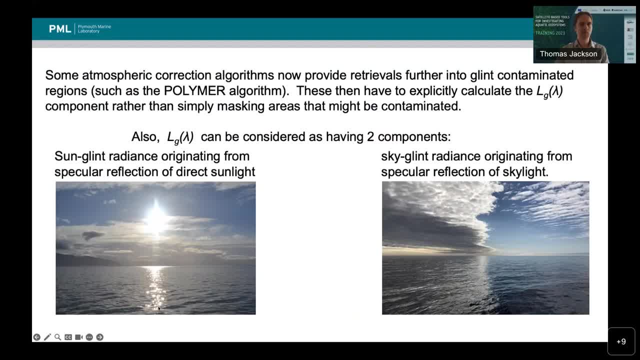 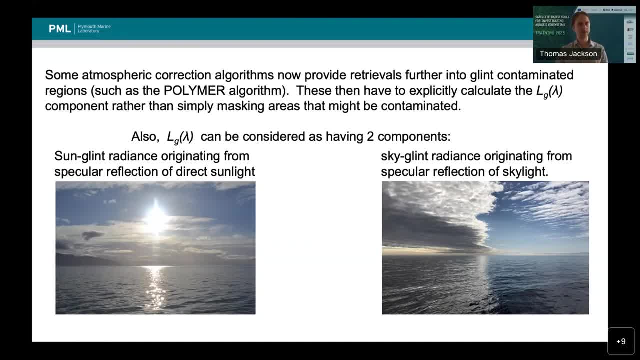 and allowed us to push into that glint region And they can actually calculate and resolve that glint component and remove it properly. Another uh component to the surface reflectance that would be could be interpreted incorrectly is: if you look at the image on the right, 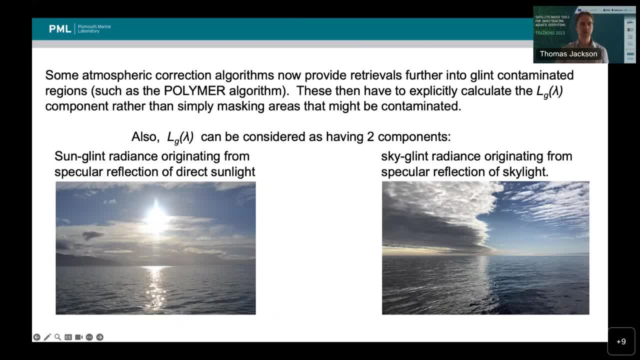 if you ignore the sky, you might think that there is a change in the ocean properties between the left and right side of the image. the left side of the image the ocean looks gray, in the right side gray and the right side the image looks blue. but actually this is not a change in the properties. 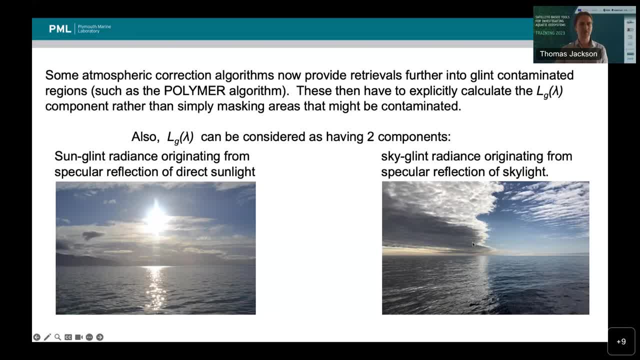 of the water. this is the reflection of the skylight, and so, again, this is a component that we would be in error if we tried to attribute that signal to in-water properties. so, again, this is just me highlighting some of the difficulties that we have to make sure we've accounted for. 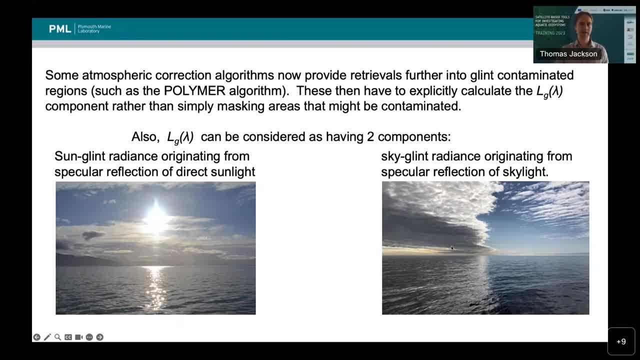 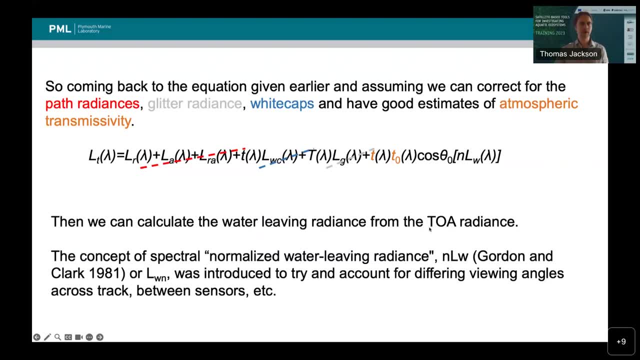 properly when we're looking at high quality data sets. so back to that equation. if we assume that our processing works and we've managed to correct the path radiances- the glitter or glint radiance, the white caps- and we understand what's going on with the atmospheric transmissibility, 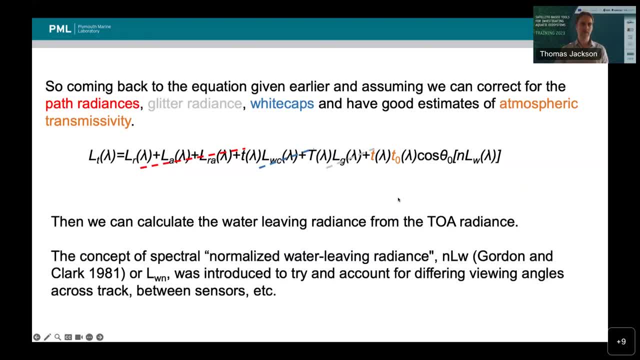 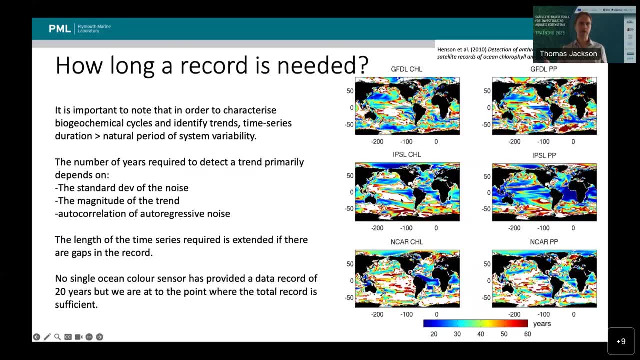 then we can calculate the water leaving reflectance, and that's what then constitutes the ecp, or the ocean color record. so we have this record of data that we've processed, but how long a record do we need? how big does the time series have to be for us to detect climate change? 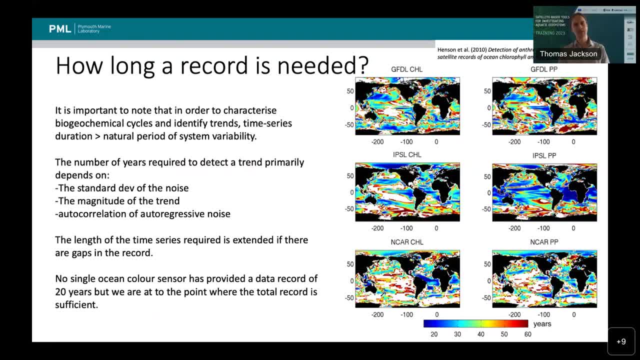 and there was some nice work done by stephanie henson and others, and they actually used a model or a series of models to try and determine the time scale. you would need to have constant observations in order to detect a climate change signal. now, fundamentally, you can think: 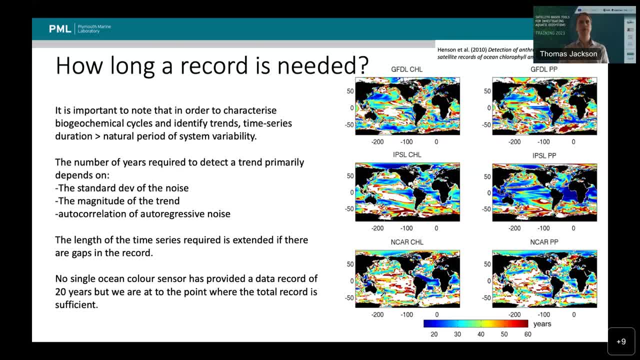 that it's obvious that if you have oscillations on the period of a year, you definitely need more than a year's worth of data to be able to detect any significant change in the water. you can change if you have oscillations on a period of 10 years or eight years, like the 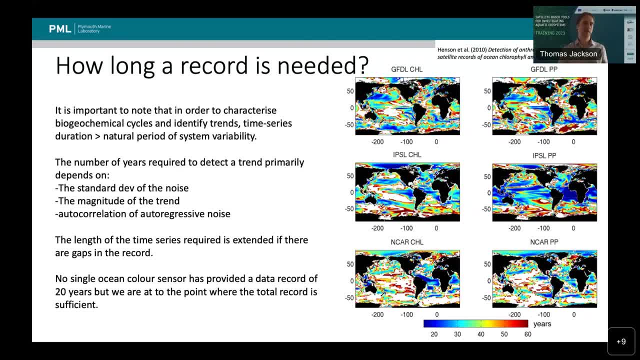 el nino cycle. you need a time series longer than that to be able to detect longer term shifts beyond that natural variability. so fundamentally for any time series analysis the duration has to be longer than the natural period of system variability. if we dig into a bit more detail the properties that really determine that, 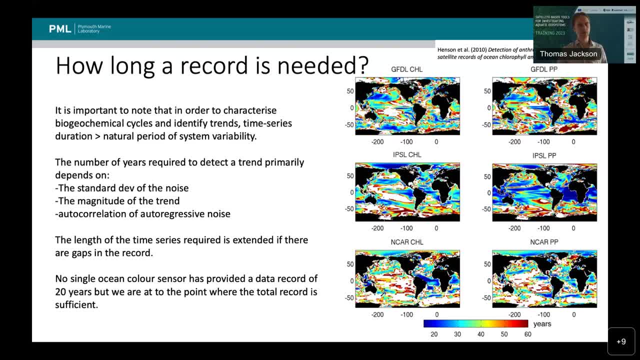 is required. so there's the standard deviation of the noise, so the noisier the signal and the longer the the time series we need. there's the magnitude of the trend, so if you have a very strong trend you don't need as long a time series to detect that trend. and there's also 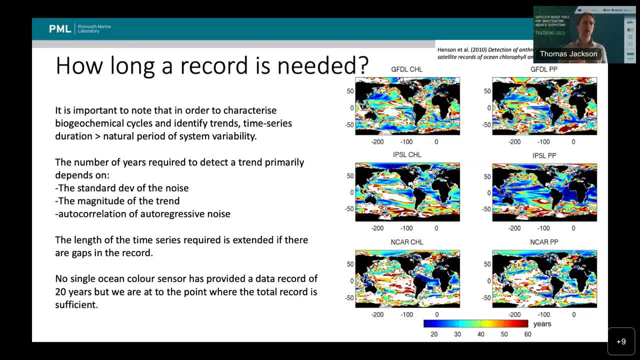 autocorrelation of the noise. so autocorrelation is where your time series has a correlation with a later time step, and so you might imagine if you were taking measurements of a child's height through time or something like that. obviously that's always going to be increasing. 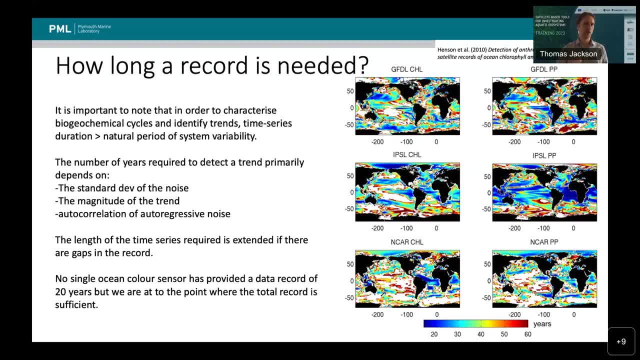 because we know that from time step one to time step two it can only go one way. so there's an autocorrelation there. so by accounting for those autocorrelations or having to account for the autocorrelations, will also change the length of time series required. the last point to consider: 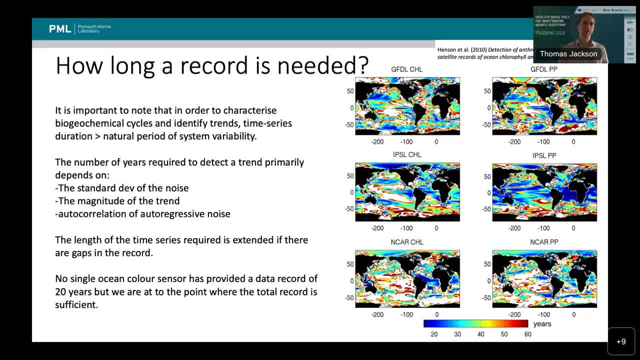 it's actually very important is gaps in the record. so if you have a time series of, say, 10 years, but you measured five years and then you have a gap of a year and then you get four years of data, that is not as useful as having nine years of continuous data with a gap at the end. 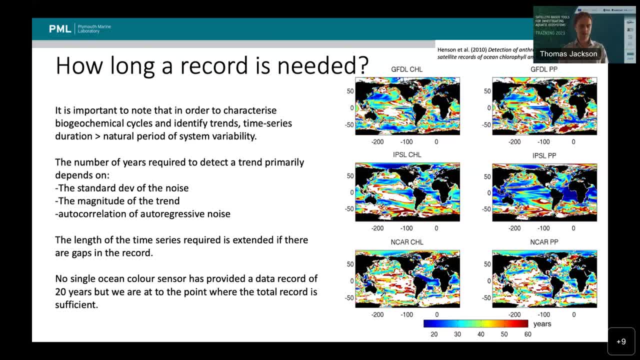 the gap in the middle of the record detaches or breaks the continuity of that record and means you need a longer time series to be able to state that the trend is real and that you know it beyond a certain level of confidence. so, looking at the maps on the right, 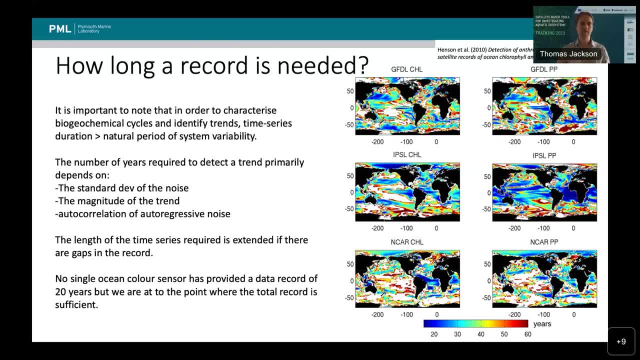 the two columns. so one is chlorophyll and one's primary production. we don't really need to make a distinction between those at the minute. and then the three rows are just different model types. so there was a number of different models used in the exercise, and the different models showed slightly. 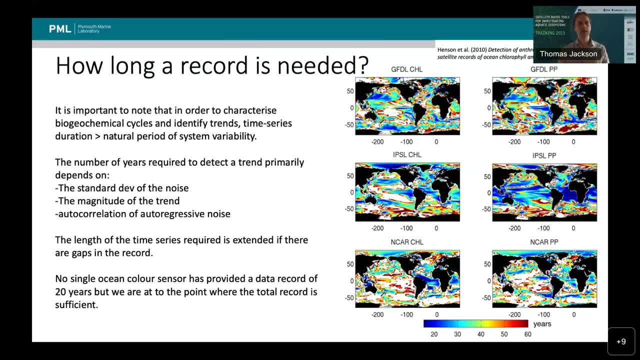 different patterns, but we can see overall there is a variance between around 20 years of data and 60 years of data, which make up a system. look at the record and how long it actually should be, And there isn't a sensor available that provides that length of record on its own. 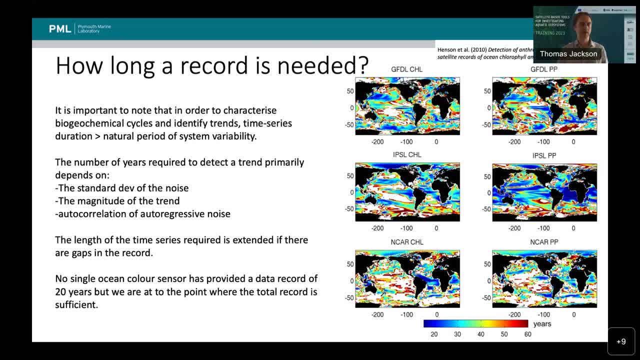 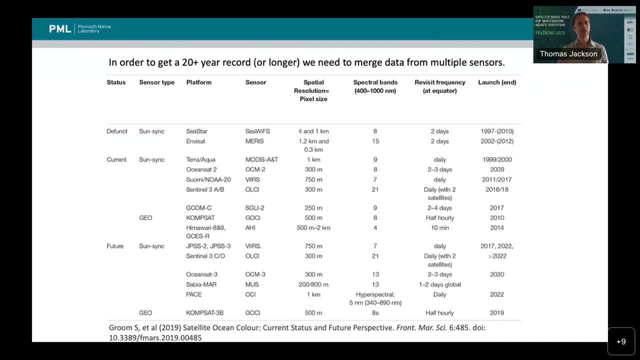 They're just. we haven't had a satellite providing good data for 20 years, So what we need to do is merge sensors. So here's a list of ocean color sensors, And some of them are no longer running, such as SeaWiFS and MERIS. 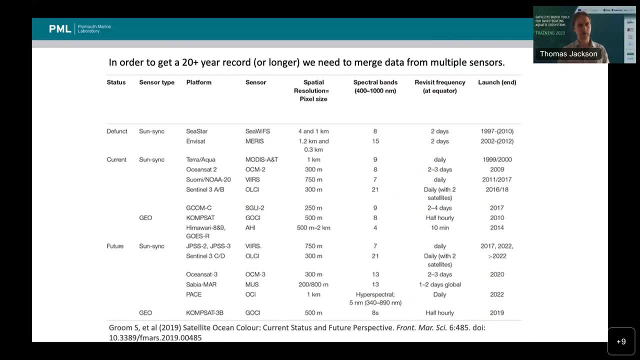 And also, I mean I would consider MODIS now not really operational. It's a dying sensor. So current sensors on here we've got Sentinels 3A and 3B And then into the future, you know, we would expect to see PACE and Sentinels 3C and 3D. 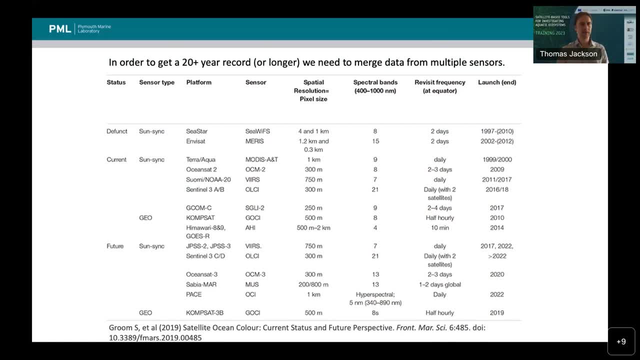 But hopefully you also notice with this list that if we look at the properties of these sensors, so whether it's the spectral bands, whether it's the resolution, spatial resolution also- those spectral bands have different sensitivities or different spectral resolutions. All of that changes from sensor to sensor. 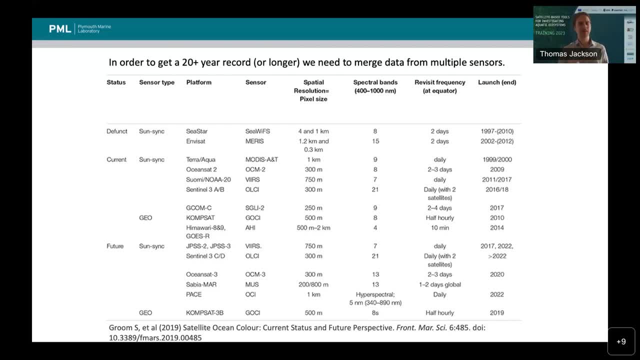 And on the one hand, that's good because the capabilities of the instruments that are being launched is increasing and improving. But it makes it difficult when we're trying to merge these sensors into a single record, because we don't have the same data coming for the whole 25 years or so that we have so far. 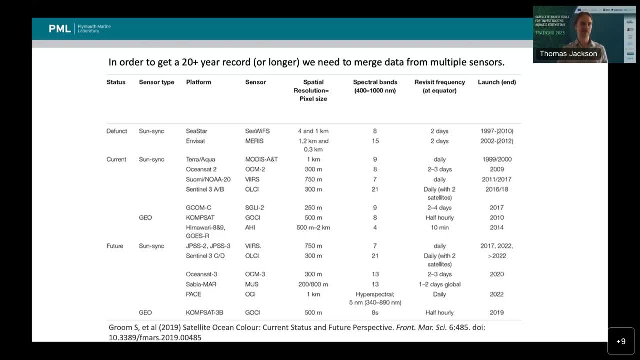 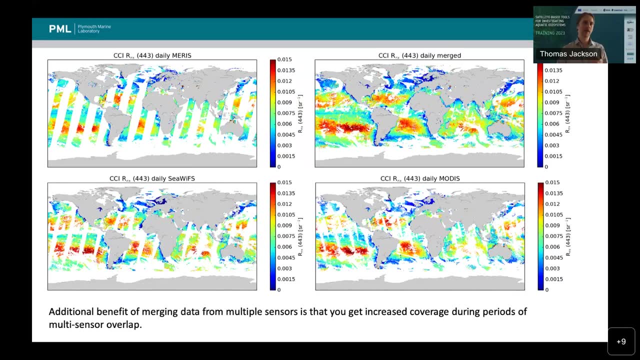 And we have to try and account for that and make sure we don't introduce artifacts where we've got different sensors contributing to the record. So one of the Benefits of merging sensors to get the time series that we need of 20 or 25 years is that we also increase the coverage. 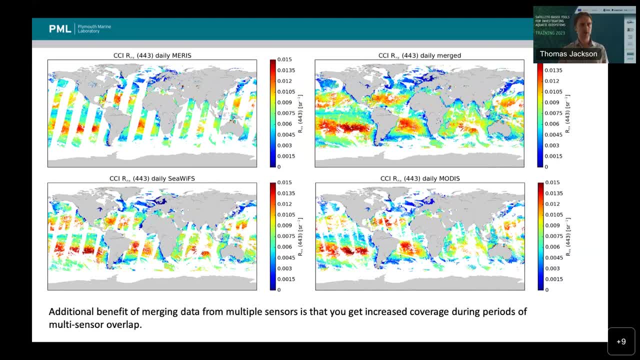 So the top left, bottom left and bottom right panels here show individual daily composites from three different sensors. We've got Maris and CWIS and MODIS, and then in the top right you can see the merge data set. And so not only does our time series grow in length by adding these sensors together into a merge record. 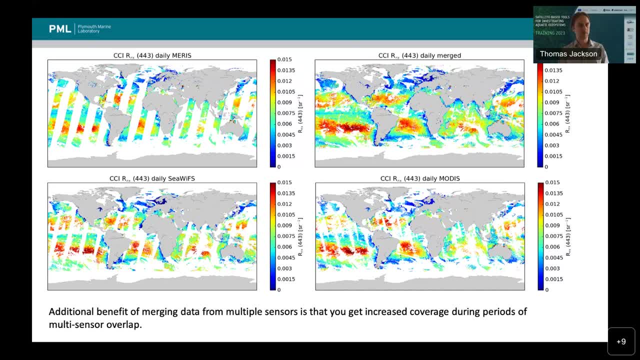 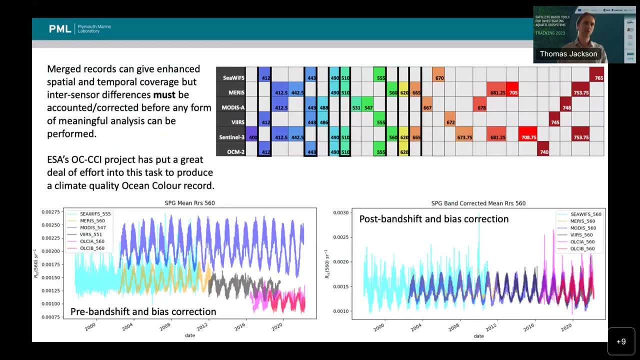 we get much better coverage and that means there's also less gaps in the record. So it's a win win. So we get multiple benefits from from merging the data sets, But we have to be extremely careful. So in the top figure here we've got six different sensors listed and you can see they all have slightly different wavelength sets. 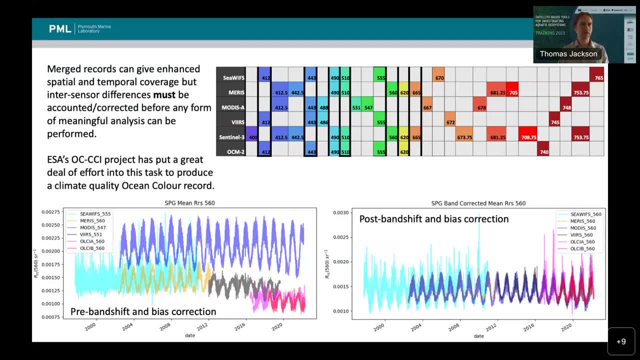 The closest pairing is probably Maris and Sentinel 3, but even there Sentinel 3 has bands that Maris didn't. And to have a consistent record across the entire time series, we basically need the same wavelengths to be measured From the start to the end. So what we do within OCCCI is we have this: 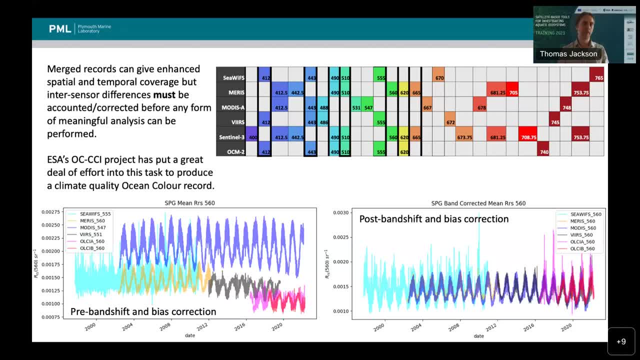 Processing stage that we call band shifting. So we pick a reference sensor and for the latest versions, that has been designated as Maris And And we correct the um data that we have at the native wavelengths of each sensor To uh the wavelengths of the reference sensor. 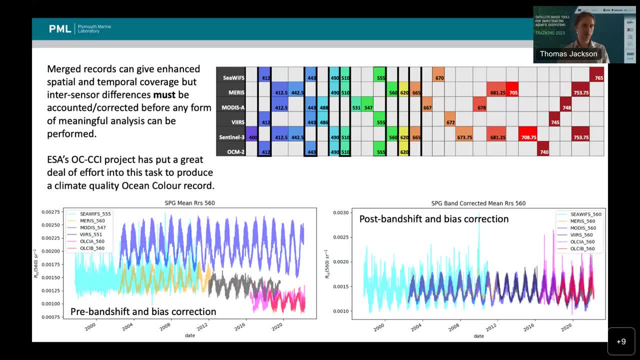 I can go into more details, perhaps in the Q and if people are interested, but basically this involves running a forward model to generate a hyperspectral Um uh signal and then we uh extract from the the wavelengths that we actually want for the references. 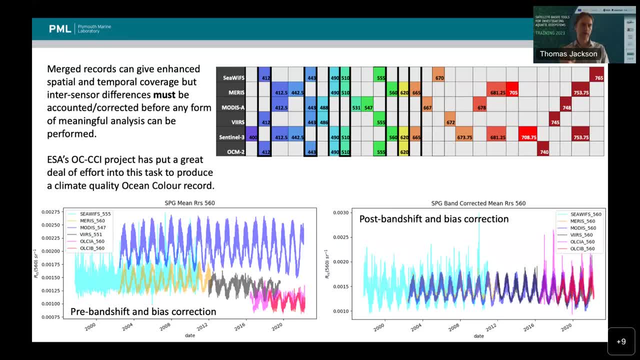 Um, but we also have limits on how how far we're allowed to shift Um, but we also have limits on how how far we're allowed to shift Um, but we also have limits on how how far we're allowed to shift. 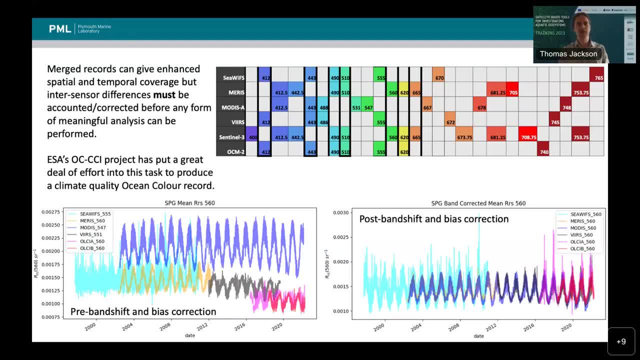 And so we don't want to be trying to shift, say, from 670 nanometers up to 720, like this too big a spectrum jump. So we're only allowed to shift a certain distance spectrum. So that's the band shifting. But even when we band shift, that isn't the whole story. 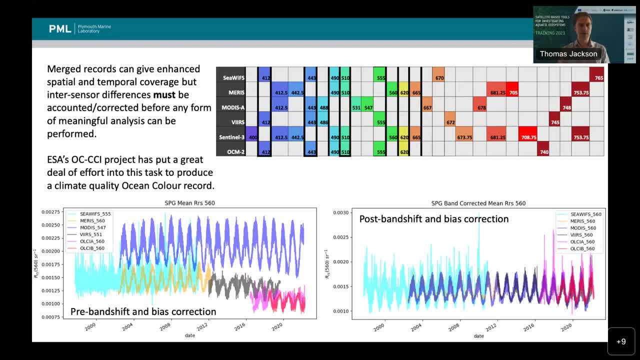 Because even if we consider two different sensors in orbit, even when they have the same wavelengths, those two sensors are not identical and they aren't seeing things in an identical manner. So if you look at the plot in the bottom left, that's an extracted data set for an area in the South Pacific, Gyre. 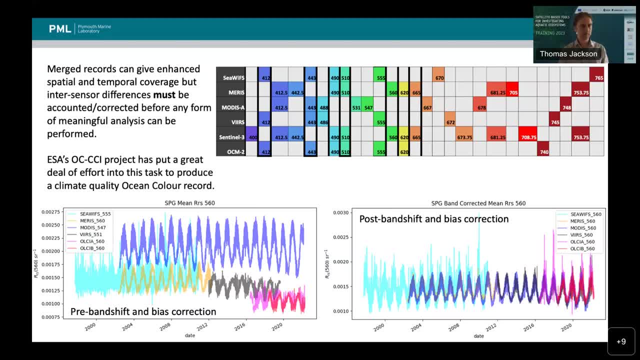 And the South Pacific Gyre is a very stable region of the ocean And so you can see there's a series of sensors on there. We've got SEWIS, MERIS, MODIS, VIRS and the two ULCHIs. 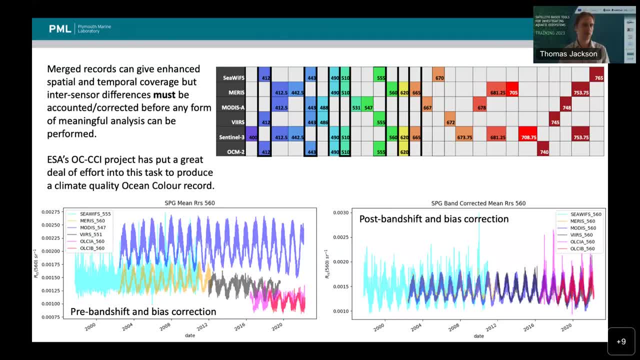 Now you would expect the two ULCHIs to agree relatively well because by design those are supposed to be identical sensors, So you can see the pink and the red overlap pretty closely. But all of the other sensors have significant offsets. And if you imagine taking something like the MODIS record in purple at the top and the ULCHI record in pink at the bottom, 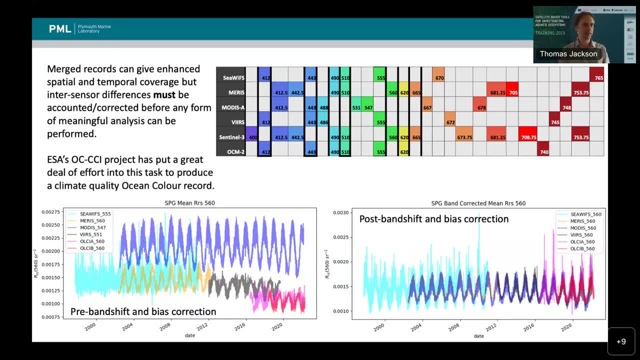 and trying to merge those or average the two together. when you introduce ULCHI, you would see a big step In the record. we don't want that, that's. that's an artefact of the merging process rather than a real representation of a change in the system. 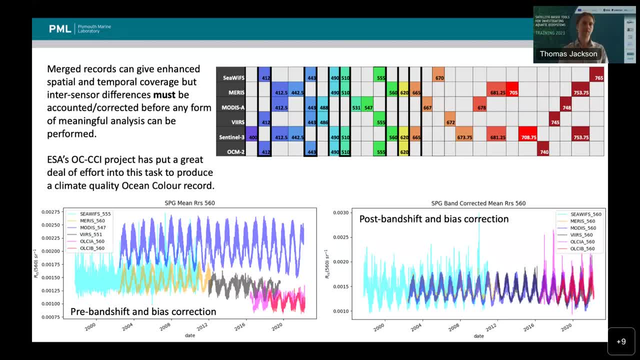 And so we have a what we call bias correction step which accounts for the differences between the different sensors, and that's done for every single pixel on the globe, every day of the year that we have measurements for each sensor. But when we constructed that methodology, we have to do it in a way. 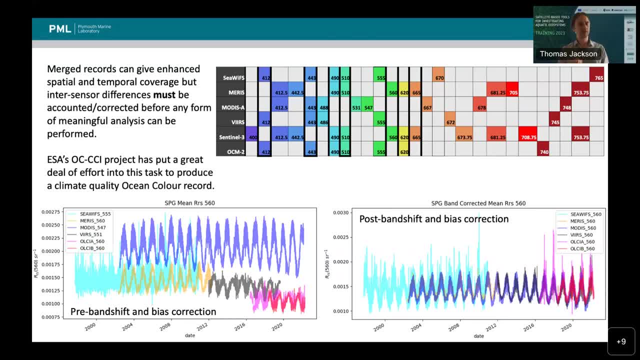 That it cannot introduce trends itself. so we don't want to have a method that might artificially create a downward trend or an upward trend in the record, as it's attempting to correct between the satellites. So what we do is we create, we use the overlap periods between sensors to basically create a daily climatology of the offsets between them, and then we apply that back as a correction. 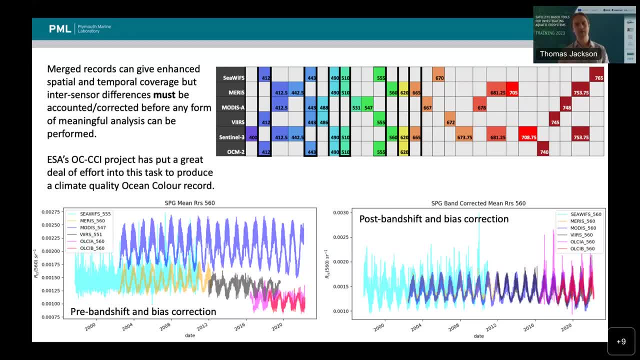 And that gives us the results From the bottom right And you can see that pretty much all of the sensors are agreeing in terms of the magnitude of the reflectance, the seasonal cycle of the reflectance And the. the 1 thing that stands out is we've got a little bit more noise during, or higher range during, the sea, with period, And so obviously that was an older sensor. 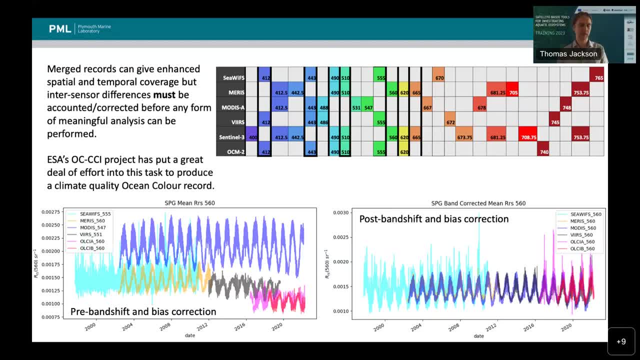 Um, and maybe didn't have the? um quite the sensitivity, uh, that the other sensors have, or the the number of bits available um in its reflective stance. Um, and maybe didn't have the? um quite the sensitivity, uh, that the other sensors have, or the the number of bits available um in its reflective stance. 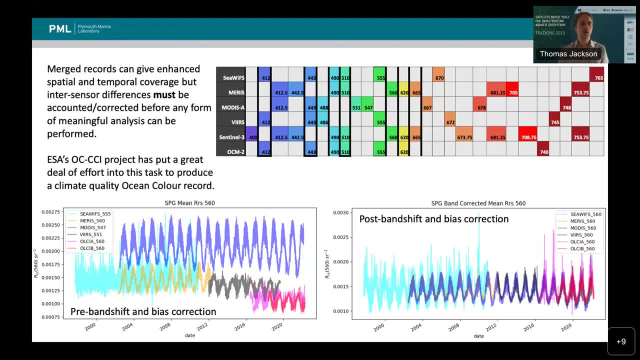 Um, and maybe didn't have the? um quite the sensitivity, uh, that the other sensors have, or the the number of bits available, um in its reflective stance, Um, but uh, yeah, overall we're happy with with that span shifting and bias correction process. uh, that is giving us a good ocean color record. 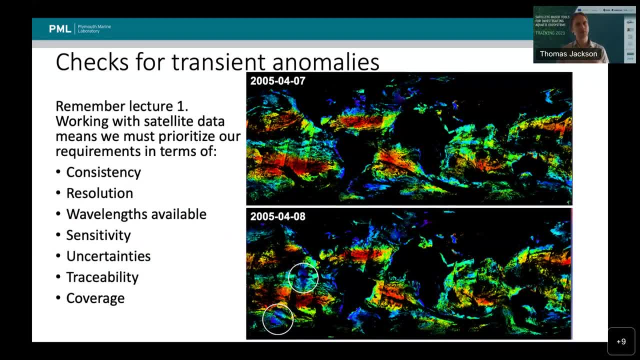 So, as well as systematic anomalies like that, we also have to take account of transient anomalies, and there's a whole number of sources of these uh that might come up, and this is part of the QC and uh quality control and checks um that we've iterated over the years within uh ocean color. 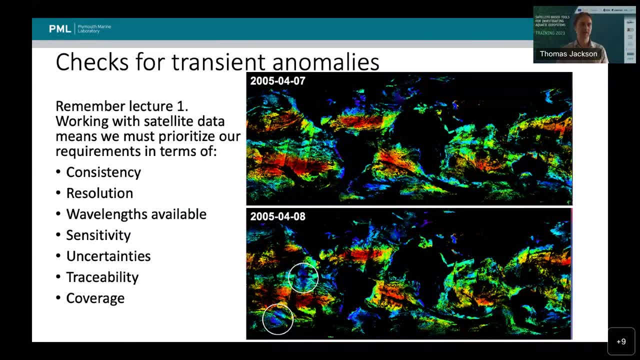 CCI and this is part of the QC and uh quality control and checks um that we've iterated over the years uh within uh ocean color CCI. So if I just uh draw your eye to the circles um in the lower panel here, these images are taken um well, the daily composites taken 1 day apart. 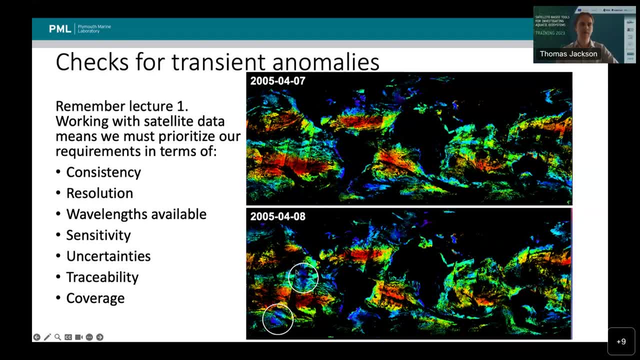 So we have the 7th and the 8th of April, uh, in 2005, and uh, you can see, this is reflectance. Um, you can see the reflectance changes significantly in these 2 areas. 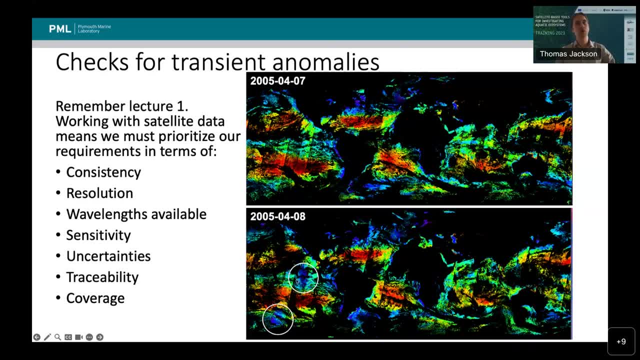 Uh, from day to day and you might imagine from what you know or have learned from this course, uh about, um, the cycles and changes in In ocean color and ocean properties. this is a very big change to happen in 1 day. 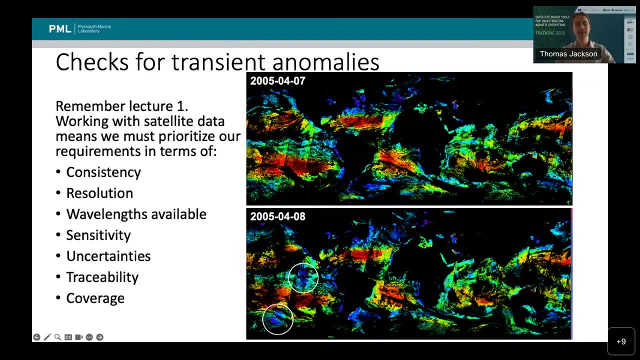 And I haven't put it on here, but if I showed you the next day, uh, they would actually revert back to values like this. So this is: it's flipped just for a day. So if you think for a 2nd, maybe about what might have caused that, um, 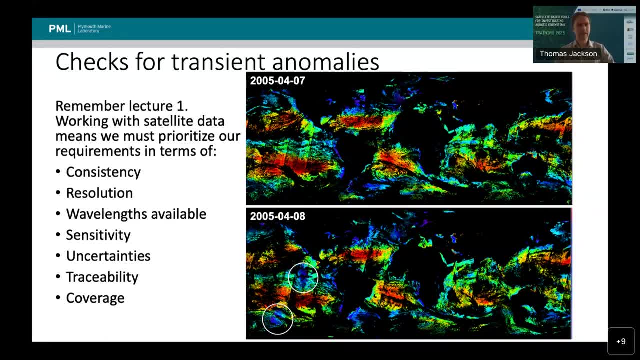 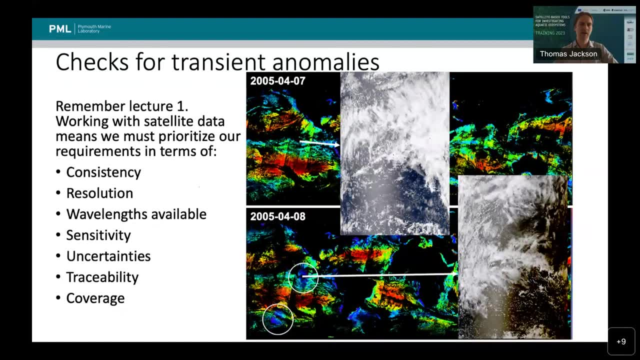 You know there's all sorts of things it might be, but when we dig into it, what we actually find out Is that the image in the top when we go- and sorry, when we go- and look at the true color, Um, looks like this. so it's got blue oceans and some white cloud. 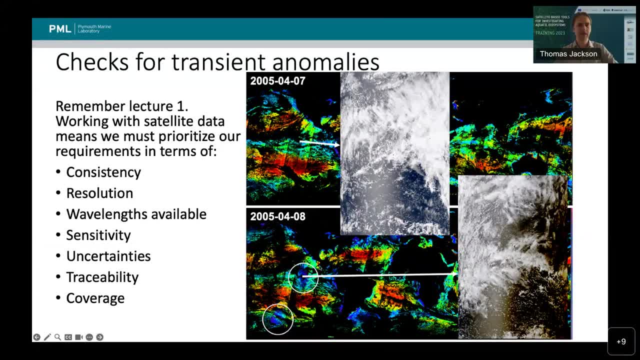 Yeah, that makes sense what we expect. down here. The ocean looks almost black and the clouds have gone kind of brown. And um, this is puzzling. uh, clearly not what we would expect to see in an ocean color image. And um, it turns out this is a solar eclipse. 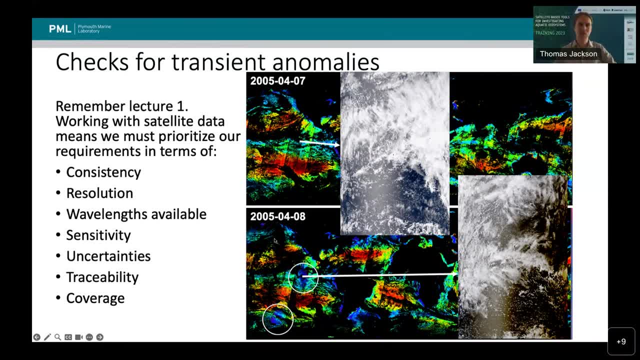 So it just so happened, as the satellite sensor was taking A picture of that part of the ocean, uh, the shadow of the moon was also passing across and this down here, So the moon transited, So as the satellite went over and came around for its next orbit. 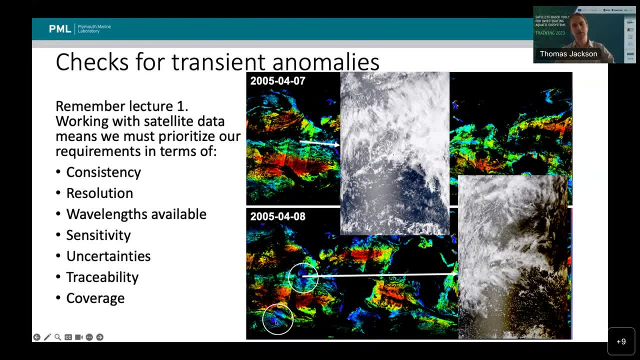 Uh, it picked up the shadow again in a different location, And so this was like a double uh hit uh from a a single solar eclipse, And these are the sorts of things that you also have to be very careful that you have cleaned the record and made sure it's top quality before you're doing uh. climate change studies. 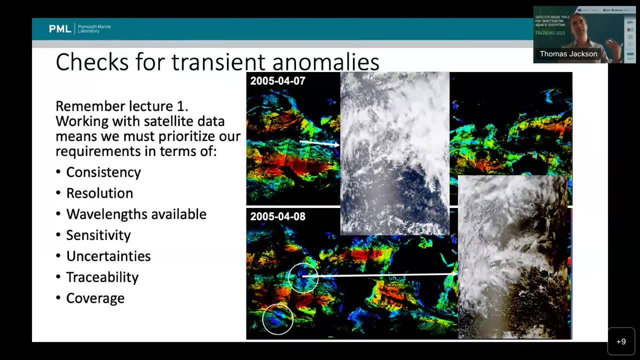 Now, if we go back to the um, the lecture that Lauren gave 1st she gets. she really stressed the point that you can't have everything all the time everywhere. You have to make a choice between whether you want high resolution. 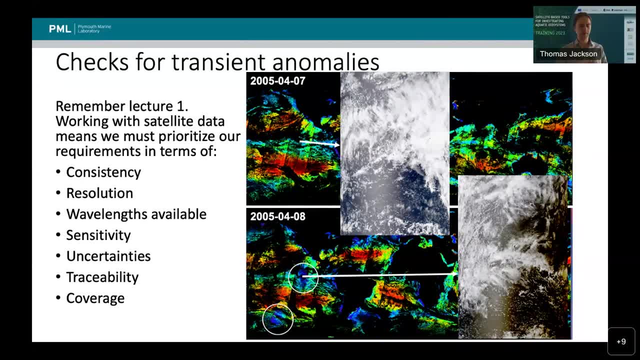 Um, you know, revisit time um spectral resolution, Uh sensitivity, uh signal to noise ratio- all these sorts of things are are are properties that you have to balance. You can't have everything. So, when it comes to the climate record, um. 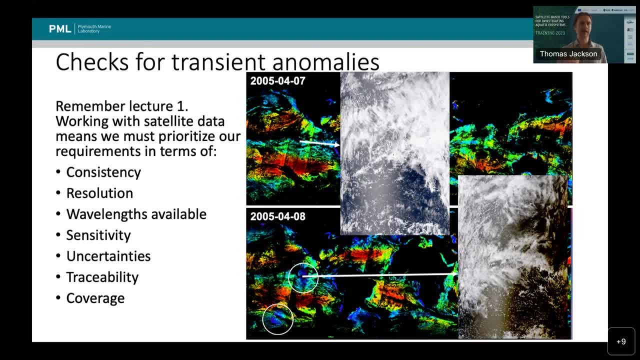 Consistency and traceability and sensitivity. these sorts of things are very important and it means that sometimes we have to push coverage down the list a little. So here is: obviously we would want to mask the Solar eclipse. that's definitely going to be bad data and corrupt. 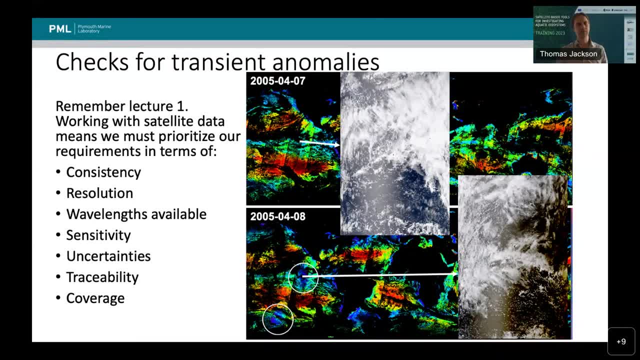 Um the record. there's also steps where We have to make a choice, and it's it's. sometimes it would be nice to have the data, But we have to apply the masks because, um, consistency and quality has to be our primary goal. 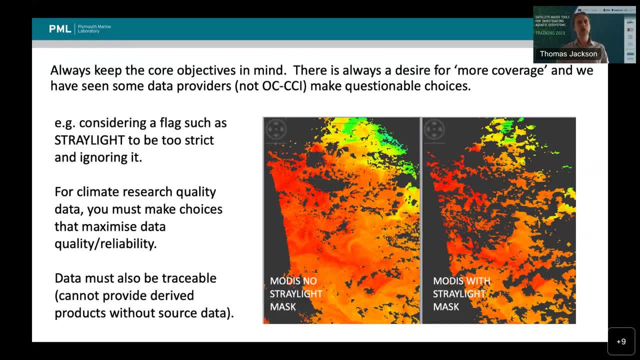 This is an example of just that. So In the left image- uh, you can see- there's much more data than in the right image, And the reason for that is just 1 of the many flags or masks, um, that are applied during the processing has been turned off. 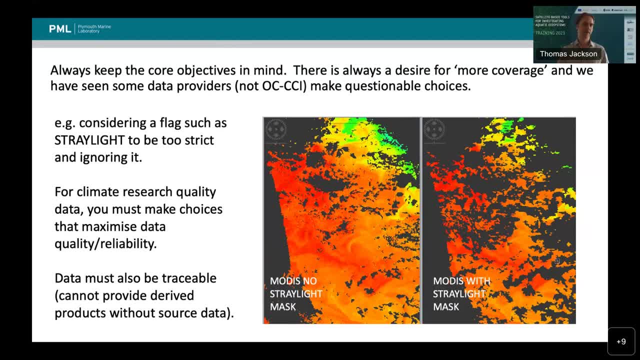 So the difference is that there's no straight light mask and the stray light mask is designed such that around bright targets you can have a problem where That uh bright object, the reflectance from it, is scattered within the atmosphere and contaminates adjacent pixels. 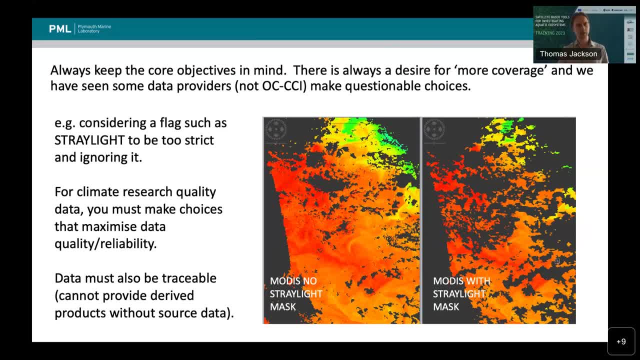 And so basically around things like clouds and and bright objects, there is this Mask in this image. you can see that by removing that mass You actually get a lot more data and it looks reasonable. It seems to follow the same um patterns and shapes. Uh, 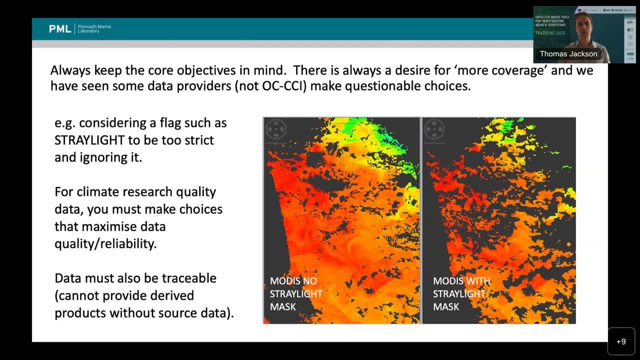 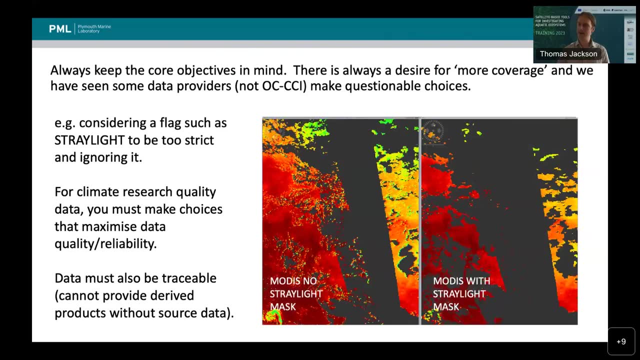 But they look oceanographic, look realistic, um. so you might think, let's turn it off, and we've seen examples of people trying to generate climate quality data with this turned off and it's a problem, um, because you go and process an image somewhere else and this is the difference and you've got a whole bunch of horrible. 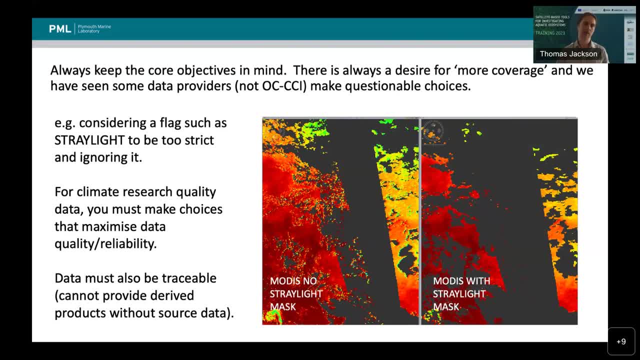 data which really shouldn't be in the climate record. um, all around the clouds, and in some ways you might think of this as being noise, and, but actually, because this is around bright objects, this actually has a slightly systematic component and it will tend to influence things in the same. 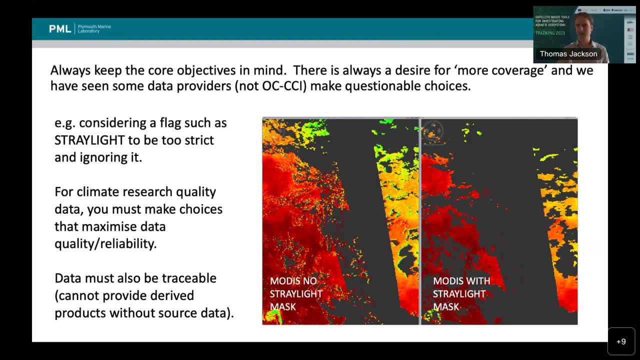 way and but anyway, that's just a thing. so we always have to stress, uh, quality and reliability, um, and and traceability. so, um, we, if we provide chlorophyll, you would expect that you should also see the reflectances to go alongside it, because if the reflectances aren't good enough, 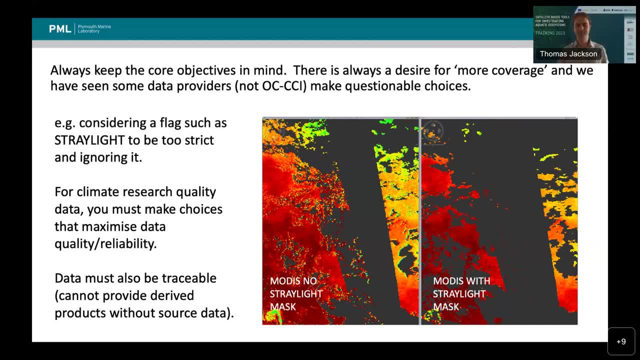 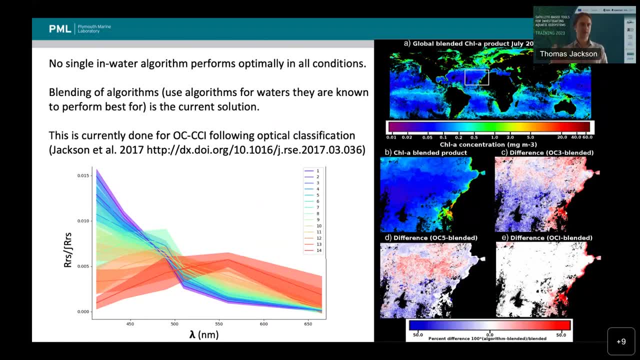 and you don't trust them, you probably shouldn't be derived in chlorophyll from it, um. so once we have a high quality reflectance data set, we have to generate downstream products like chlorophyll, and there's been a whole bunch of questions over the past weeks. 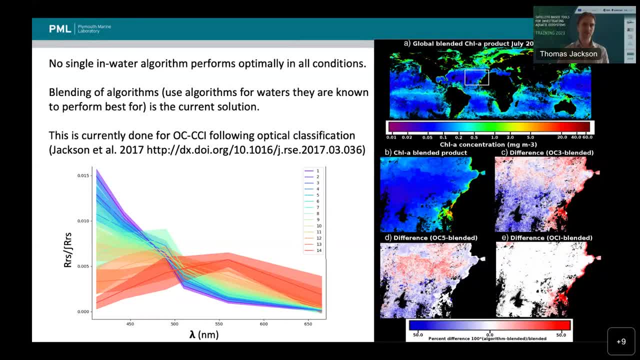 around which algorithms best. which algorithm should i use, and at the global scale? uh, the answer is: there isn't just one, and there is no single algorithm that performs best across all waters. so, um, when we're merging all this data, we're going to have to think about how we're going to 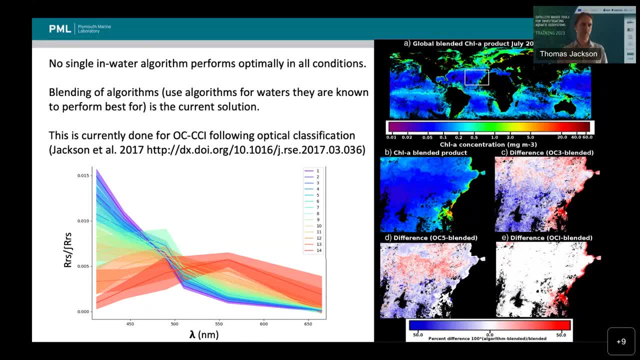 do that and then, when we're doing that, then once we've got all this data together, the approach that we've taken is to use an algorithm blending approach. so the way this works is that we look at the spectral shape of each pixel and we assign it a membership to a number of different spectral. 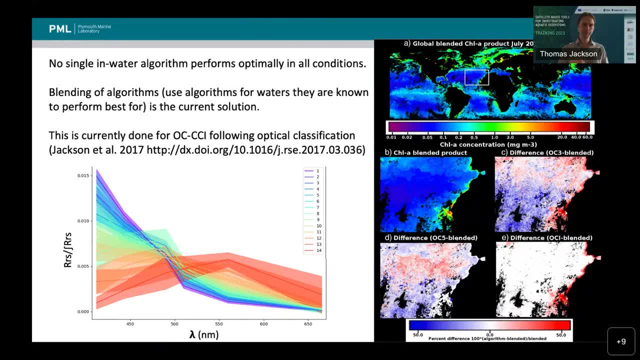 types, and those are shown in the the plot on the bottom left, and we know, or we can use in situ measurements to say which of the algorithms perform best in each of those types. memberships to all the types. we can weight the algorithms accordingly. So then, if you look at 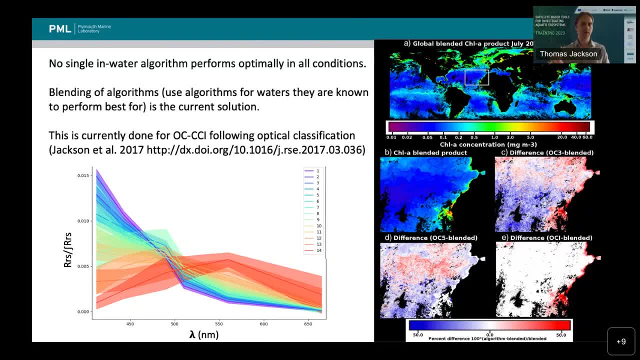 the image on the right. the top image is the output blended product And the idea is that this blending wouldn't introduce artificial boundaries. You don't get a hard line where we flipped from one algorithm to another. It's a smooth, continuous process of weighting. the 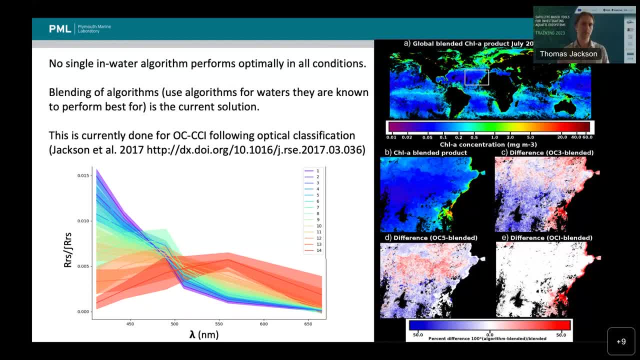 algorithms that are doing best in those optical conditions. And then so if we zoom in on the box area, you see the four lower figures And that's the blended product and then basically the contributions from three different algorithms which are going into that blending, But the final 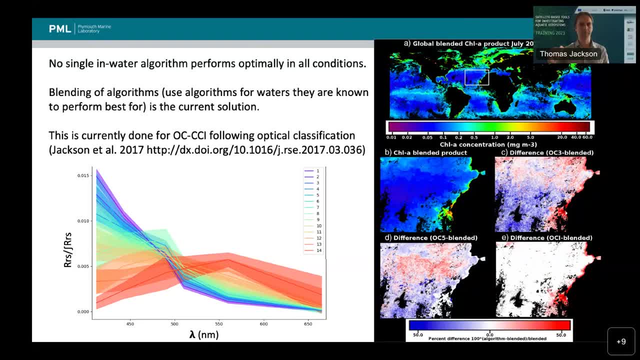 product is smooth, And you can see that the OCI algorithm is mostly used offshore, whereas the OC3 and OC5 algorithms are mostly used in – well, the OC5 isn't used closer to the shore in this example, And that's the final output product. So it's not just one algorithm, It's a blended approach. 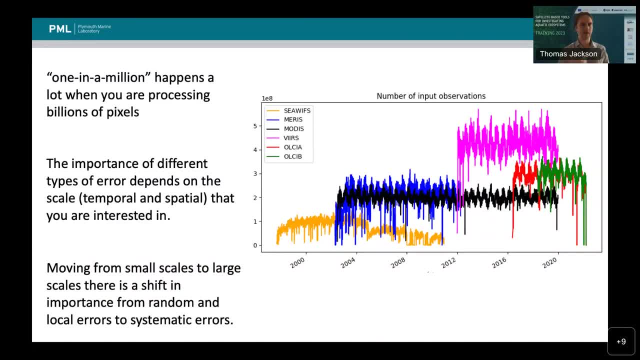 And so what I was saying about finding these bad pixels: it takes a lot of rigor and a lot of effort and a lot of checking to go through the climate records And in some ways we rely on the – we do a lot of that internally within the project, but it's also really useful to hear back from the. 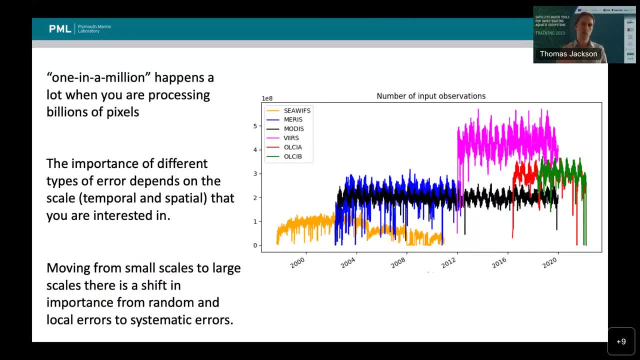 community when they've found things that are odd And that's gone on over the last decade within OCCCR. The next one is a quick analysis of the OCI, Because basically one in a million happens all the time when you're processing billions of pixels. So the y-axis on this chart the values naught to. 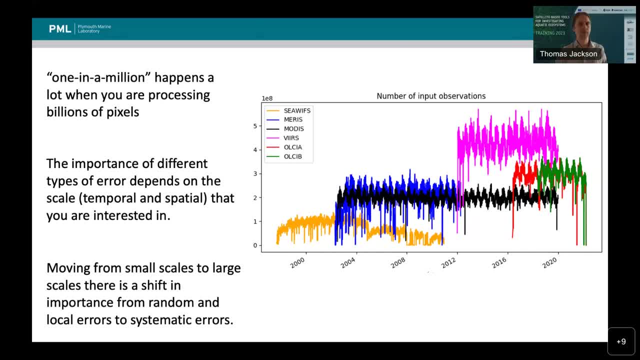 five, that is 500 million pixels or 100 million observations processed, And this is daily through our record. So you can see when VIIRS kicks in, that's 400 to 500 million observations per day, going into the total record. 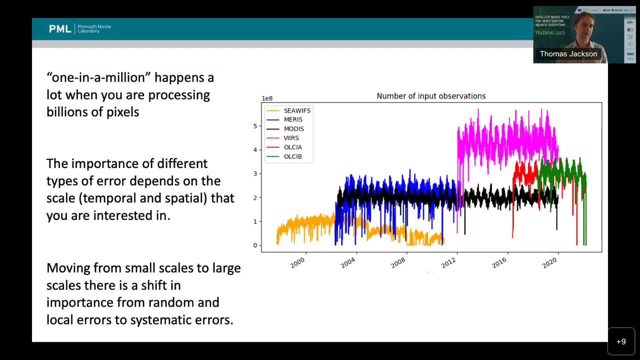 So it really is billions and billions of observations. So if there's a condition that could be tricky, we will have to deal with it at some point. Now I've talked about systematic errors and systematic issues like intersensitive bias correction, And we've pushed more into the kind of noise or the random errors that can be a problem. 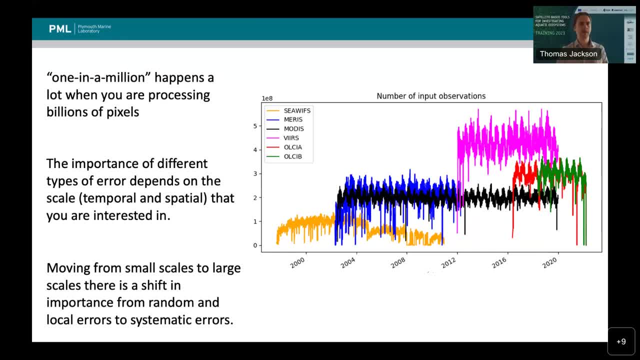 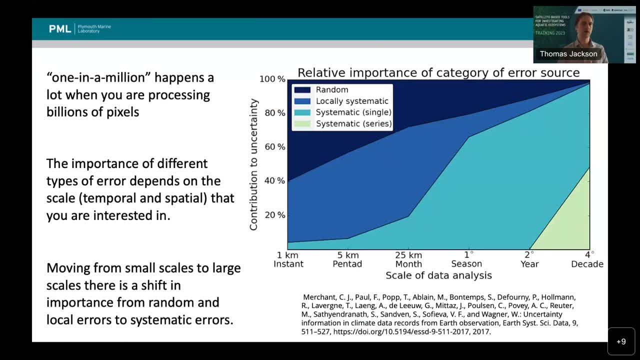 And that's often this one in a million type. And which of those errors is more important actually depends on the scales that you're looking at. So if you're looking at short timescales and small distances, the random errors are much more important. 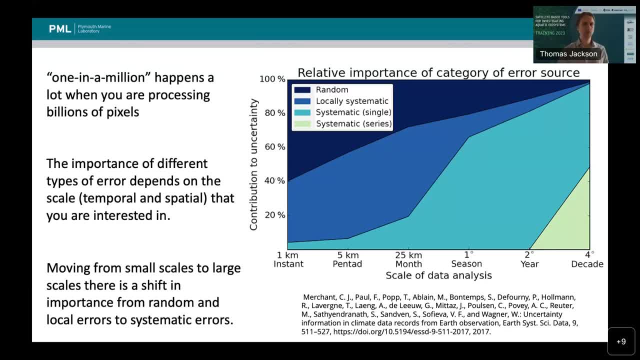 They will potentially corrupt your record. As we move to coarser resolutions, degree half, two, degree four, degree composites and long timescales over decades, they tend to average out and the systematic errors become much more important, And so it's just something to be aware of that, depending on the spatial and temporal timescale that you are interested in, 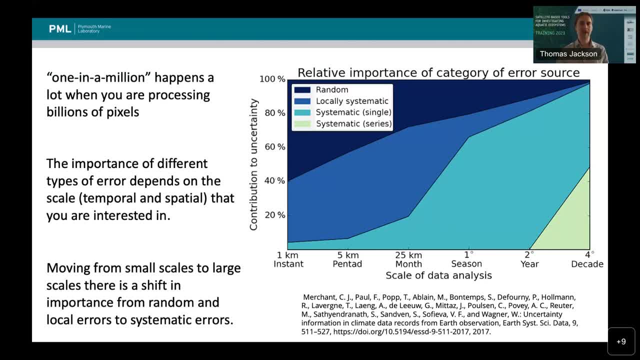 you have to pay attention to which errors are more important. As creators of a climate record, we have to care about all of this, because we don't know if our users are going to be doing stuff with one degree composites or if they want to be looking at one kilometre or four kilometre data for their local region. 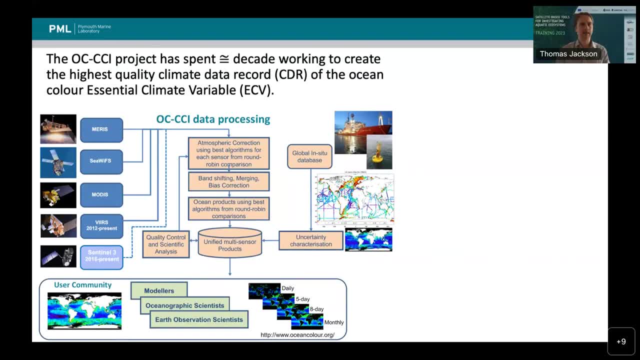 So, after all that, the OCCCI website, our project, has this processing system which ingests data from multiple ocean colour sensors And it goes through atmospheric correction. We have all the band shifting and bias correction, We have algorithm blending and we output products. 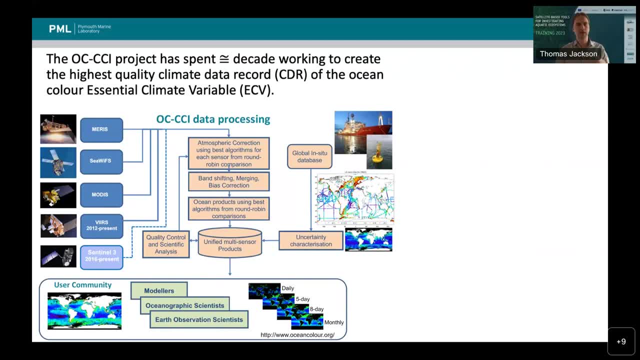 And those also have associated uncertainties, which allows them to be ingested into things like climate model analyses, And this is part of a cycle. So this we've gone round about six times now Six data set releases and plans are afoot for future data sets. 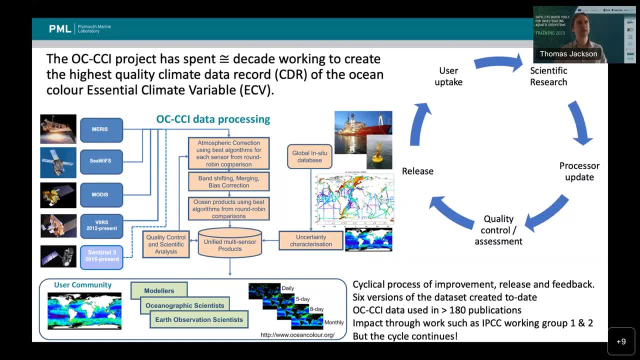 And we take it as a sign that the data has been good quality and taken up well, because we've always had good feedback. There's been over 180 publications now that have used OCCCI data And it's also gone through into really high level stuff like the IPCC working group reports. 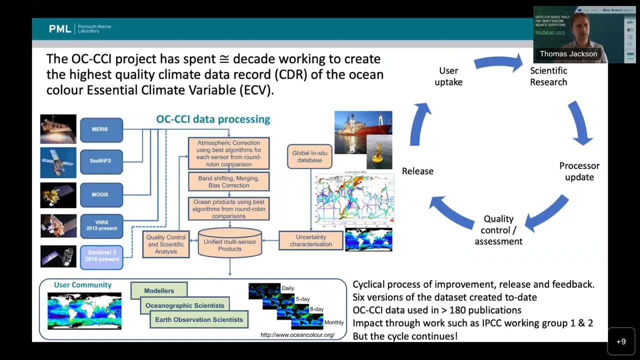 and the Copernicus climate change report, And those are the reports that come from that as well, The European State of the Climate report. But the cycle continues, It goes on, And I will just take one minute to say that part of that process. 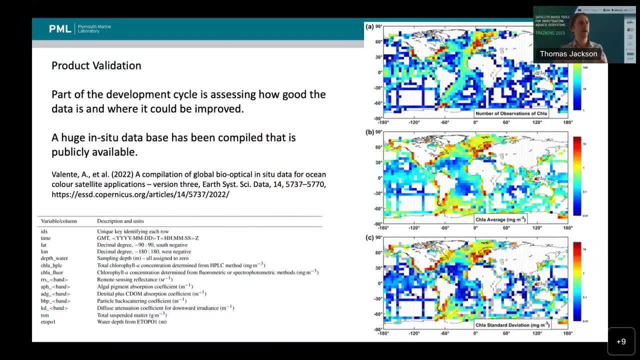 that validation and quality control and understanding how good the products are. it relies on good in situ data, And we've heard this in a number of lectures, So I'm just reinforcing the point that we cannot overstress the importance of in situ data for grounding the satellite data records. 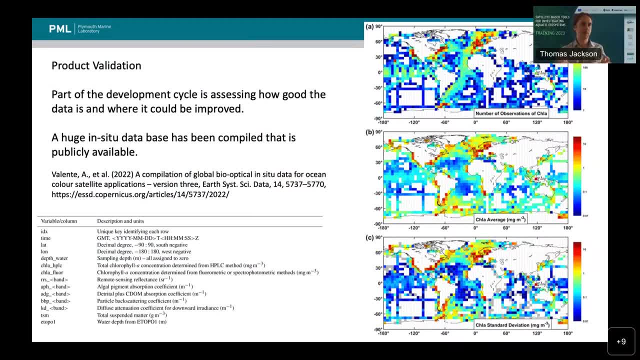 So within OCCCI there has been a compilation made of ocean colour in situ data So that's got reflectances and TSM and chlorophyll and absorption by phytoplankton and backscattering And that's publicly available. So I've linked to the paper there. 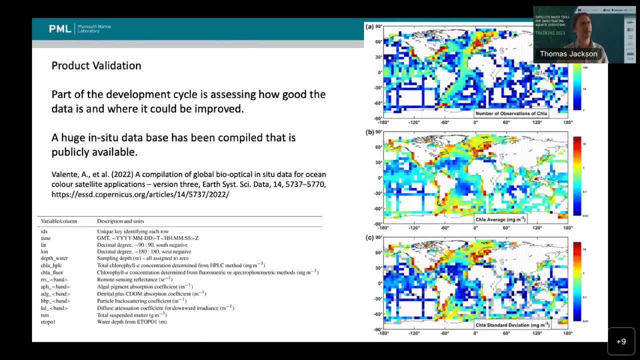 And the data sets on, I think, Pangea or ESSD And- and you can take that and have a look at it yourselves, Download it, Have a play with it And when we do that analysis for the OCCCI products. 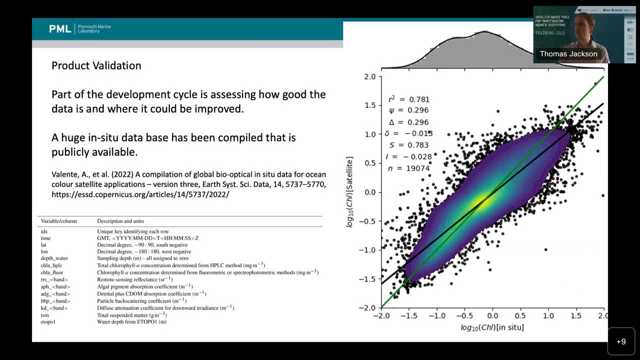 this is for chlorophyll. We get a pretty good relationship. You can see here that the bias- overall bias, which is the delta in here- is very low And that's good. That reinforces pretty much what we were trying to minimise with any biases in the data set. 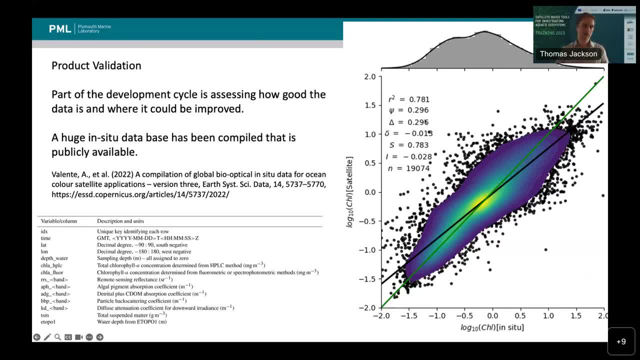 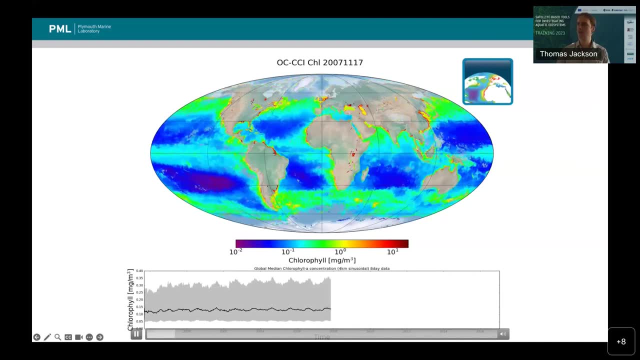 especially over a long time series, over the long time record. So, yeah, we have a pretty good performing global chlorophyll product over the 25 years or so of the record And it looks something like this at the long time scale: 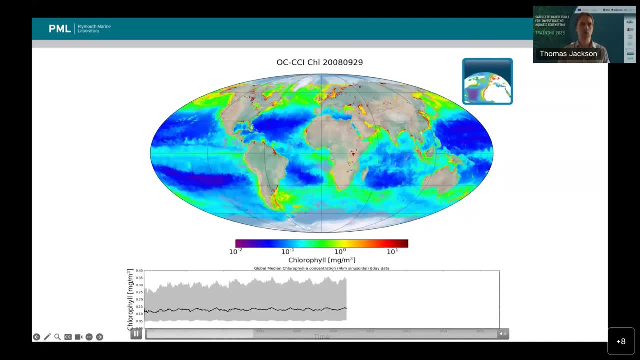 So you can see the blooms in the northern and southern hemisphere. You can see local dynamics of upwelling off the coast of Africa, You can see the Amazon plume and all these sorts of things And over the long time scale this is the global median chlorophyll at the bottom. 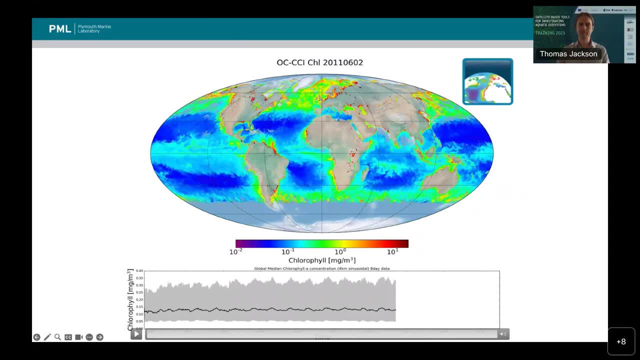 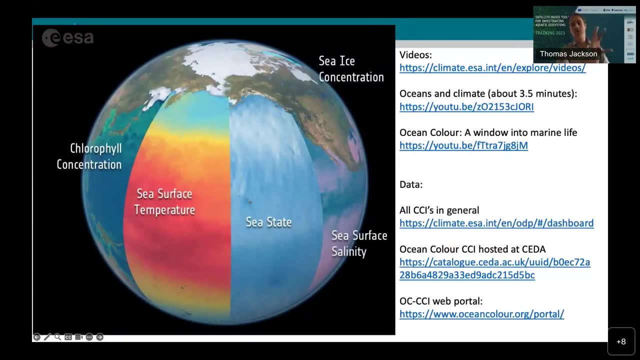 You can see that evolving over time. So we have this data set and then we have to use it. So also for a bit more information, please go see all these various places for either access to the data or there's a few useful videos. 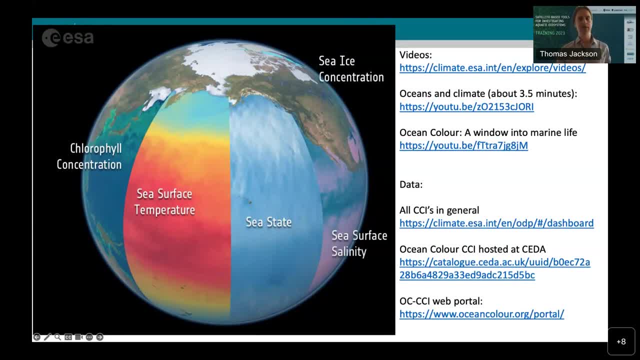 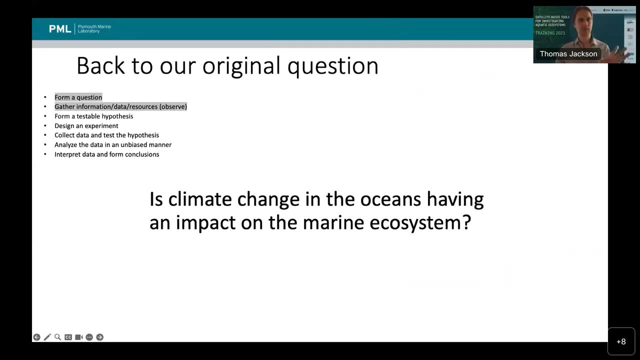 kind of introductions to the CCR project, all the different data that's available and why it's important, And so, again, I'll put all these in the thing at the end. So, coming back to this original question, we have a climate data set now that we're happy to use. 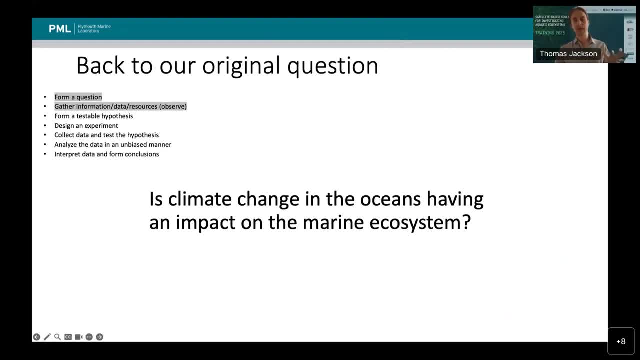 So can we actually see if there's any changes going on, And I'll speed up a bit at the clock. So we know the Arctic is likely to be an area where there's we need to detect. we would be likely to detect some change. 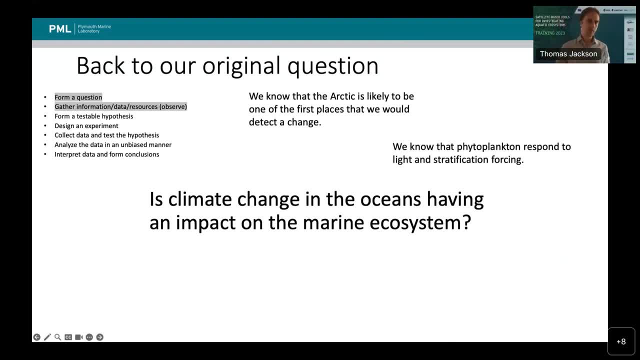 We saw that in the work from Stephanie Henson. Basically, that's where, if you're going to try and find something in a 20 year record, that's a good place to look. We know that phytoplankton respond to light stratification, forcing changes in nutrients. 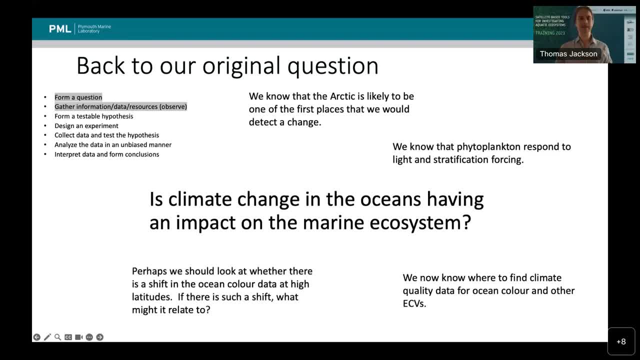 We know where we can get some good quality data now, So maybe we should look in the Arctic at ocean colour and see if there's a shift in the record And, if so, what might be causing it, And rather than just saying all latitudes, high latitudes, the whole Arctic. 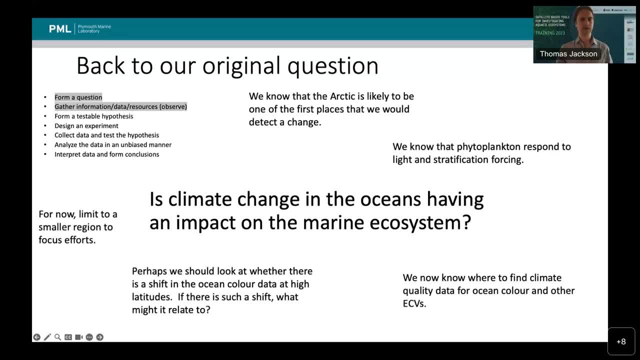 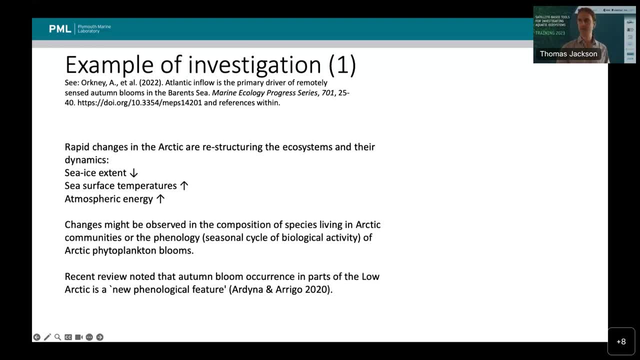 we're going to focus on a small region just for this demonstration purpose, And there's a nice example of this. It was a published paper from Andrew Orkney And the premise of that paper was that there's ongoing rapid change in the Arctic. 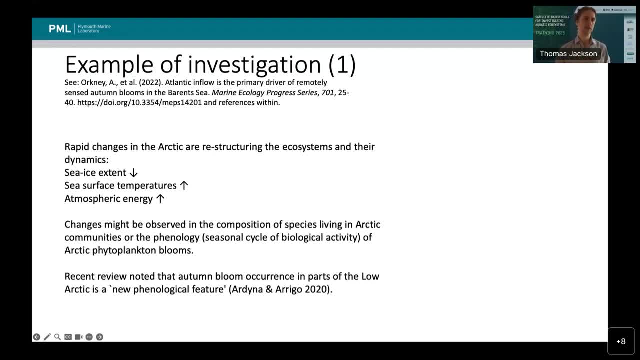 We know sea ice extent is falling, We know sea surface temperatures are increasing And we know the amount of energy in the atmosphere is increasing As well. potentially it's becoming more stormy or turbulent, So we might expect that with those changes, 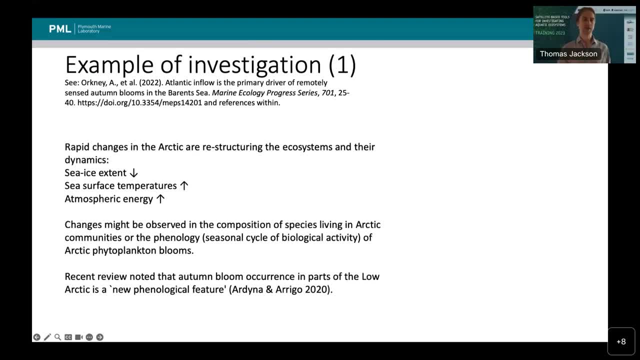 we would expect to see changes in either the composition or the phenology of the phytoplankton And you know there's a pretty significant changes and likely to have an impact from what we know around the drivers of phytoplankton growth. 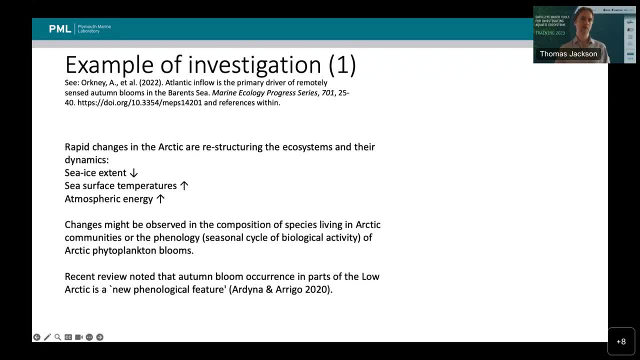 And there was a recent review that noted that autumn blooms have been occurring in the low Arctic as a new phenological feature. So normally in the Arctic it was classed as primarily just one bloom, rather than this spring and autumn bloom, But now we're starting to see spring and autumn blooms together. 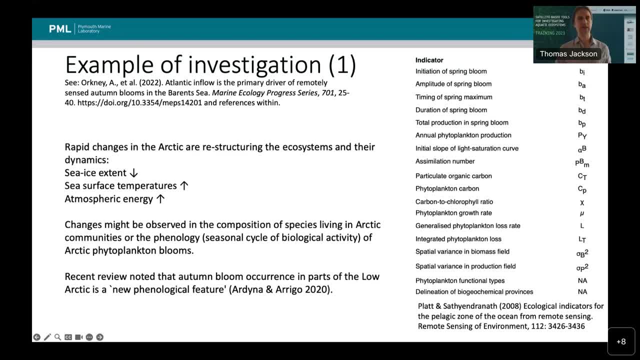 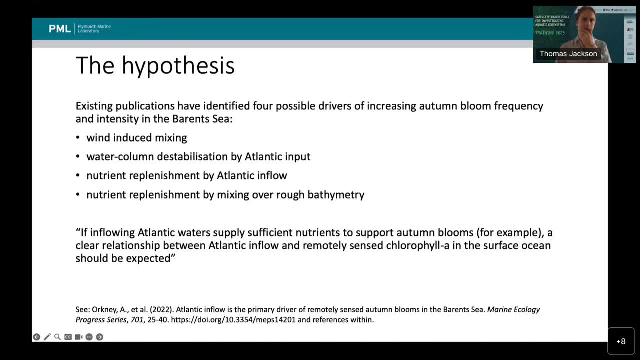 And again this is coming back to this list of indicators. So we're looking at what might be changing and which indicators we might use to look at that. So, after a literature review of the area and what might be changing and driving phytoplankton growth, 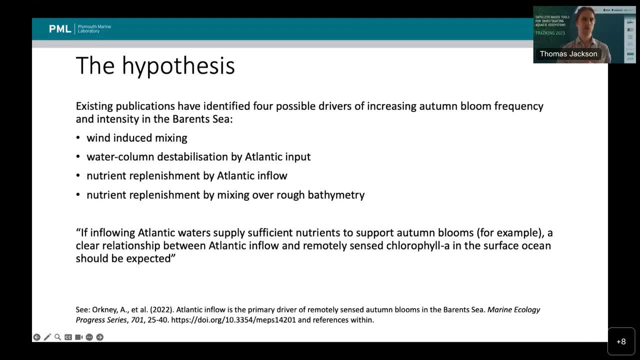 there were four candidates for what might be facilitating these autumn blooms or increasing the autumn bloom frequency. It could be more mixing from the wind. It could be water column destabilization from Atlantic inflow. It could be nutrients coming in from the Atlantic, ie more nutrients coming in and promoting more blooms. 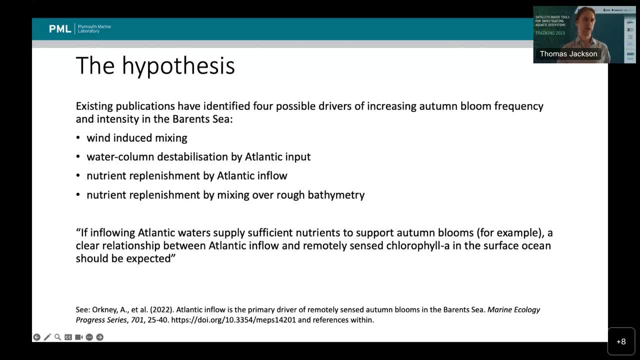 Or it could be that there's enhanced nutrient replenishment from mixing over bathymetry sea bed features. So the hypothesis to test basically is that if the inflowing Atlantic waters are supplying nutrients to support these autumn blooms, then a clear relationship between the Atlantic inflow and remotely sensed chlorophyll would be expected. 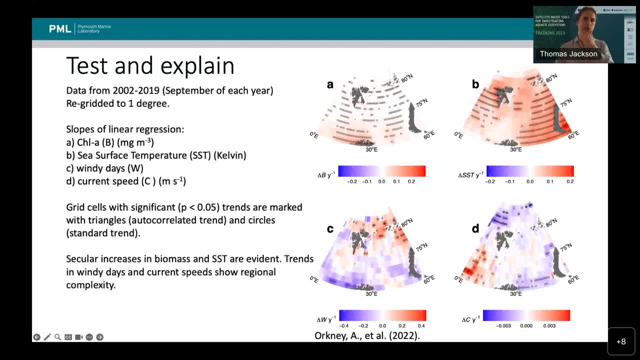 I have a nice hypothesis to test. So in that study they went and they looked at a number of variables. So in the top left here we've got the trend in chlorophyll. In the top right we've got the trend in sea surface temperature. 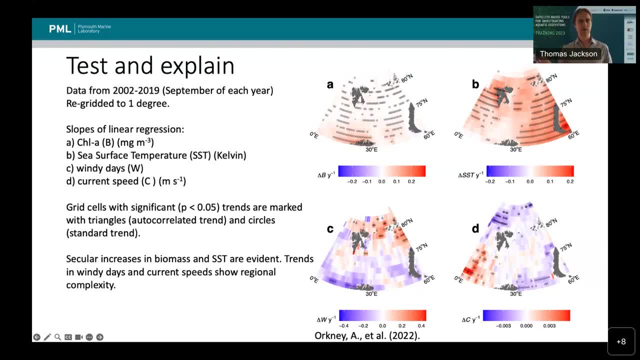 In the bottom left we've got the trend in windiness And in the bottom right we've got a trend in the currents, And this has been re-gridded, I think, to one degree, And they've taken only September data across a 17 year record, which I think is the record that was available for all the variables. 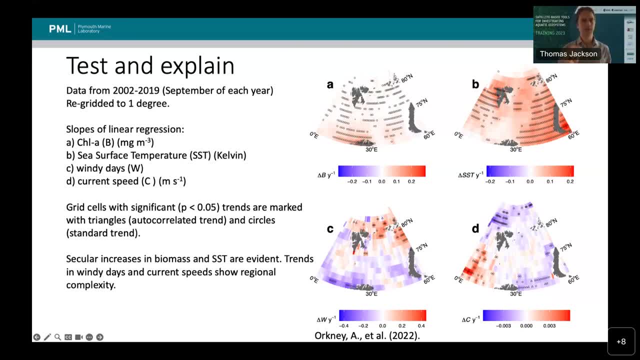 And you can maybe see those little circles and triangles. The difference between those is to do with autocorrelation. Again, I'm not going to go into detail on that now, But basically all the points that have either a circle or a triangle were classed as significant trends. 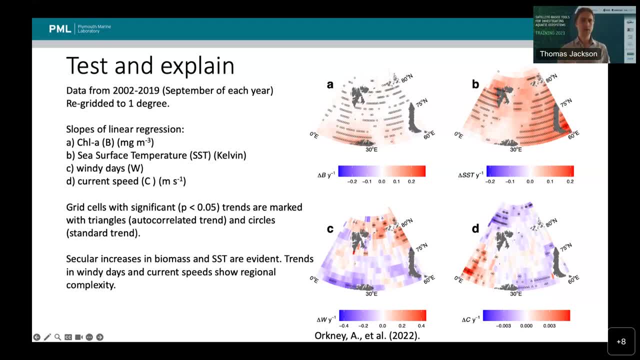 So statistically significant And what you can see is that basically, the chlorophyll and the temperature in September are increasing pretty much everywhere. There's nowhere where they're really decreasing, Whereas the patterns in the windiness and the current speed are a bit different. 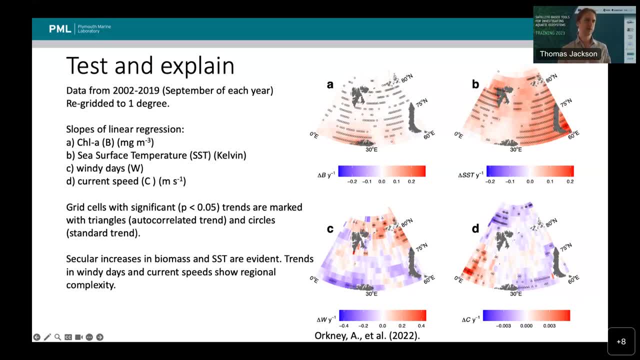 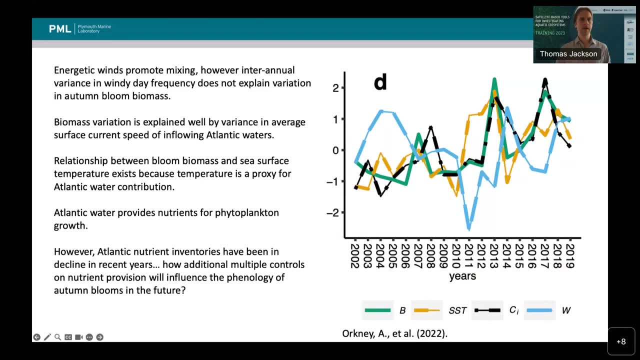 You could say that the chlorophyll is maybe increasing more in the southwest and not so much at the highest latitudes, Whereas temperature is increasing pretty much everywhere And if we look at a time series of these across the region, So you can see the chlorophyll in green. 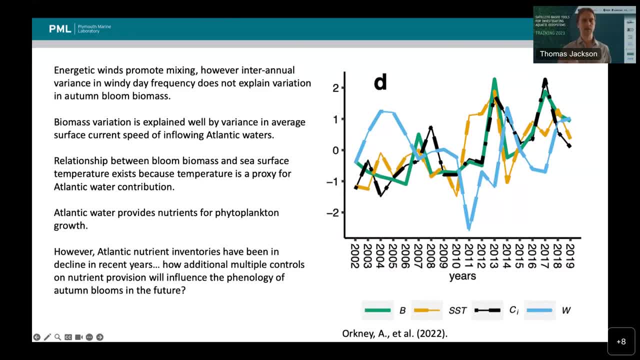 We have the SST in orange, The currents in black and the windiness in blue, And the strongest agreement of any other variable with chlorophyll is for the currents. So this is the black line and the green line. So, although energetic, So although energetic winds do promote mixing, 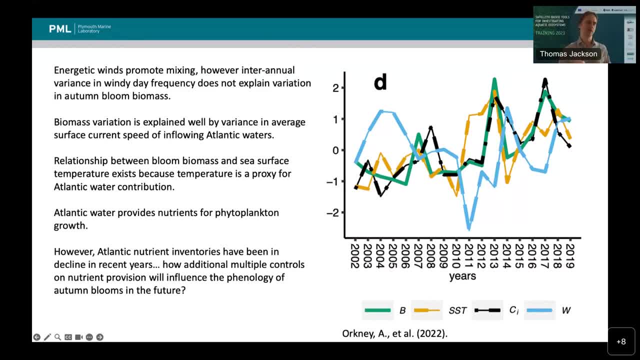 The inter-annual variance doesn't agree with the change that we see in the biomass, But the current speed does So. although there is a hint of a relationship between the bloom biomass and the surface temperature, That's actually more likely due to them both being forced by the Atlantic inflow rather than there being a direct forcing from the temperature to biomass. 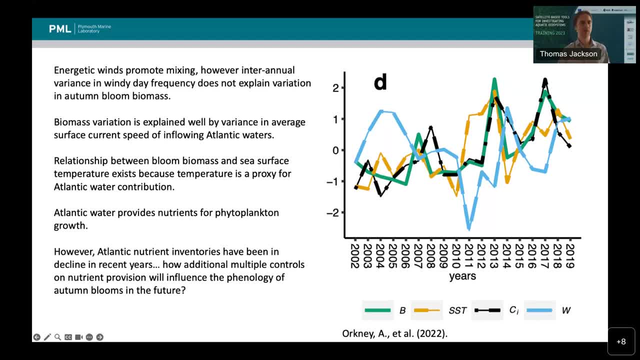 But an interesting side note on this or point from the study was that although here it looks like an increased Atlantic inflow, or Atlantification as it's termed, Is pushing the biomass for the autumn bloom up, It might be that the- or it seems that there have been studies to show the Atlantic nutrient inventory has been decreasing. 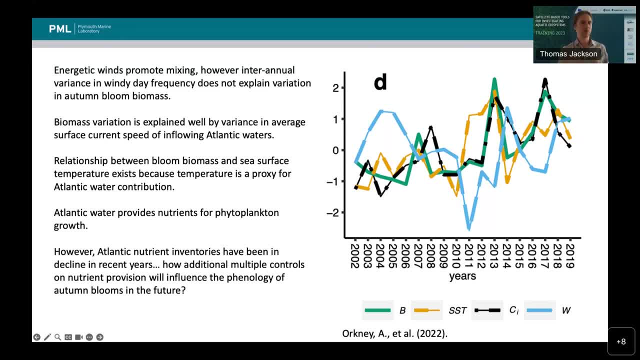 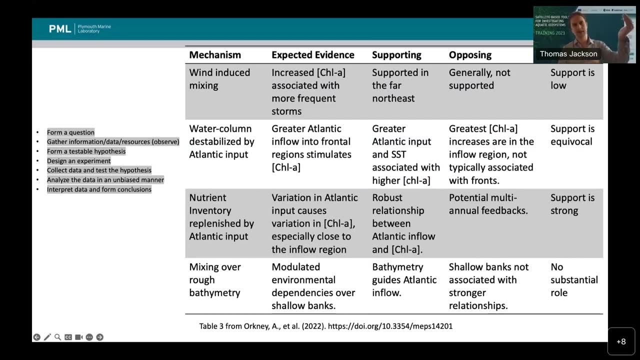 So it might be on longer timescales. We might see this change reverse, Because additional controls on the nutrient provision might actually dominate. So we'll have to wait and see. But in summary, basically this study has gone through that whole process that we discussed right at the start about forming a question. 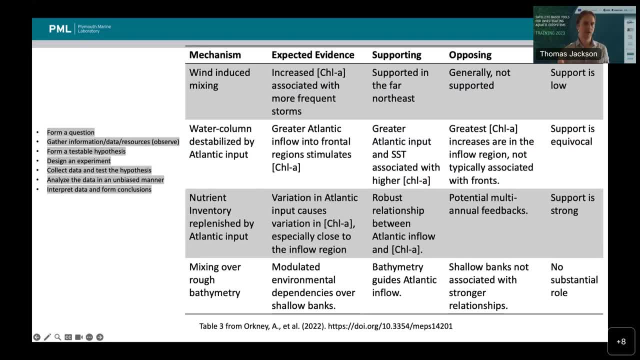 Getting some relevant data, Creating a testable hypothesis, Analyzing the data in a clear manner And presenting the summary results and the conclusions. And basically, here It's that the strongest support was for this increased nutrient inventory from the Atlantic, Whereas for the others we didn't see as such a strong support for that hypothesis. 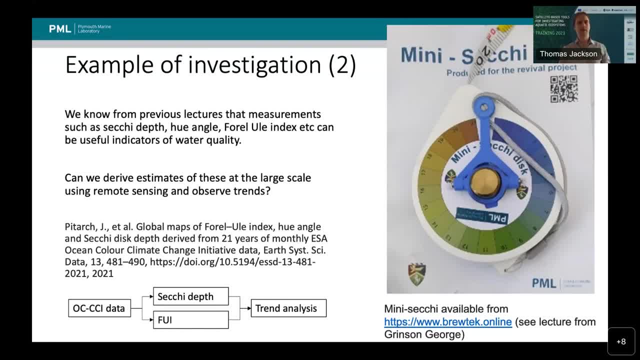 So, moving on to a second, just a quick example here, And the reason I put this one in is I think it ties in nicely back to some of the work from module 2. Where we saw Grinson talking about the mini SECI and water quality indicators. 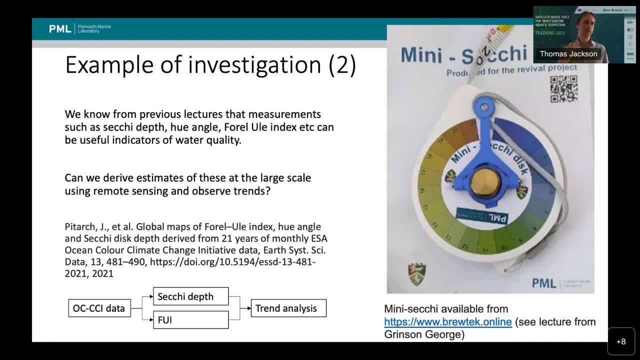 So in those lectures we were told things like the SECI depth, the hue angle, the index are really useful indications of water quality. So can we look at these as a climate record? Can we take our climate record of ocean color and try and look at water quality across those scales? 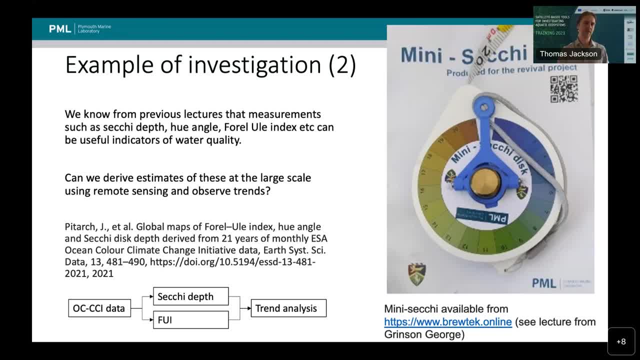 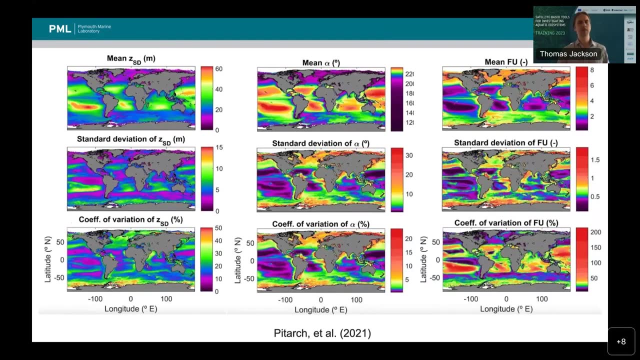 So there was a study from Shane Patak and others which took the OCCCI data as input, Developed some algorithms to calculate SECI depth And the index And then performed some trend analysis on that. So the maps that they produced of SECI depth, hue angle and can be seen here: 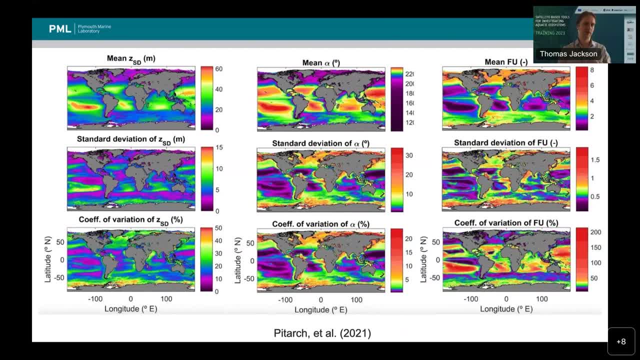 I wouldn't worry too much about the standard deviation or coefficient of variation right now. If you want to dig into it more, go to the paper. But you can see in the mean panels in the top that these they make sense. The deep blue oceans, the gyres, have a very low FU index. 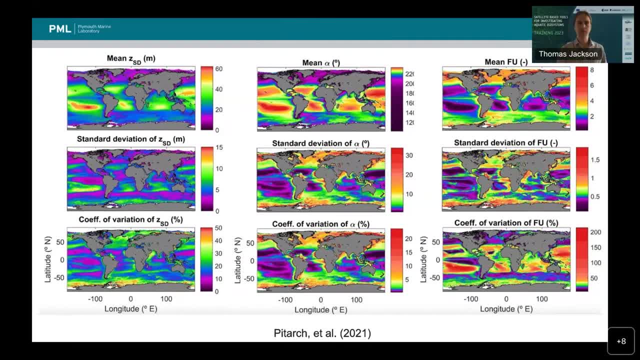 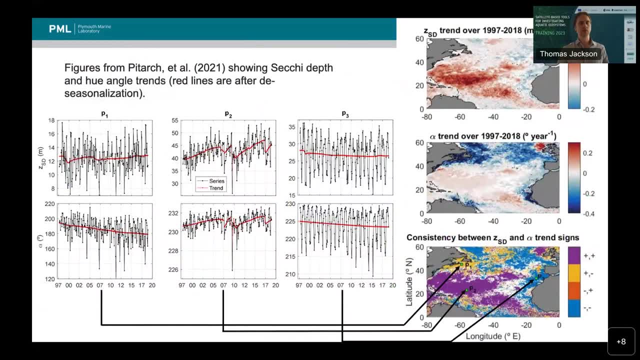 The SECI depth is very high or deep compared to the coastal waters and the Arctic, for example. So then, what they did was they took those products and analyzed them across the time series, So the 20 plus years of CCI, to look for trends. 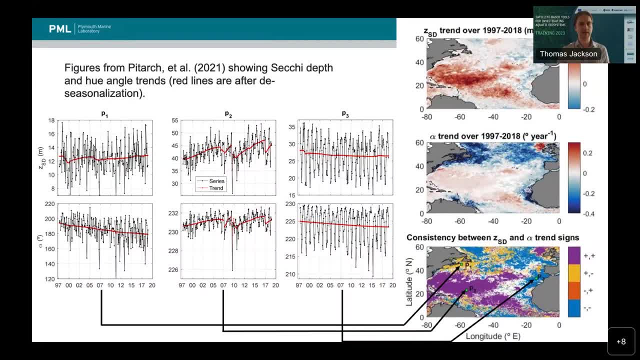 And so here you can see a panel for the North Atlantic. The columns left to right, P1 to 3, are three different areas shown here. So we've got the northwest And the south, We've got the Atlantic, We've got the central gyre. 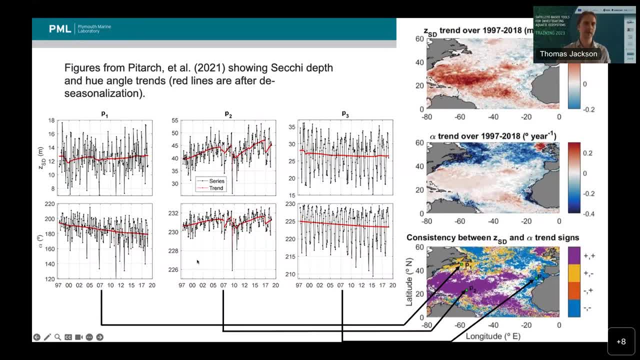 And we've got the eastern Atlantic And you can see if we look at the SECI depth on the top and the hue angle on the bottom, they have potentially different trends in different areas. And that's just for three individual pixels. But then if you look at the trend in the red line here, which is the de-seasonalized values, 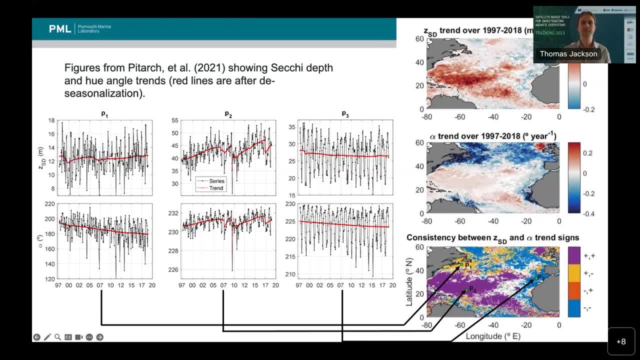 So there's a seasonal cycle And then they've de-seasonalized it to get the red line. The trend in that for each pixel is shown. It's shown in these two panels And you can see it looks like there's an increasing SECI depth in the central gyres with the waters becoming clearer, reflected also in the change in the hue angle. 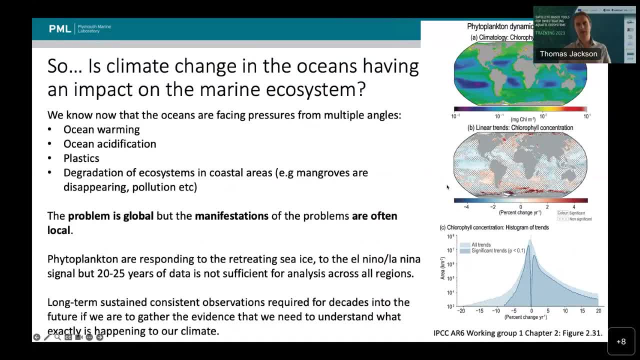 So, going back to our big question that we posed a long while ago. Sorry, it's taken so long to get all the way back to this, But if we look at climate change in the oceans And if it's having an impact on the marine ecosystem, 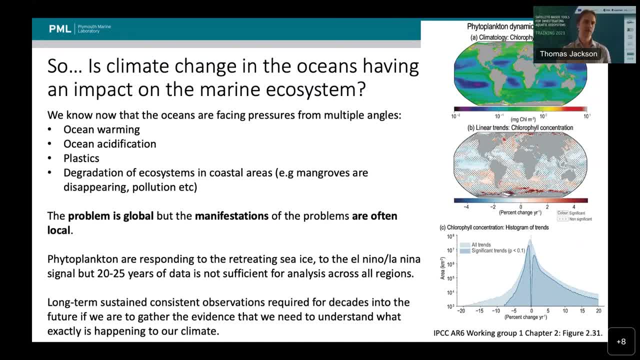 Well, we know that the oceans are facing pressures from multiple angles. There's ocean warming, There's acidification, There's pollution and plastics. There's definitely stress on coastal areas. We've seen mangroves disappearing and all these sorts of things. 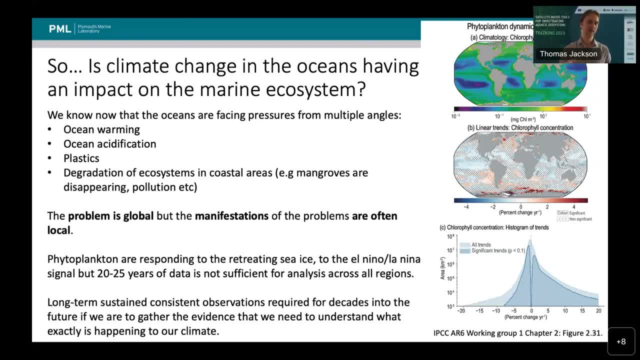 And although the problem is global, as was shown by the study in the Barents Sea and also in this map that I'll go into in detail, a little more detail on the right from the IPCC- It seems that the manifestations are local. 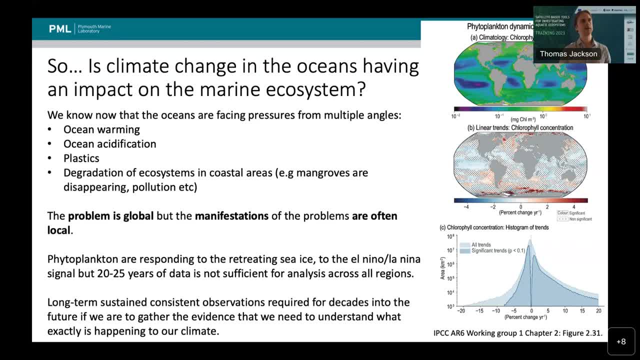 So it's not like sea surface temperature or atmospheric CO2, where we have a unidirectional trend where everything is warming or everything is increasing. The dynamics of the ocean mean that some areas might be seeing more biomass. Some areas might be seeing less biomass. 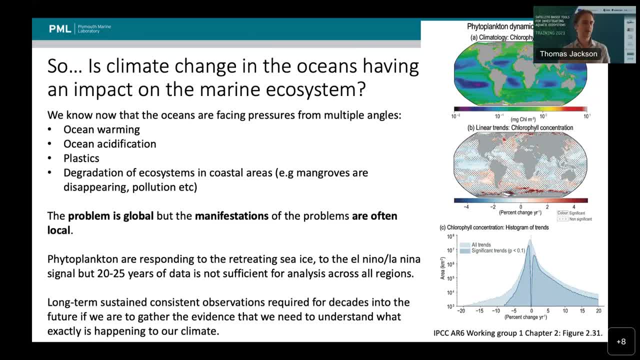 Not only that they might have the same biomass, but it's a different species or a different community, And Heather will go into details on what that might mean later. But it's really. we have to look at the local scale to try and see the expressions of this broader change. 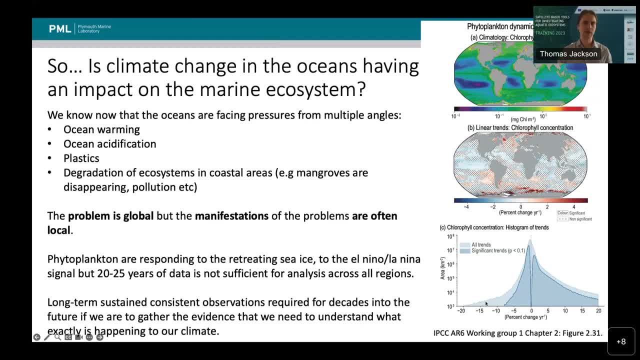 So this is a panel just from the IPCC AR6 working group in Chapter 2.. And this middle panel- sorry if it's a bit small, but this is showing the trends at the global scale for different areas. So you can see the Arctic is seeing an increase in chlorophyll. 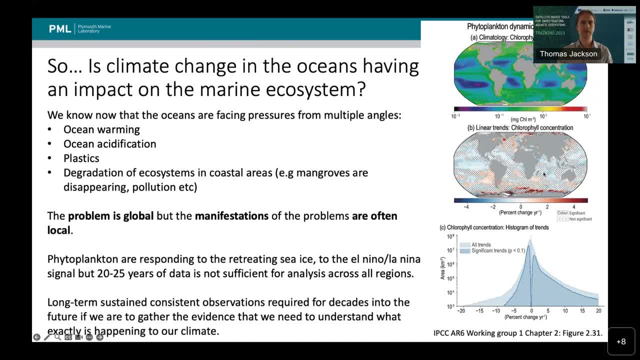 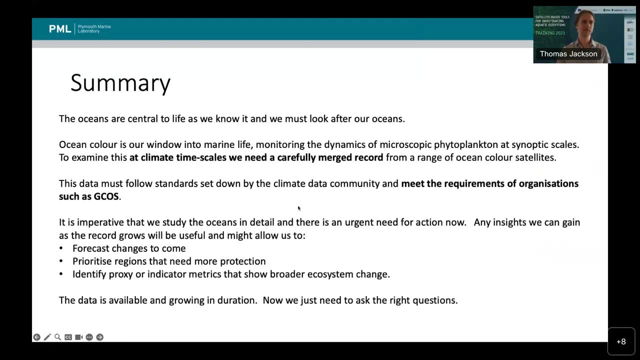 The gyres, potentially, are seeing a decrease And it really depends where you are as to what sort of features you would expect to see changing over the next 10 years and have changed over the last 20 years. So just in summary summary of the whole talk, the oceans- we can't stress this enough through all of these talks- is fundamental to how the Earth system functions. 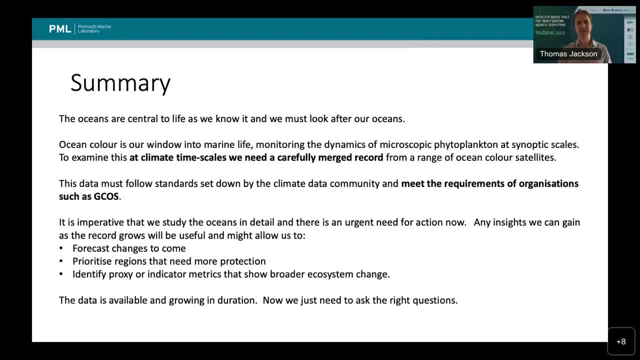 And we have to look after them. Ocean color is our only window really into the base of the marine world. We have to look after the food web and the marine ecosystems So we have to see any way really to monitor the microscopic plankton at the synoptic scale. 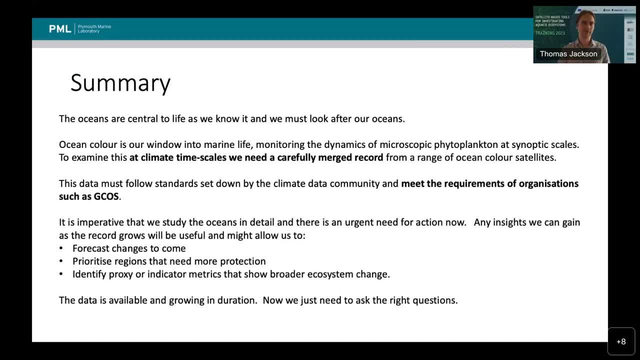 And to examine this at climate scales, we need a very carefully merged record from multiple ocean color satellites, And that record has to meet the requirements of the climate community laid out by organizations such as GCOS. And basically, now we're at the stage where we just need to look at the climate. 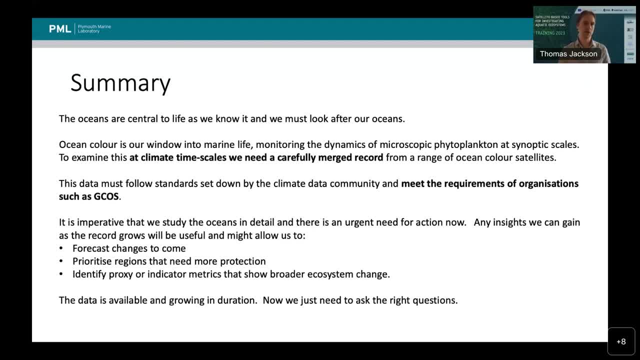 We're at the stage where we just need to use those records and really start asking good questions. So, whether that's looking for forecasts of change to come by looking at what changes we're already observing, or if it's prioritizing regions that might need more protection, because we see that they're changing very rapidly, 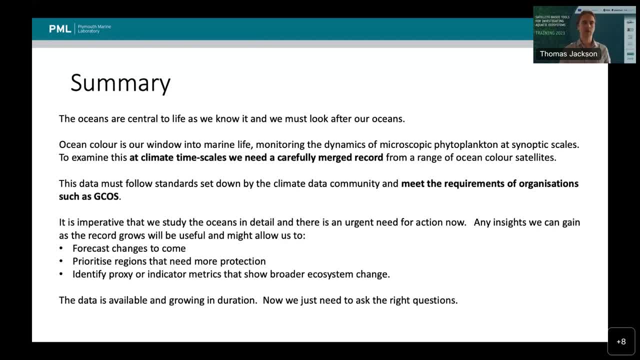 Or if it's identifying proxies or indicator metrics where we see something in the ocean color record that might be representing a much bigger ecosystem change. But now it's basically we can say: the data is available, It's growing as we continue to make the record longer. 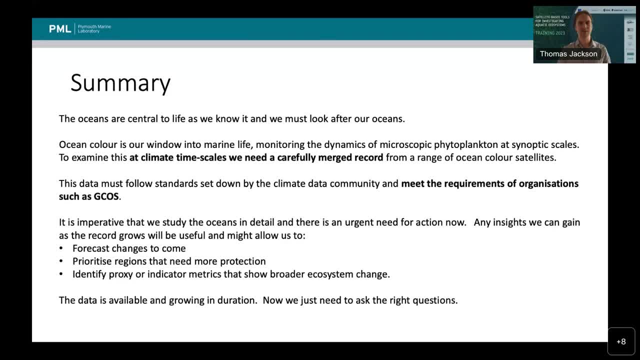 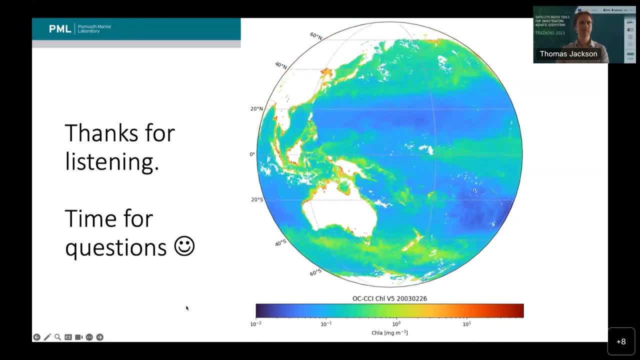 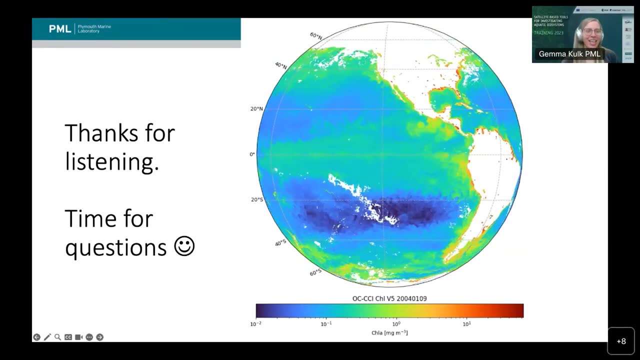 And it's over to the community to ask the right questions. So thank you very much And I'll just leave that there. Thank you, TJ, for this really wonderful presentation. Marie-Helene, are you there? Yes, I am. 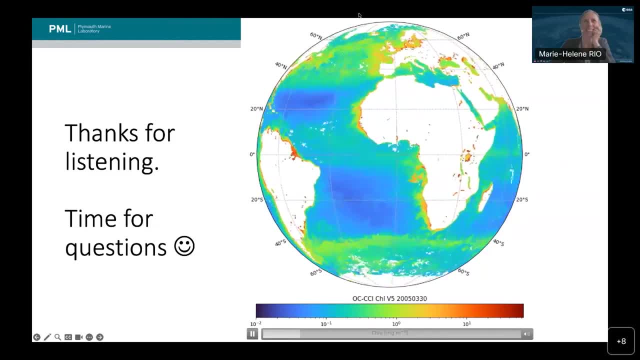 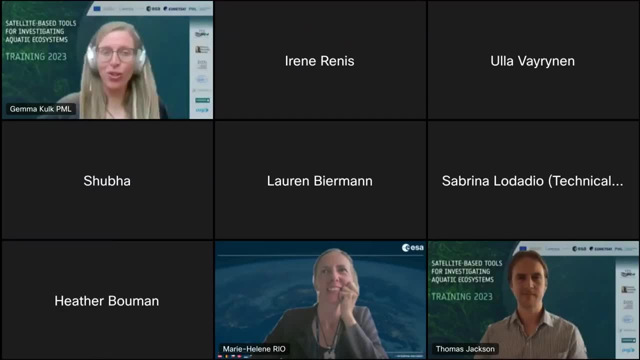 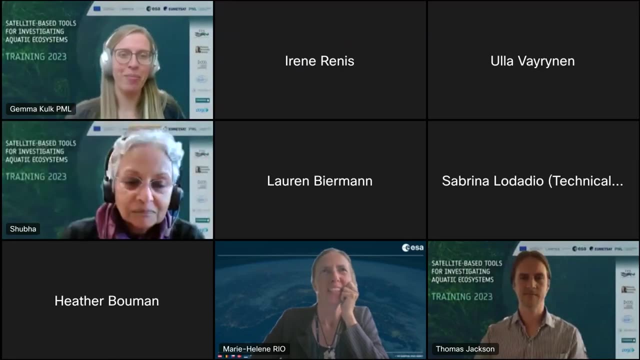 Perfect, I've already introduced you before at TJ's lecture And I thought now would be a good time, before we go on to Q&A, for you to tell us more about the activities of ESA on the topic Sure. Thank you very much, Emma. 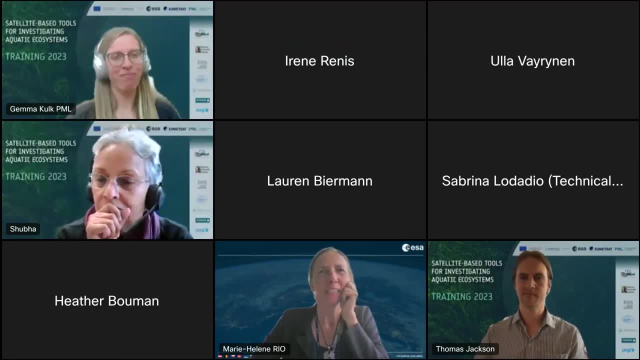 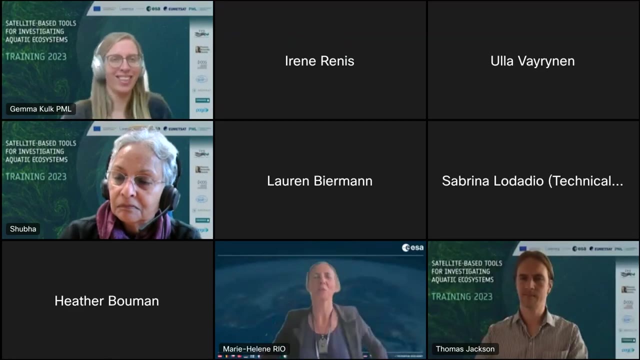 And I apologize for the small technical issues encountered, But let's do it now. And actually, Thomas mentioned quite a few elements that you will find Again in my introduction, So it was very nice to hear. I will share my screen. 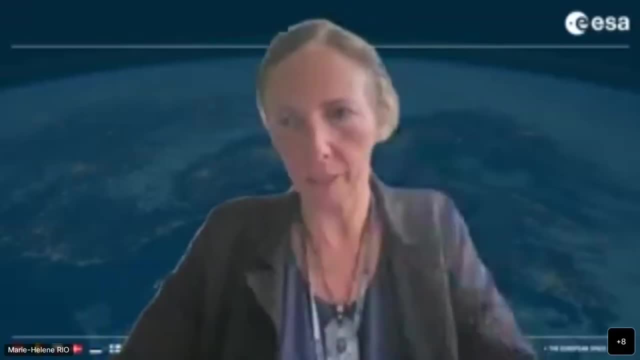 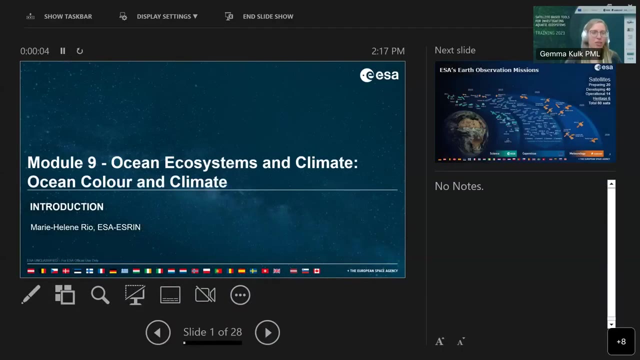 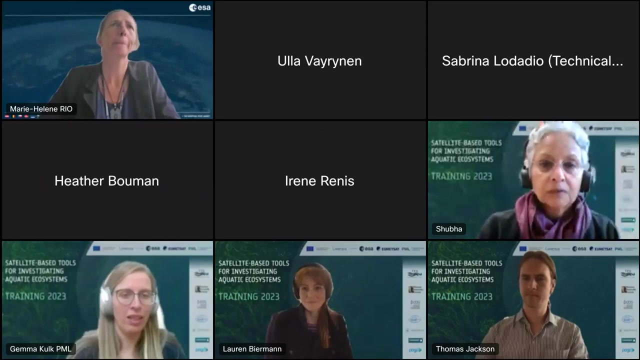 And tell me if you see the presentation In the right. No, we see your presenter mode. Okay, So we will. Now we should be okay. I lost your screen. Okay, So let's try again Where I am, Okay. 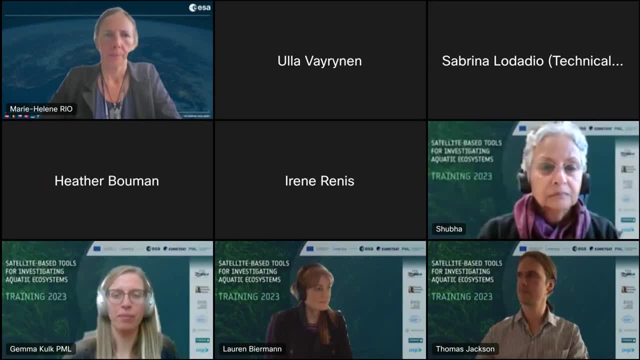 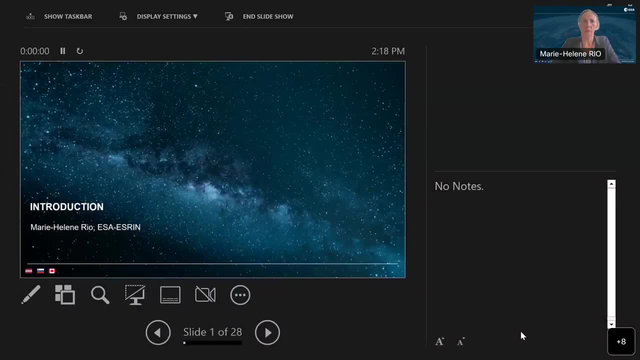 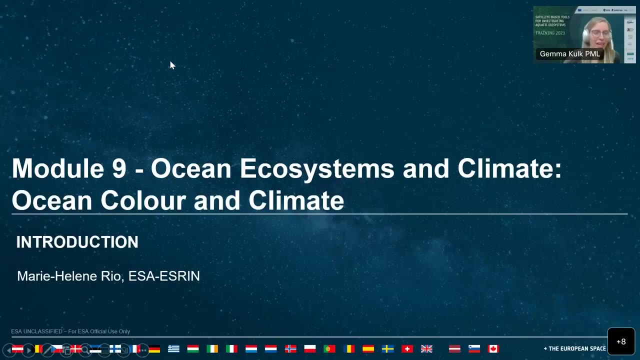 Share And do it again. Now, what do you see? Still the presenter mode Now. Yes, Perfect, We will manage. Okay, Good afternoon, Good morning Everyone. Very nice to be here. Thank you for the invitation. My name is Marie-Hélène Riau. 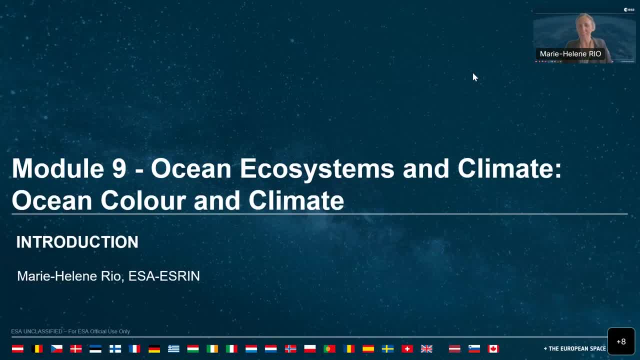 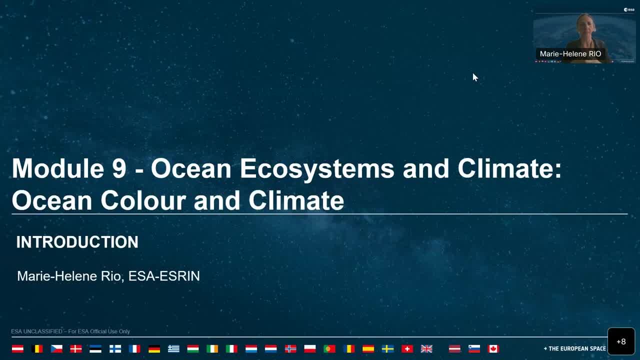 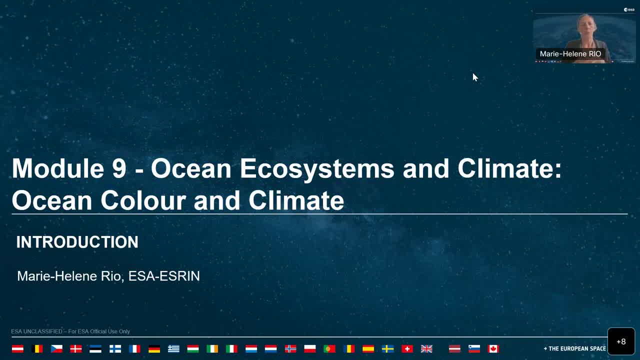 Space Agency on the topic. Of course it is very short, Don't hesitate. maybe to get the slides. uh, go to the links i put in the slides to the different projects, and at the end i also give my email, and so you're very welcome to contact me for any questions. so the european space agency. 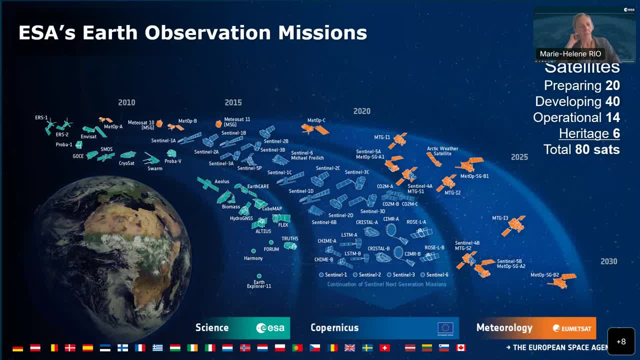 okay, here we are. together with european and global partners, contributes to develop world-class observation systems to address scientific and societal challenges. and here you can see the very complete set of earth observation satellites that we have currently operational, being developed or being prepared, so it's actually a 14 satellites. 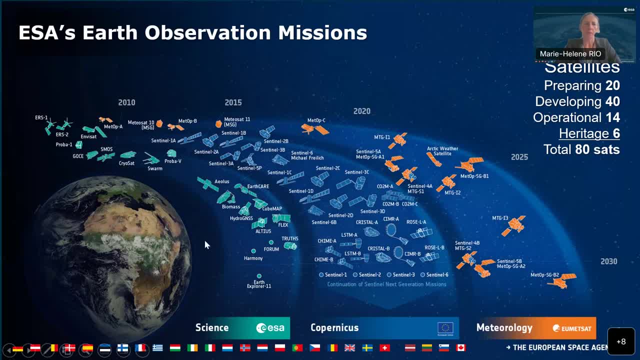 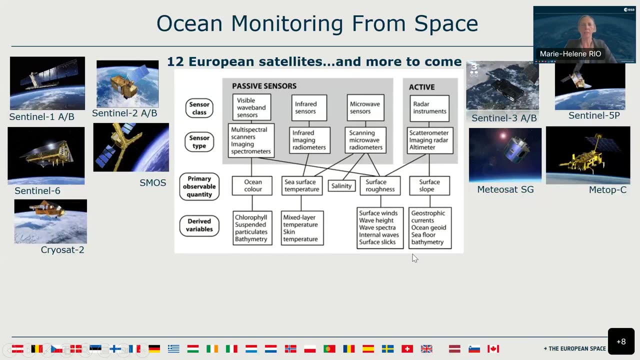 operational level of today with a different lines: science missions, the operational mission with the european copernicus initiative and the meteorological mission. when we look at ocean, a number of satellites used to monitor the ocean from space and providing information on many different variables that you can see here, using different sensors, passive and active sensors. 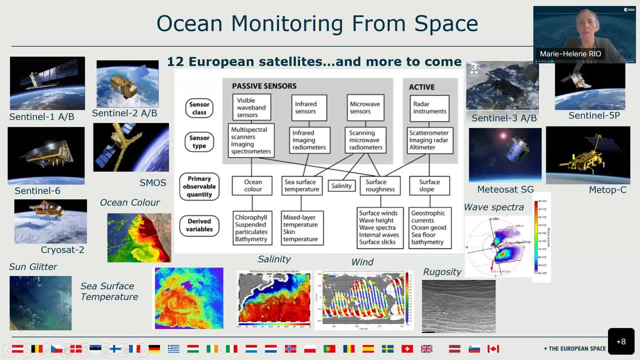 and so we have a number of parameters that can be used to study and to monitor, to better understand our ocean ecosystems and ocean health. so one of these parameters, of course, is ocean color. it's not the subject of the webinar today, but, together with all other parameters, again we have 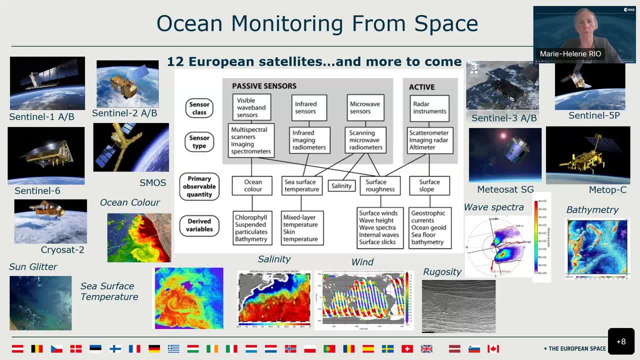 the information, or we have a substantial set of information needed to do science and to to have a look into these key issues regarding ecosystem and climate. so, to exploit this large amount of data, we have a number of programs ongoing, and the first one you already heard about in thomas's book is the 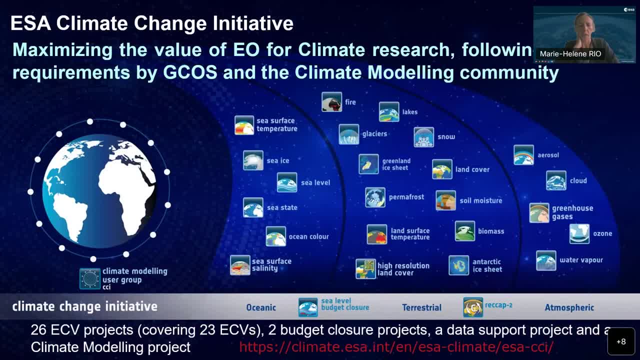 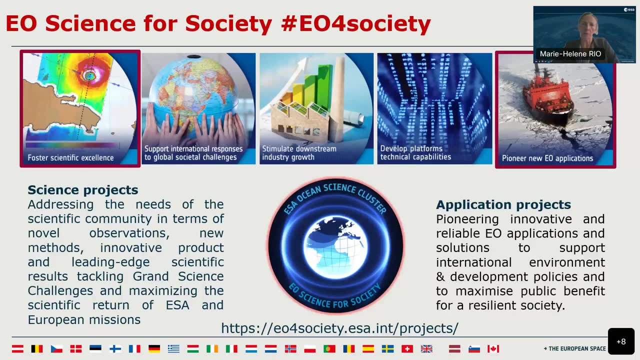 isa and climate change initiative, which was launched in 2008,- so 25 years ago- in response to the UNFCCC request for having a systematic monitoring of the climate system. So, through this program, what is being done is to develop the data records of key components. 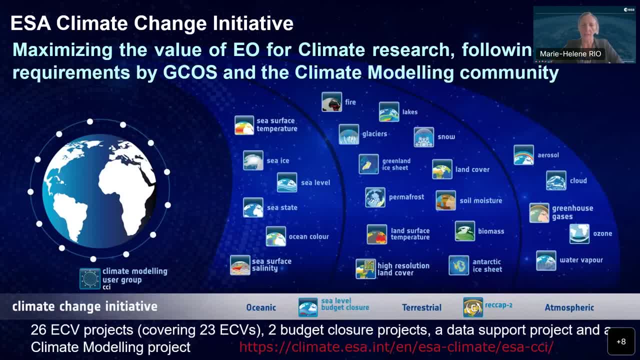 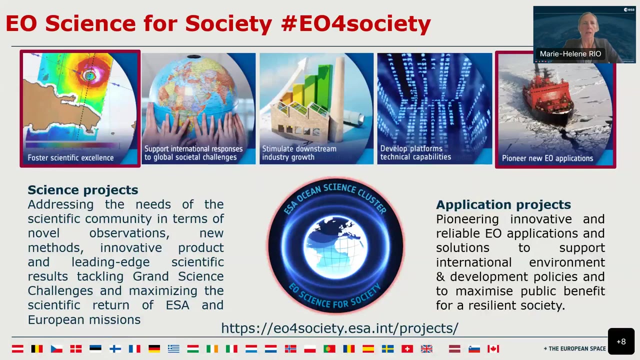 of the climate system which are known as essential climate variables. So there are 26 ECBs. so essential climate variable projects ongoing two-budget pleasure projects and the climate modeling project and other support projects. All the data you can download at the link below and find more information also there. 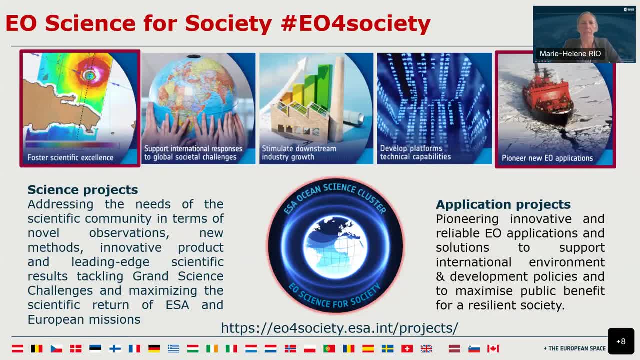 Another important program that we have is the EOScience for Society program, which has a number of objectives that you can use. You see here, in particular fostering scientific excellence. So this is done through the development of a science project where we address the needs. 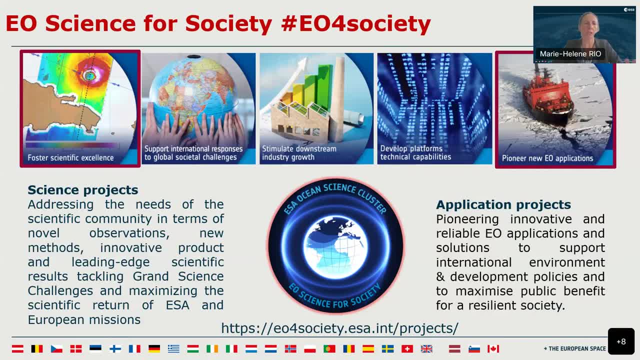 of the scientific community in terms of new observation, new algorithm development in order to tackle grand science challenges. The second important component, important objective is to pioneer new Earth observation applications. So we have a number of objectives. So we have a number of objectives. 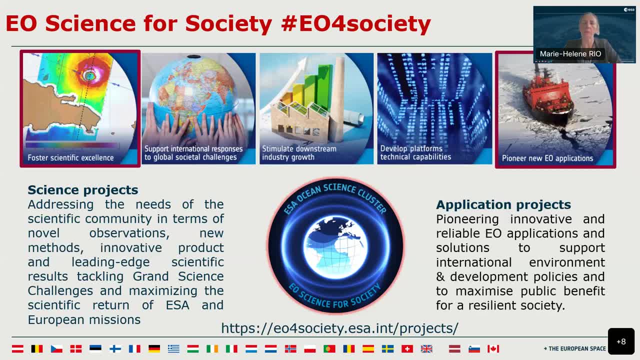 So we have a number of objectives Here. the objective is to really foster the use of remote sensing to develop new and reliable Earth observation application, to support international environment and development policies and maximize the public benefit of the Earth observation system. So the numerous projects that we have, they are gathered here into what we call the EOScience. 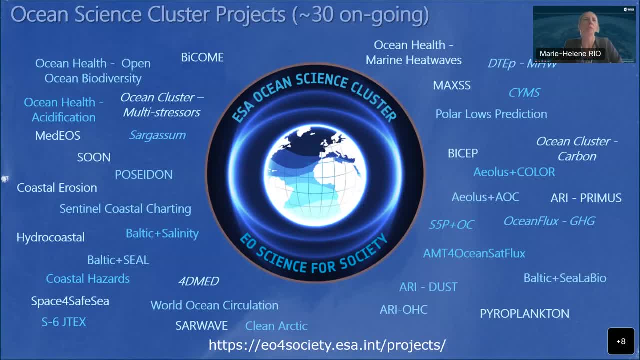 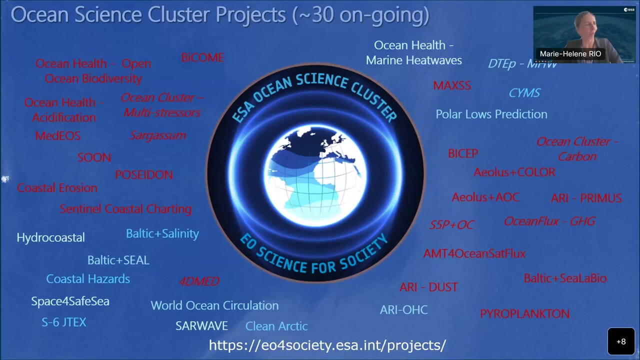 EOScience Cluster. EOScience Cluster- And I put here on this slide the names for the different projects that are running, actually more than 30. And among those I put here in red, the one which are based not only, but which are based: 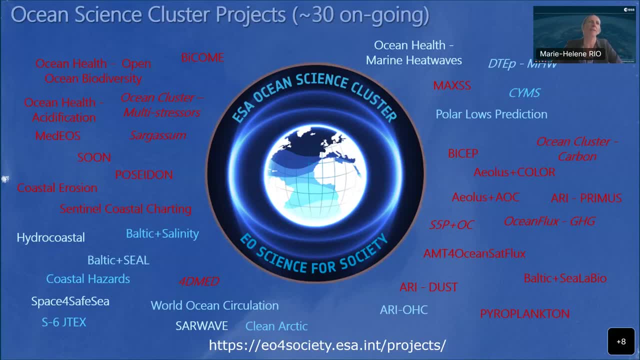 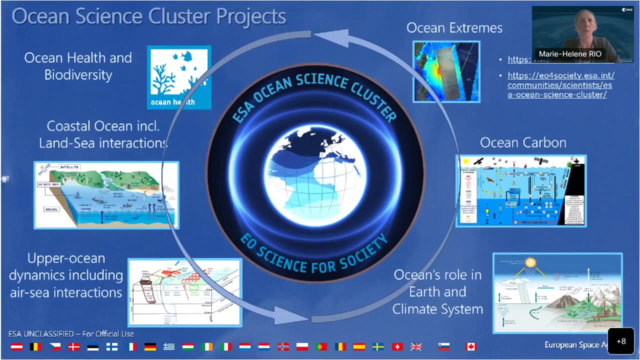 on the use of ocean color and geometry data from the different sites And those different projects. we have a number of objectives. We have also further cluster them to different topics which are linked one to each other, But we can identify a main. 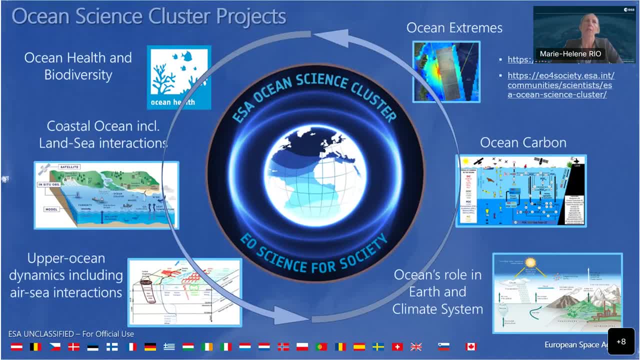 And so we have projects looking at ocean health and biodiversity, projects on coastal ocean and land interactions, projects investigating operation dynamics, including Earth interactions. We are also looking at ocean policy and conservation at the ocean, extremes at the ocean carbon cycle, and that the oceans fall in the Earth and climate system. 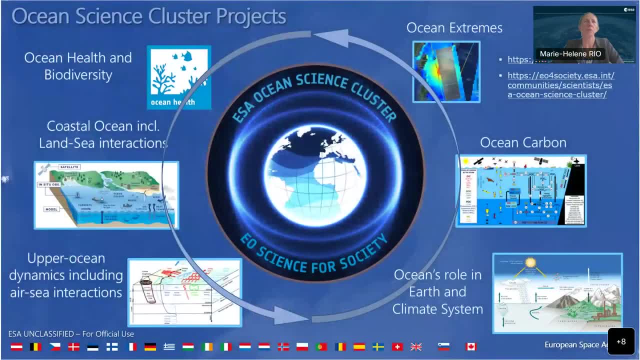 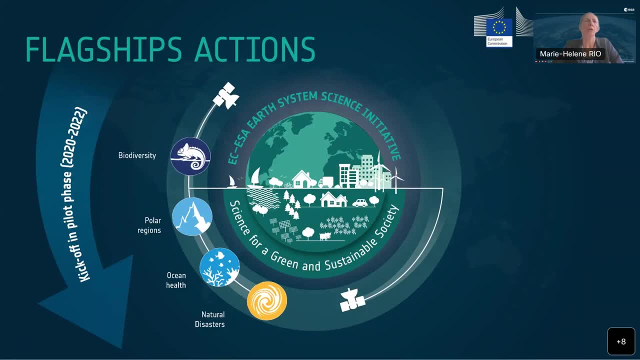 So, among these projects, an important point also is that three years ago- so in February 2020, we launched a collaborative framework between ESA and the European Commission called the ESA Earth System Science Initiative, to really start launching projects in a coordinated manner between ESA and the European Commission, and we have defined a number of priority topics. 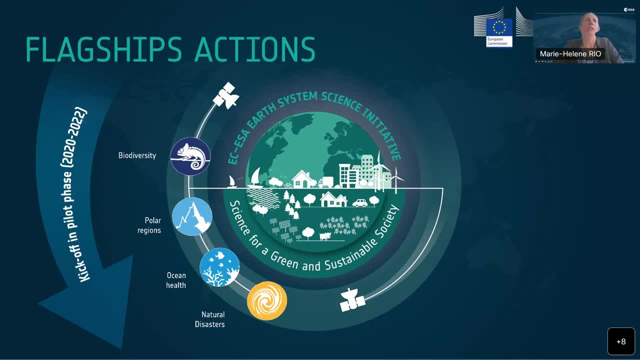 for which flagship initiatives have been created and flagship projects are being started to launch collaborative projects, And among those we have a flagship initiative on biodiversity and another one on ocean health, So both of these initiatives- of course, ocean color data are key in this. 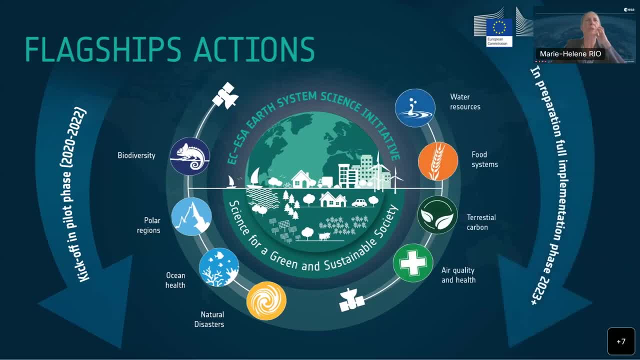 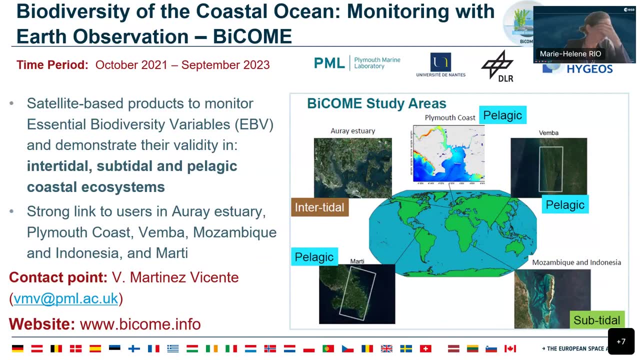 So I will go very quickly through a number of these projects. It's not exhaustive. There are different projects. There are many different projects. You can have a look at them. I was giving the link on the slide with the Ocean Science Cluster. 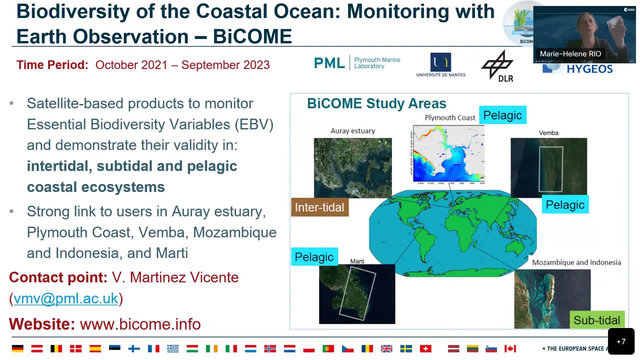 There is a link to the EO Science for Society website where you can browse for projects and find more details on the objective and the link to the project website. But very quickly so. in the Biodiversity Flagship Initiative we have a project on the coastal biodiversity. 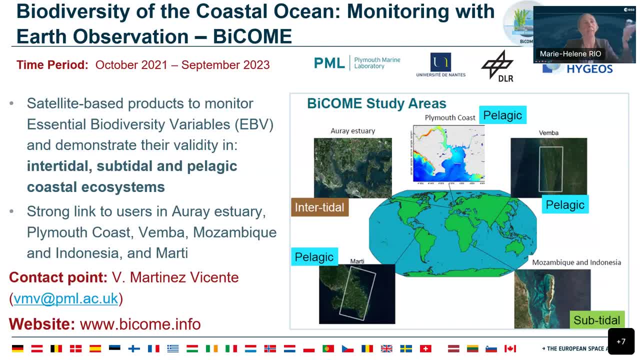 which aims at using satellite data to develop essential biodiversity variables for three different ecosystem types, so the intertidal, subtidal and pelagic coastal ecosystems. It's strongly linked with area doctors around the world to demonstrate the impact of these new products. 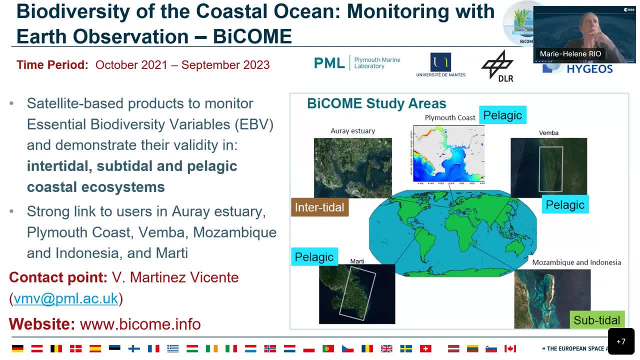 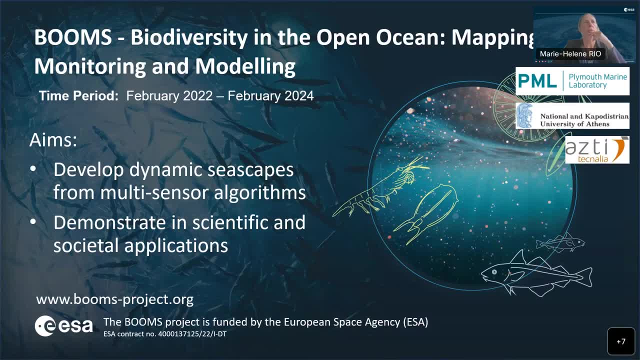 for specific use In the Biodiversity Flagship Initiative. we also have a project dedicated to open ocean biodiversity. It's called BOOMS, And the objective of this project is to develop dynamic seascapes from the use of satellite data. 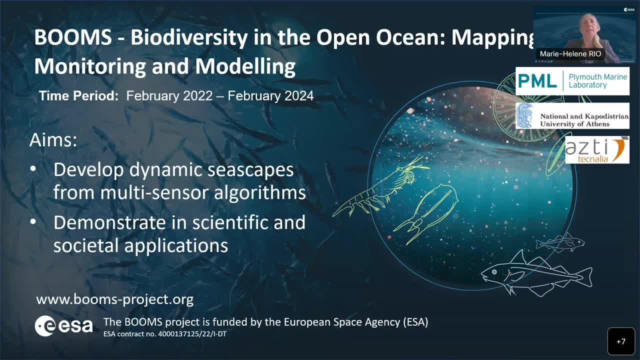 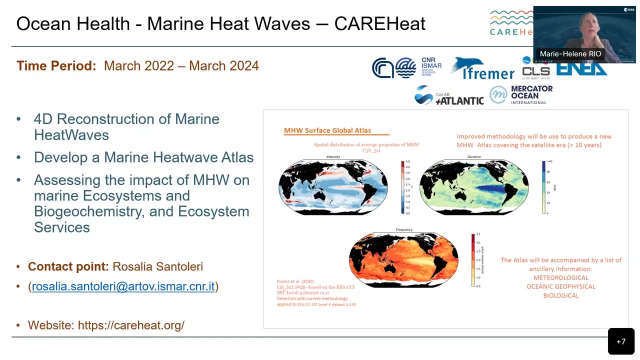 And again demonstrate how these seascapes can be used for a number of scientific investigation, for more application, like the mapping of marine protected areas into fisheries, and so on. In the Ocean Health Flagship Initiative we have launched a whole set of projects. 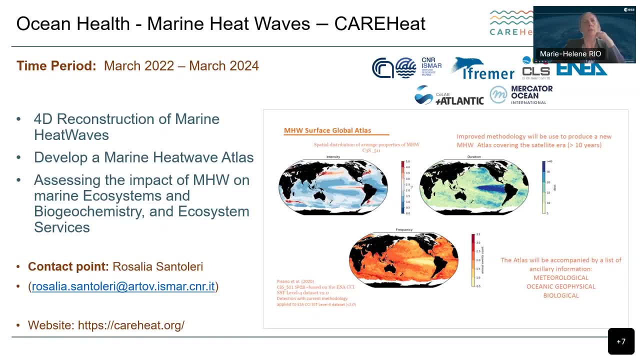 One is dedicated to marine root waves, so how we can identify and monitor marine root waves from satellite data. In this project, a marine root wave atlas is being developed, also looking at the 4D reconstruction of such events, And a number of scientific studies are being done to understand the impact of such extreme events. 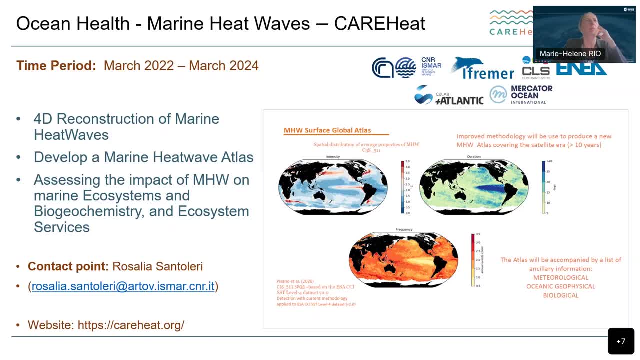 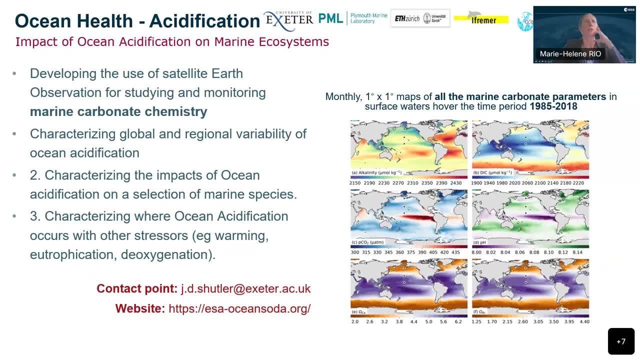 on the marine biochemistry and ecosystem. In this ocean health flagship initiative, we have a project called BOOMS. In this ocean health set of projects, we also launched a project dedicated to acidification, so how satellite data can help monitor acidification in the ocean. 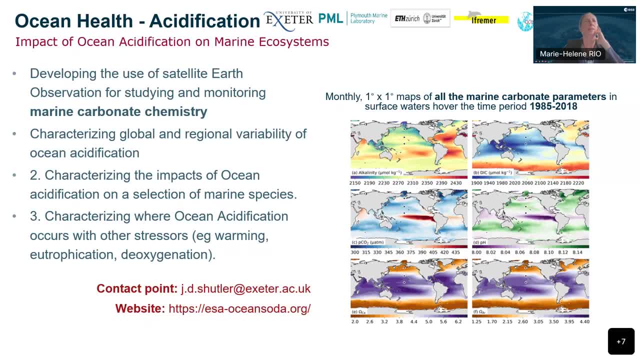 And in this project a global dataset of the different parameters of the marine carbonate system has been developed for a period starting in 1985 until today. The map I've shown here was developed in the previous project, Ocean Soda, And in the ongoing project the team is working on improving the spatial and temporal resolution. 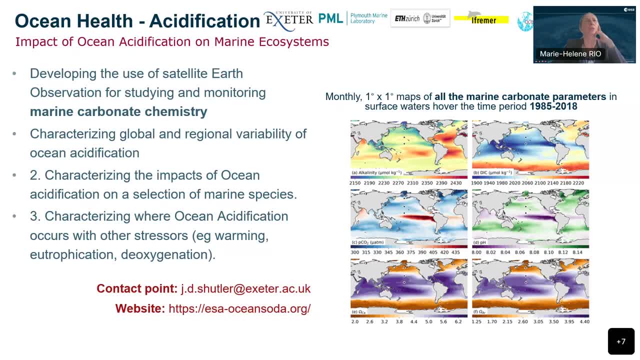 of this data going eight days and a quarter of a year, And here again, one objective is not only to develop these new products over a long time period, but also then to understand how acidification, in that case, is impacting marine species, marine ecosystem. 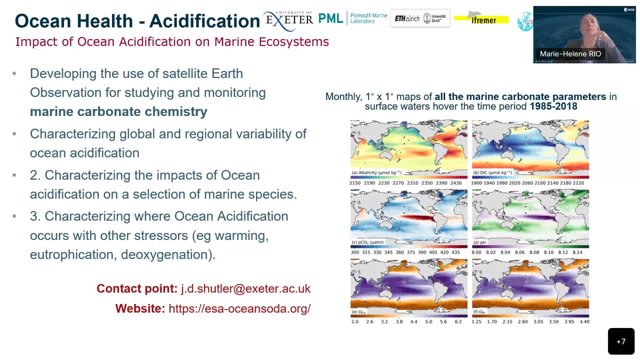 and also characterize how these ocean acidification events impact the ecosystem when they co-occur with other stressors such as warming, ossification or deoxygenation. The mapping of marine carbonate parameters is very important in the frame of ocean health. 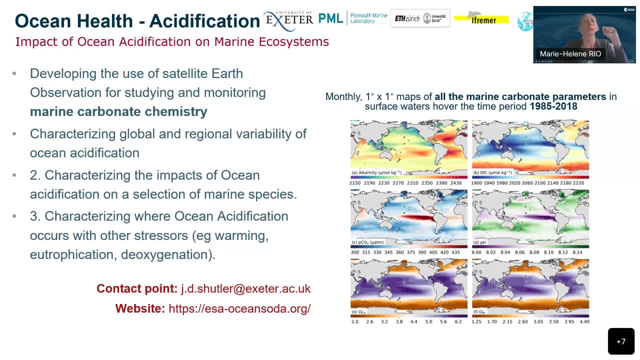 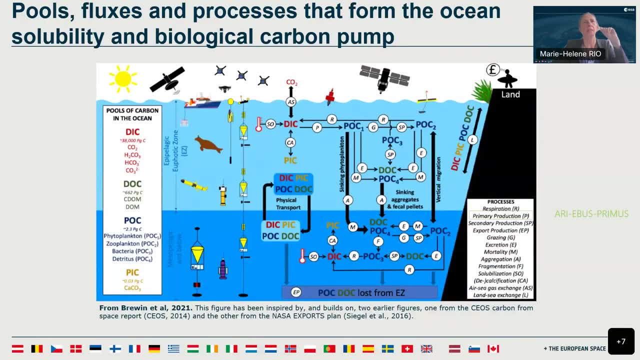 But also in the frame of better understanding the ocean carbon cycle, And there we have a number of projects. We have had a number of projects tackling the different components of the ocean carbon cycle. So here I took a number of projects that you can see. 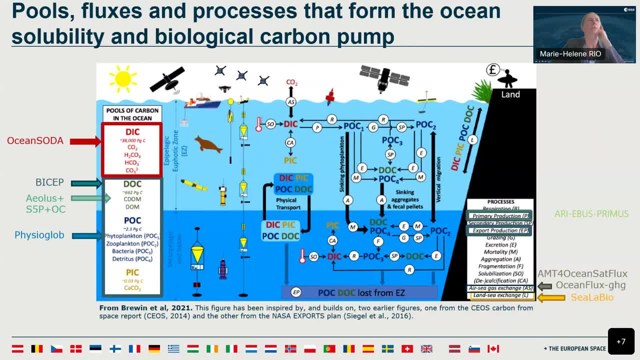 I've been tackling the different groups of carbon in the ocean, but also a number of processes as primary production, export production and the exchanges at the interface between air, sea and land and sea. This nice schematic that you already saw in Thomas' presentation. 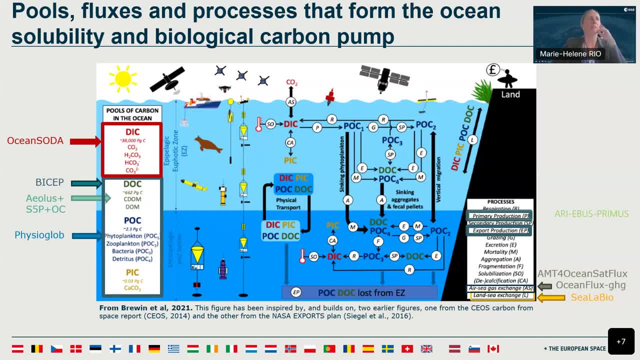 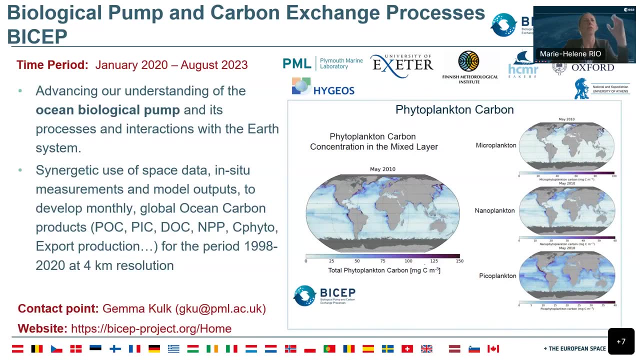 was done in the frame of the BICEP project. It's one of these projects Which was dedicated- still running, actually dedicated- to the biological carbon pump And so the estimation from satellite data of the different groups of carbon in the ocean. 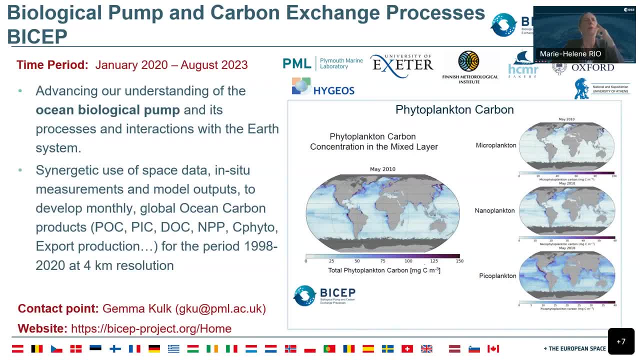 So the project is coming to an end at the end of summer. It has developed a data set from the ITI 2020 at four kilometer resolution, monthly global of different products: Particulate organic carbon. inorganic carbon. dissolved organic carbon. 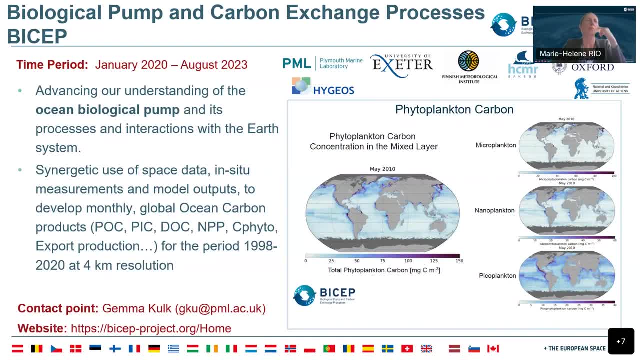 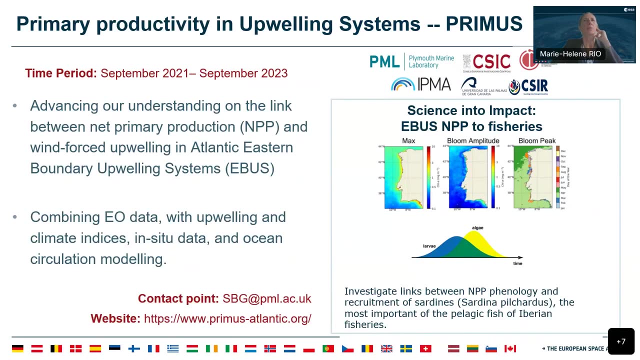 net primary production, phytoplankton carbon export production and so on. So all of these data sets are available. You can go on the site, on the project website, and you can have a look at them. Another project which is still running is looking at net primary production. 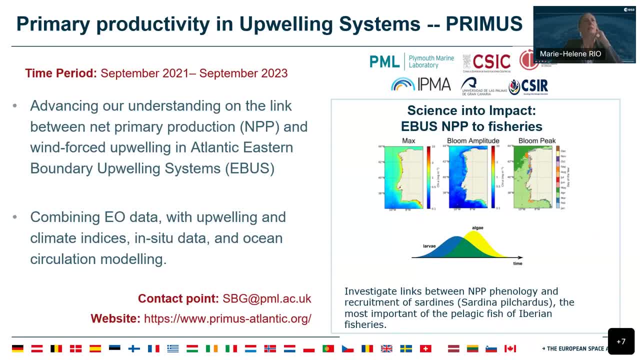 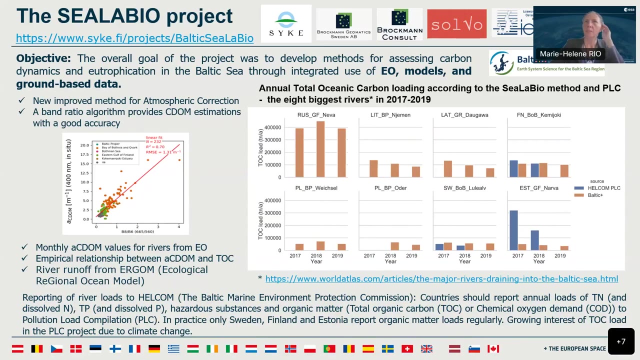 in a specific case of a cooling system, To advance our understanding on the link between net primary production and wind force operating, Combining satellites with in-situ data, ocean circulation modeling and climate indices To look at what happens at the interface. we also had a project. 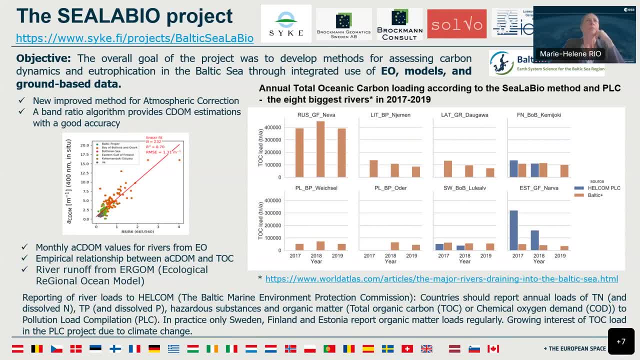 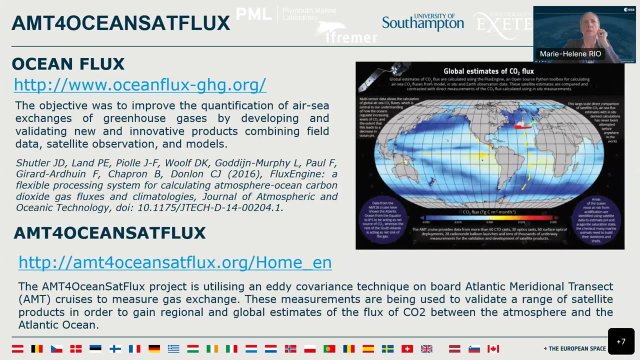 the CILABU in the Baltic Sea, And its objective was to develop methods for assessing carbon dynamics and stratification in this specific area of the world And also calculate total oceanic carbon load from the eight biggest rivers of the Baltic area. We also have had in the past and still running some projects looking at the fluxes. 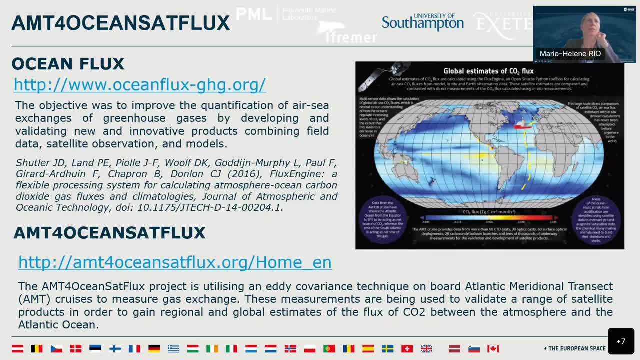 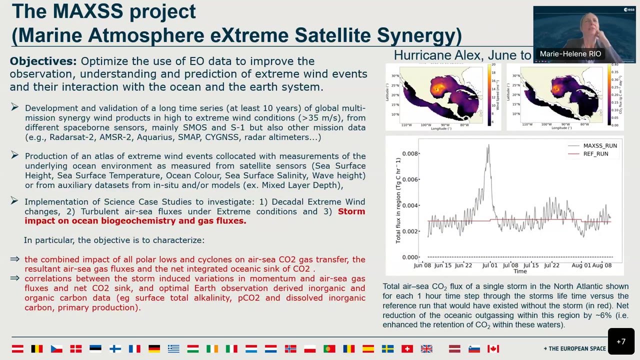 So the ocean flux was dedicated to quantify air-sea exchanges of greenhouse gases And we also have this AMT for Oceansat, first project With an instrument on board the Atlantic Maritime Transit Cruises to measure gas exchange. We also have coming to an end a project looking at extreme wind events. 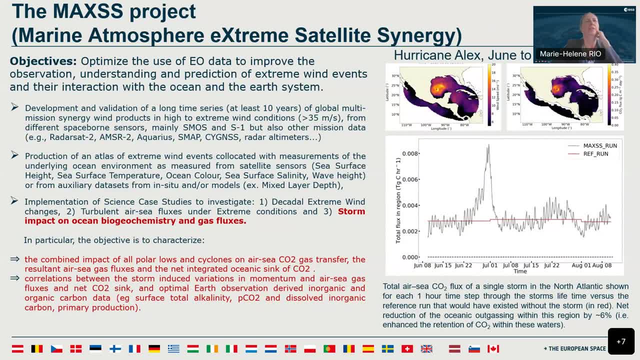 And I mention it here because we had an interesting case study linked to the ocean carbon. So in this project a new data set of winds was developed using many different instruments that we have in Synergy that provide information about winds, So a radiometer, a scathevometer and a SAR. 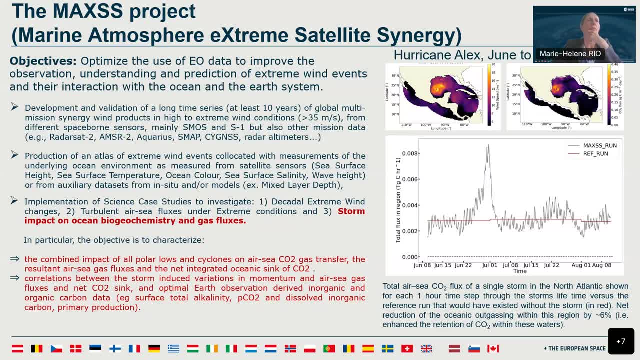 And an atlas of extreme wind events was developed, collocated with measurements of the underlying weather conditions, And we also have a project looking at the ocean environments which time we had a storm. So the tropical cyclone, the polar lobes, the hurricanes. 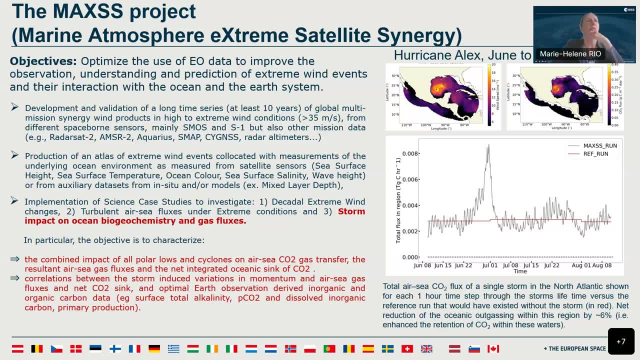 The project has been looking at what happened at the ocean, at the surface of the ocean, in terms of temperature, color, salinity and so on, And the specific work has been done to understand the impact on the gas exchange and CO2 fluxes. 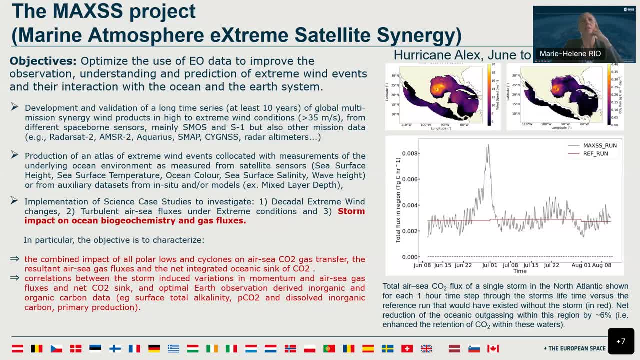 And this is an example- This is in 2010.. And this was found in the specific case that the storm induced a net reduction of oceanic outgazing by around 6%, And so the idea now is to upscale this study on a single case to the ensemble. 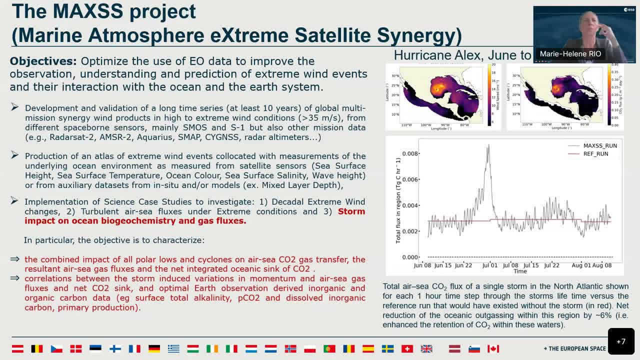 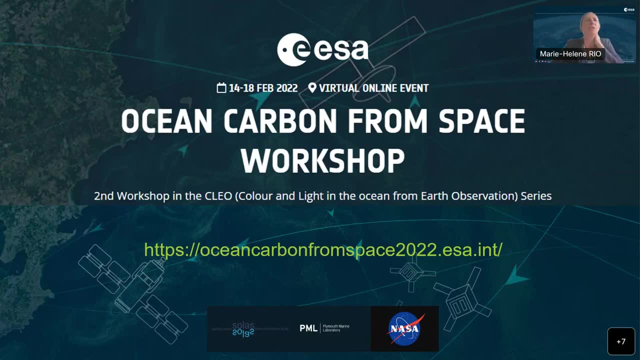 of tropical cyclones and storms that we have in the atlas to have a global view of a long-time period of the impact of such extreme events on Earth's sea and sea-level fluxes. So all these projects. on ocean carbon, We had a very interesting ocean carbon from space workshop last year in February. 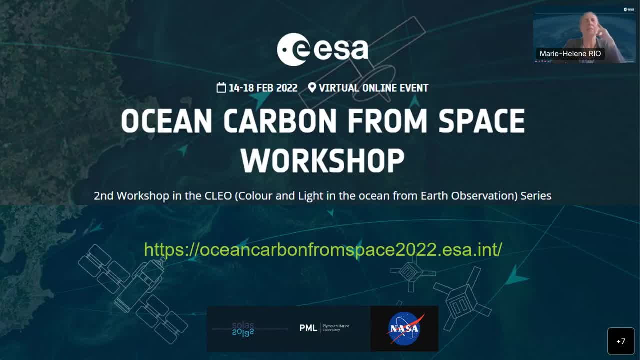 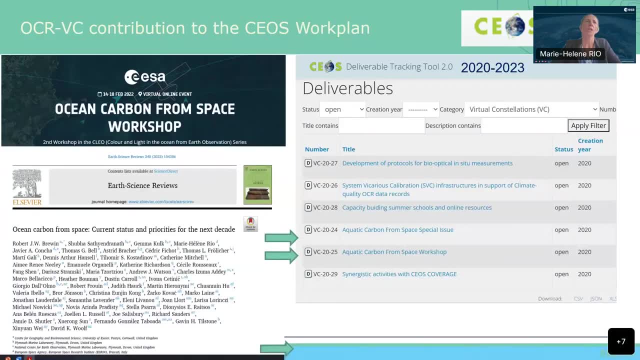 where all these projects were presented, and many others. This was an international workshop very successful, out of which a number of recommendations arrived on the current status and priorities for the next decade to further understand the ocean carbon cycle and how we monitor it from space. 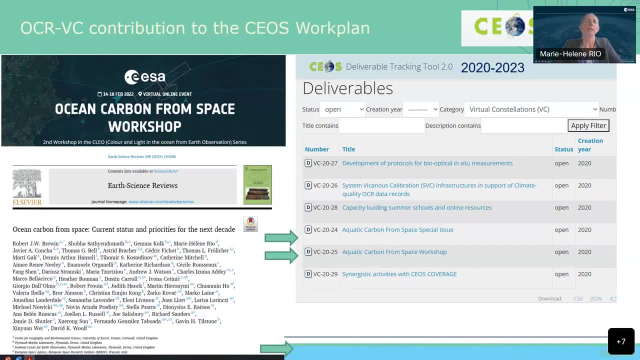 And this recommendation and this white paper that was issued out of it was actually also one of so the workshop and the paper was well, actually deliverables from the CEOS. so Committee on Earth Observation Satellites, which is, of course, ESA, is one member on this committee. 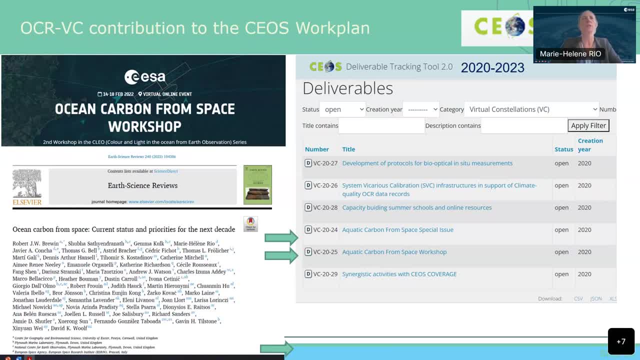 And together with other space agencies in the world, we are trying to cooperate to make the best out of satellite data for us observation, And we have dedicated topics on ocean and aquatic carbon. So the workshop and the white paper were part of the work plans for 2023. 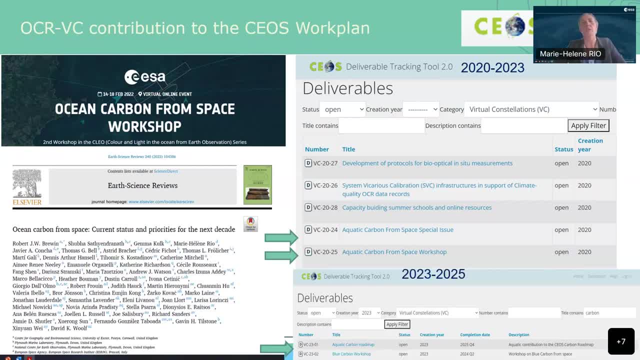 And for the next work plan. so in the next three years. we have included other deliverables So we plan to contribute or to develop an aquatic carbon network roadmap in these three years And also we have planned a blue carbon workshop that will take place next year. 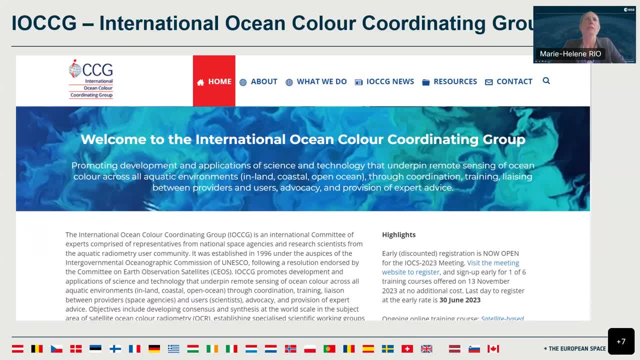 I also would like to mention that ESA is part of the International Ocean Color Coordinating Group, which is an international committee of experts comprising representatives from the National Space Agencies and research scientists of the Aquatic Radiometry Reserve Community. The objective of the IUCCG is to promote the development and application. 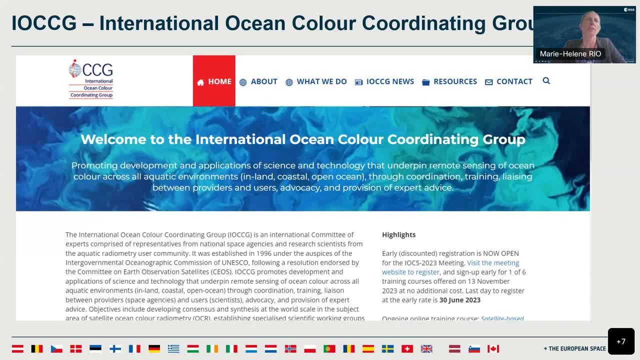 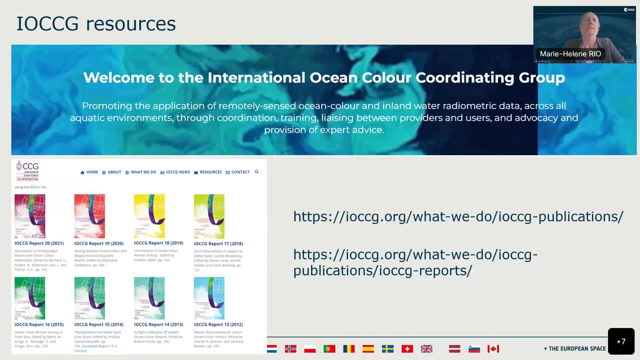 of science and technology on the cleaning or absencing of ocean color across all aquatic environments, so not only ocean but coastal and also inland. So through coordination, training and so on, And in that context I think it is going to be very useful. 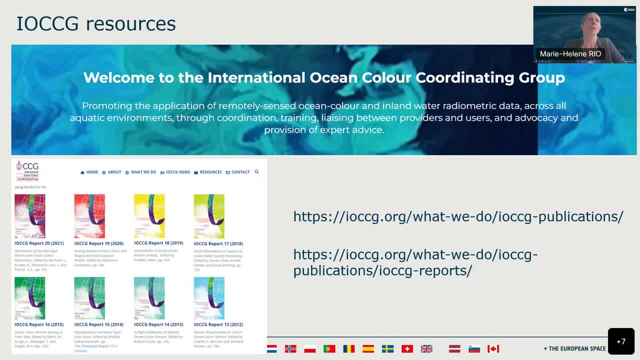 for everyone who wants to know more about ocean color, ocean color radiometry, to have a look at the resource pages- resources pages of the IUCCG, where you can find a number of publications and reports which are very, very, very useful to further understand. 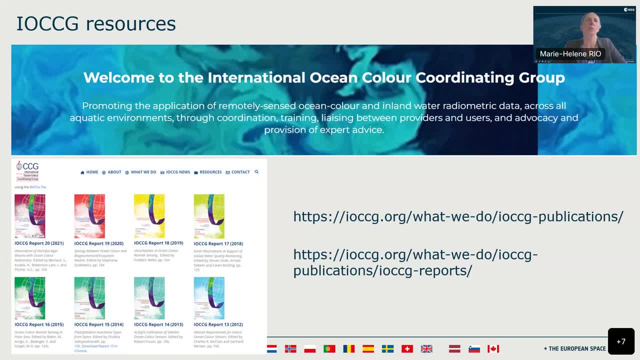 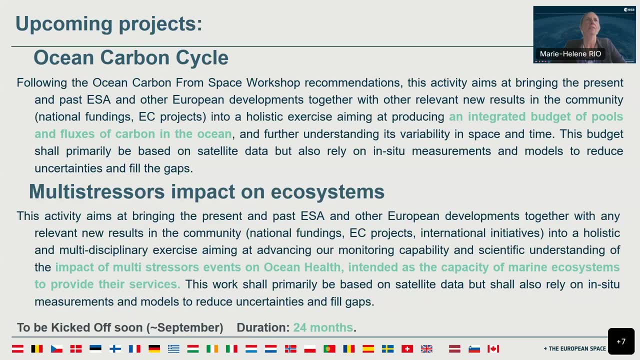 what can be done with ocean color radiometry. Finally, we have a number of projects upcoming In the pipeline. we have two projects that should be kicked off very soon, I guess after summer. One following the Ocean Carbon from Space workshop recommendation. 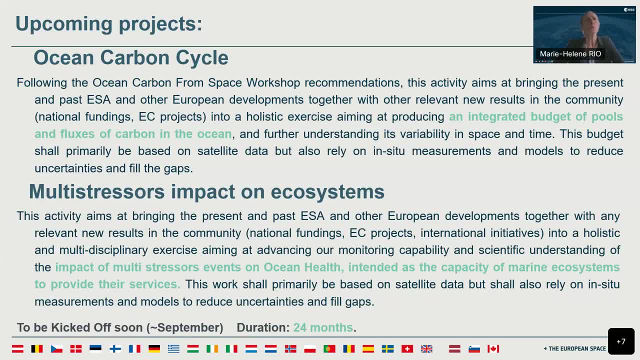 we have launched a new project on ocean carbon cycle, with the objective to produce an integrated budget of flows and fluxes of carbon in the ocean, so primarily based on satellite data and also, of course, related in situ and models, to reduce uncertainty and fill the gaps. 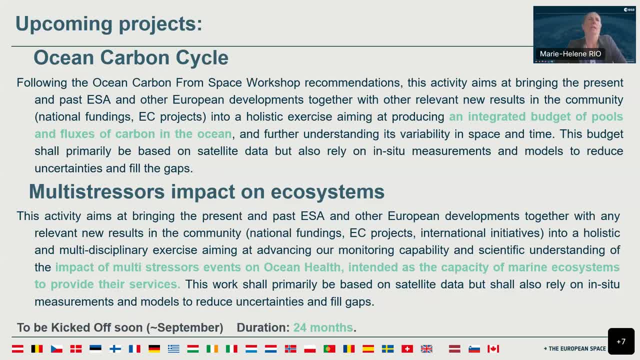 And we also have another project that will advance our scientific understanding on the impact of multi-stressor events on ocean health, intended as a capacity of marine ecosystems to provide their services. So these two projects will last two years, and so they'll be starting very soon. 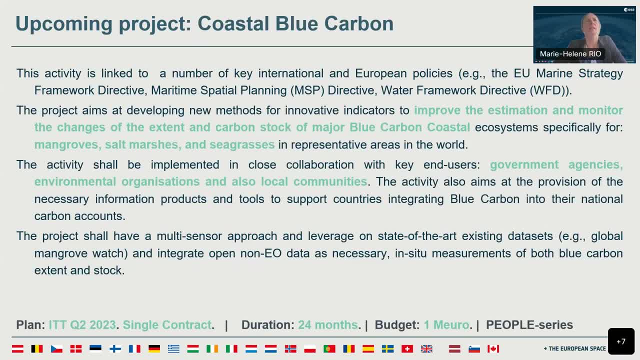 And finally, we have a project which is still sort of to come- We are opening the call in the next weeks actually- and this will target coastal blue carbon. So this project, the objective will be to develop new methods to develop and to further to improve the estimation of carbon stocks from remote sensing data. 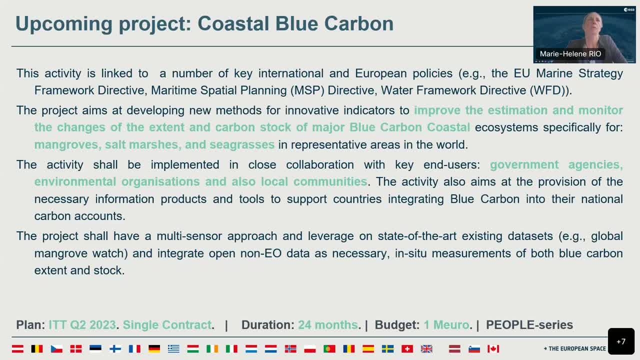 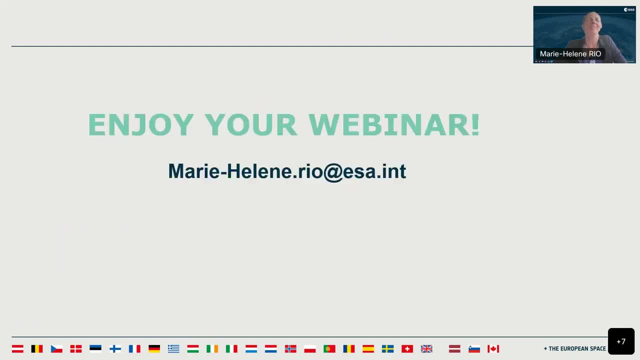 for major blue carbon coastal ecosystems, So in particular, mangroves, salt marshes and sea grasses. And I think I'm already running out of time. I wish you a very successful, fruitful webinar. Again, here is my email. 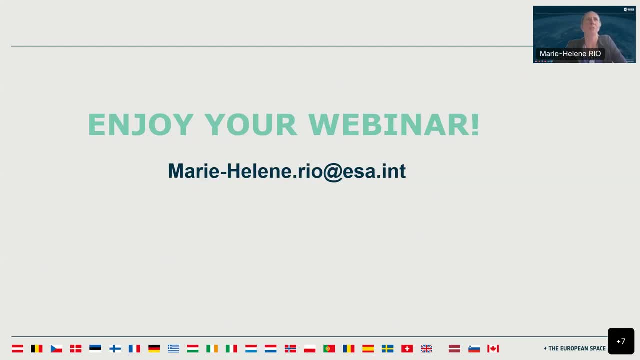 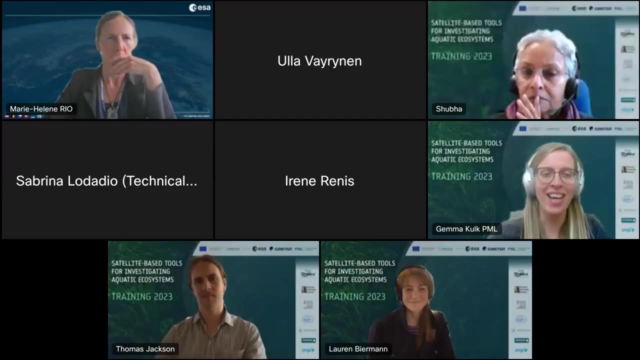 You are very welcome to contact me for any question to get further information on our program and projects. Thank you very much. Thank you, Marie-Helene. That was a really good overview of all of the activities from the ESA side And, clearly, the topic of climate and ocean ecosystems. 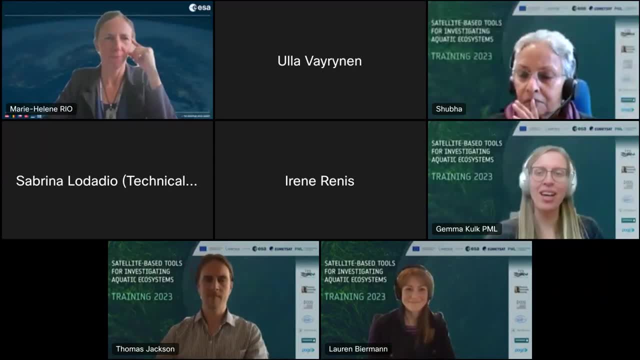 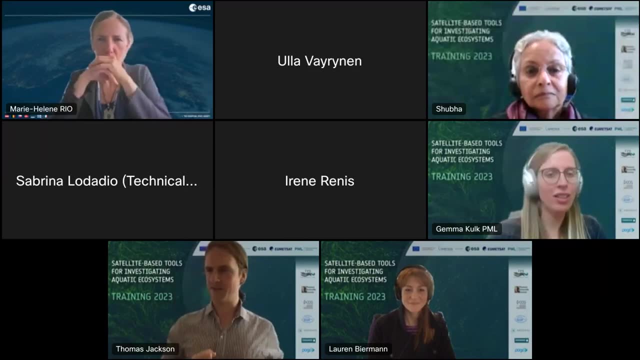 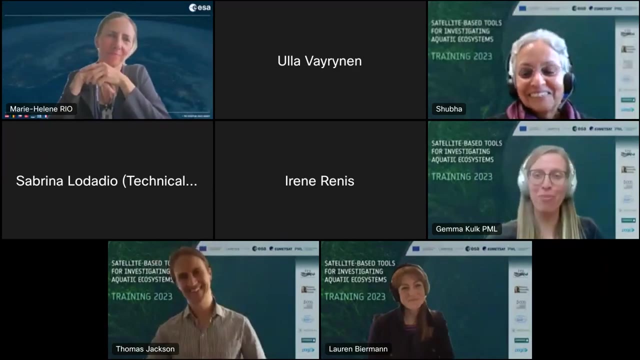 is very important to ESA. I'm going to continue on with the Q&A session. I'm expecting good questions after my thing about Good questions- Excellent, I hope so. We'll do our best. We have a bunch of questions, So I just wanted to tick off the logistical ones first. 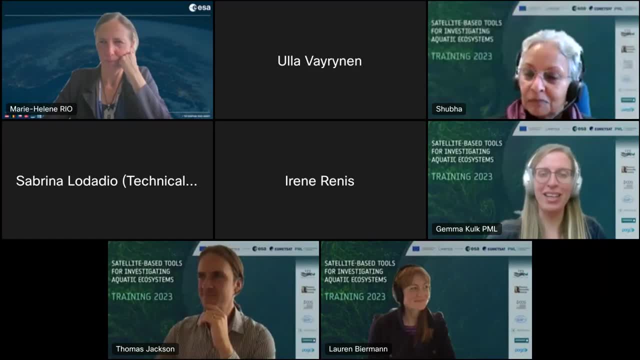 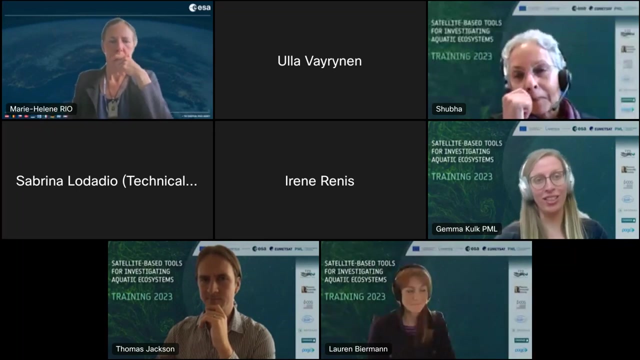 So there was a question about whether the PowerPoint presentations were going to be available. I think the answer is no. The recordings of the presentations and the slides that are presented are available on our YouTube channel, So you can check that out. And then there was a question on where to access the OCCCI data. 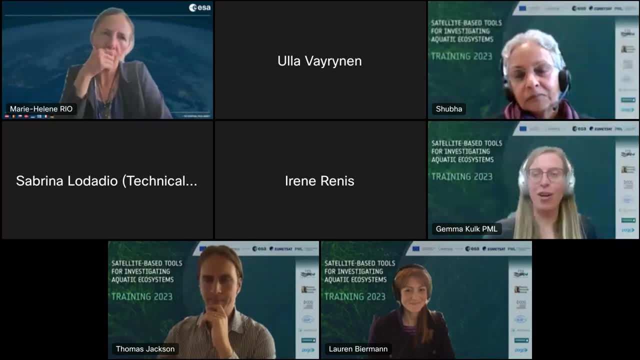 So in the first instance you would go to the ESA CCI open data portal And I'm just going to put the link in the chat again. So if you download your data there, ESA actually has a good idea of who's using the data. 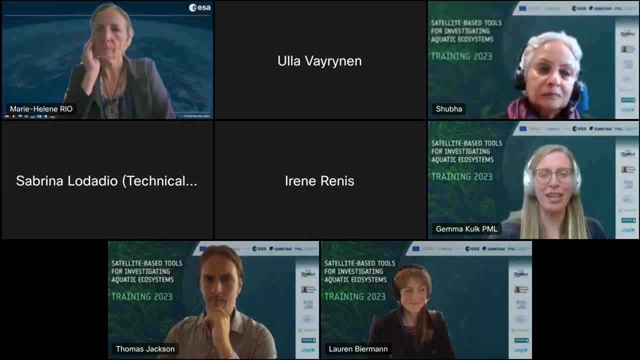 when and why and what for. So it gives their information about the data usage, which is also good for the developers of the data. And then a comment from Lauren that please be careful with downloading the data If you do global products for 20 years. 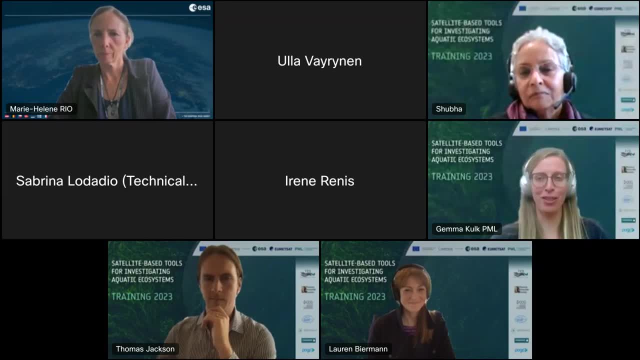 that's a massive amount of data, So start small bits of data download. It will make it easier for you to download all the data. If you go to the CCI, if you just Google OCCCI ESA, if you go to the documents section of their page. 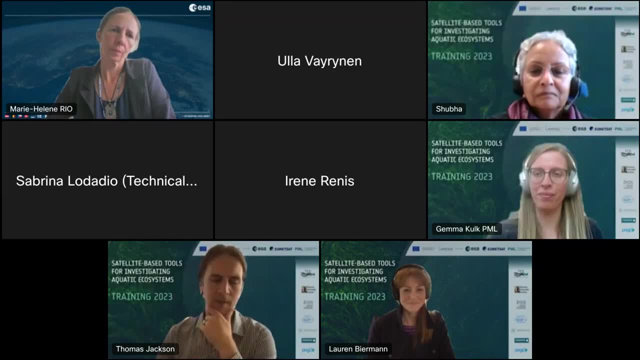 which I think is linked in my references in the product user guide. there's also some helpful hints on how to extract little bits of data using basic code and things like that, So you don't need to download terabytes of data if you're only interested in a small region. 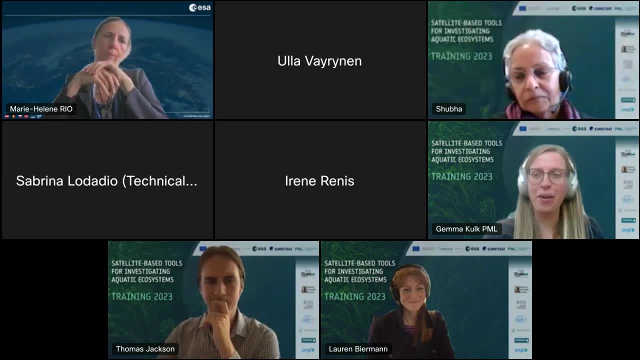 A very good point, TJ. So there are a couple of questions about ocean color indicators. So you mentioned two ECVs related to ocean color, which was chlorophyll A and the reflectances, And the question was whether that's sufficient information. 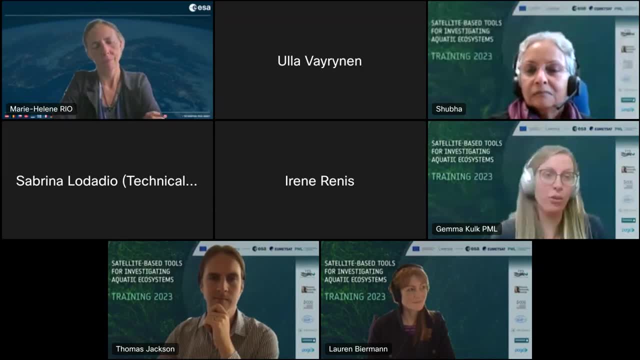 to determine the impact of climate change on the phytoplankton community, whether globally or in a specific location. I think that's a mixed question, Fundamentally not everywhere. no, I mean, as we saw, the record has to be longer than we've got now. 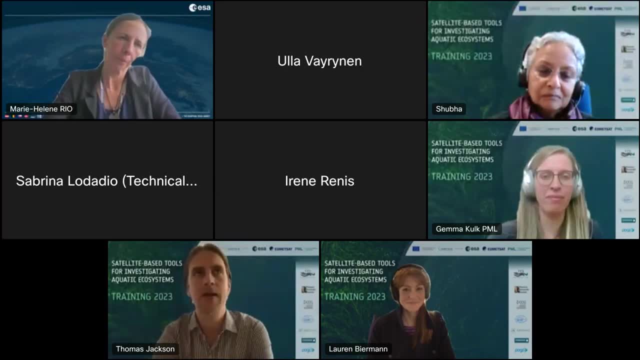 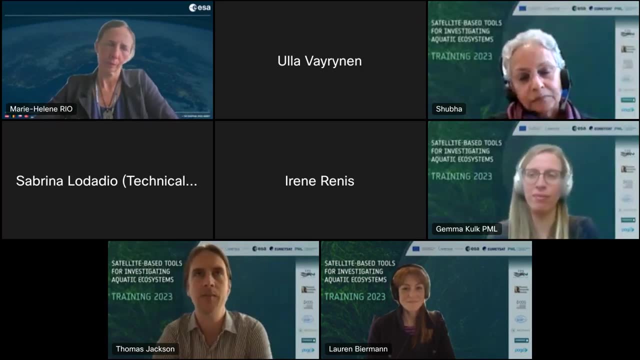 In terms of the actual indicators themselves, this comes back to what constitutes a fundamental record, so a climate data record. which are those? So the reflectances measured, calculated from the radiances, are the most fundamental variable, And then from there we can derive other indicators. 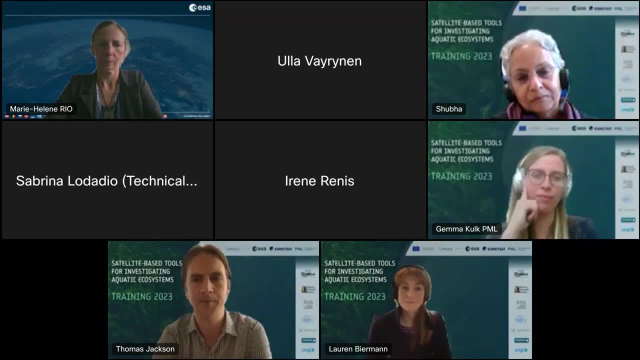 But those other indicators might not be classed as essential or fundamental records, but they are still useful climate indicators. So, yeah, I think that the breadth that we can go to of indicators from ocean color is very big, but the definition of the ECB and the CDR. 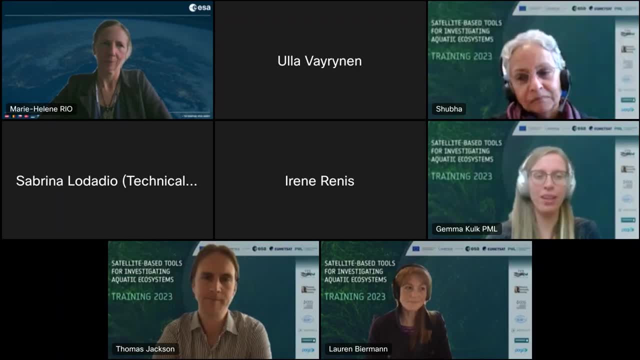 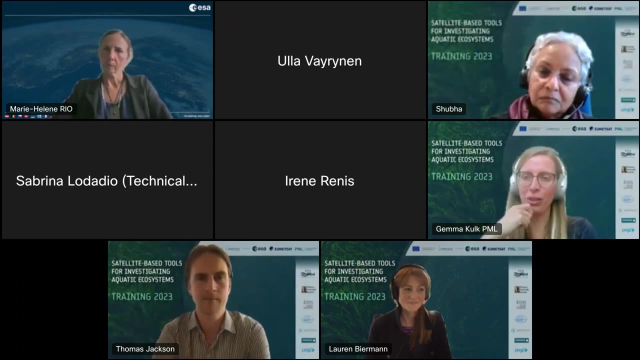 is quite tightly constrained. Thank you, TJ. A question also related to the ocean color data record, and I think Lauren mentioned that you've already touched upon this. but is ocean color really changing or are we just assuming it will change Because of the physical drivers? 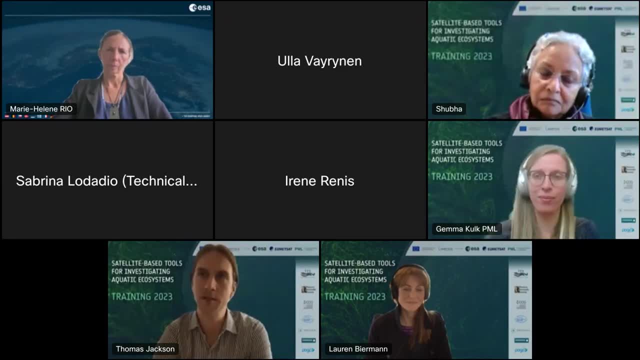 So I think, from what you see, from the two short studies I showed- I mean, as I said, there's been hundreds of publications using this data, but the two examples I showed, both of those were driven by- Well, the Barents Sea was driven by an observed change. 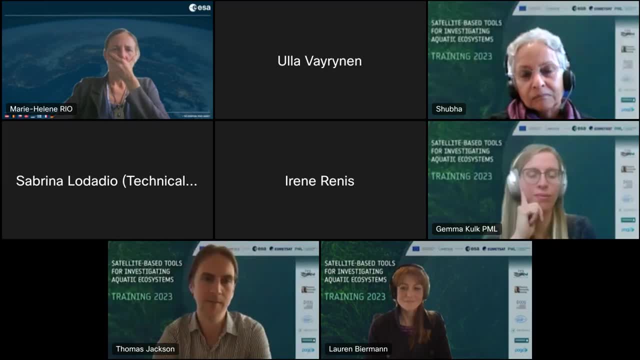 So they saw there was an increase in autumn blues. That is a change, The reason that people started. You know you might say I'm going to go and look at the Arctic and you expect there to be a change, but the change was found. 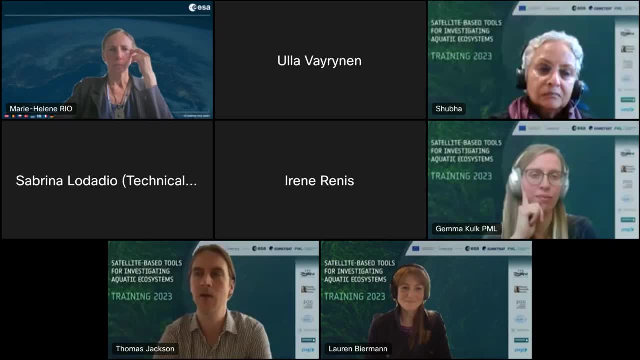 And in terms of the changes in hue angle or Secchi depth, again, that's observed. So, yes, we are seeing some shifts, The bit that's difficult or we don't have, let's say, a big red flag to wave. 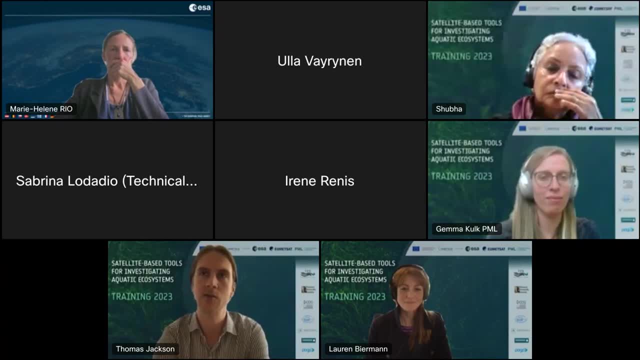 is. you know, if you look at things like sea surface temperature or atmospheric temperatures, you know those are increasing globally. You take the big global average and it's going up. We're not seeing that in the ocean colour or chlorophyll record. because it's a much more complex system. It's not just physics. Biology is messy And it's really in the detail. So what's increasing, what's decreasing, what's staying the same, but the community is changing. All of that has massive impacts. 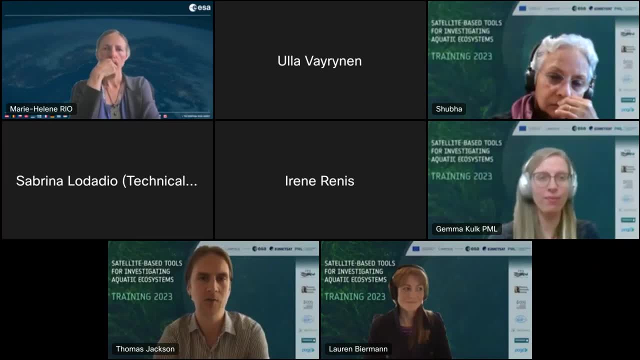 But it's not a uniform story across the globe, And that's a really good point to make. Thank you, TJ. Another question is whether ocean colour can be applied to assess climate change in coastal ecosystems, including estuaries, for example. 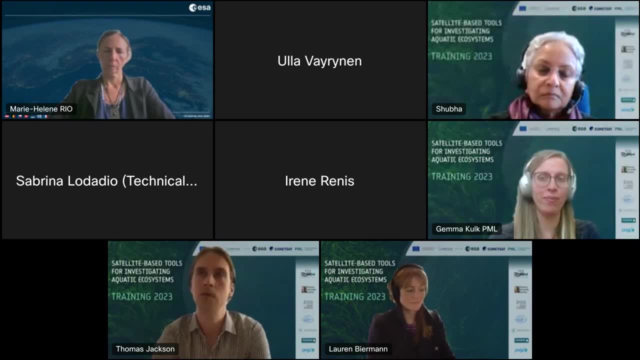 So the OCCCI records focused originally on the deep oceans. In the last two cycles they've been pushing to try and do better in coastal waters. So that's part of the justification behind the algorithm blending. It means that in more complex waters 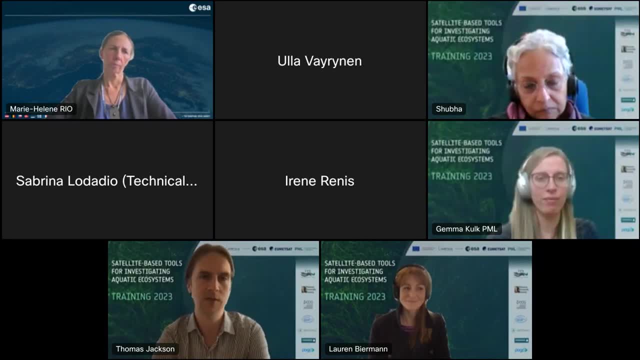 we can use algorithms that are tailored for those environments. Once you push really up into estuarine waters or into river mouths, that's going to start being less reliable. But that said, there are ongoing projects such as CHIRTO and others that have links to the CCI projects. 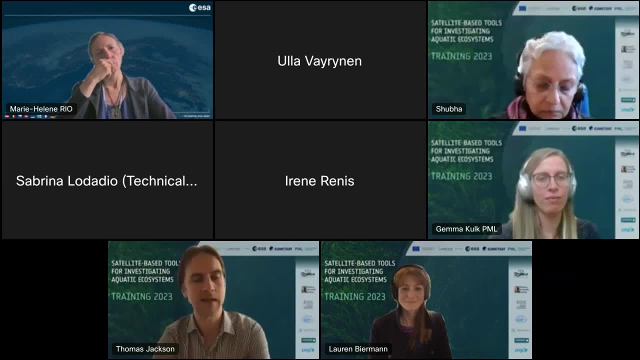 that are looking to basically use similar techniques but develop them into really coastal waters and inland waters And then we might see over the next years those feedbacks, those upgrades, coming back into CCI. So for now, in really, really estuarine. 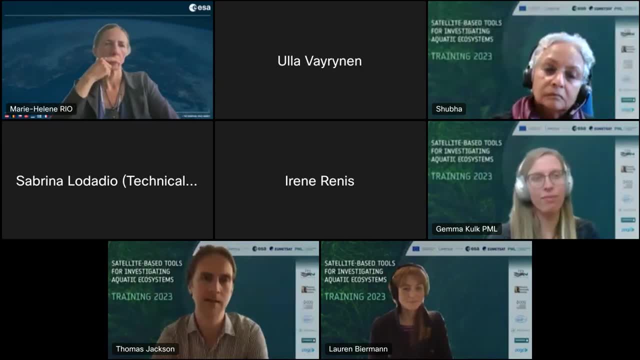 within deltas and things like that I wouldn't trust necessarily the data, But in near coastal and coastal areas there's been a lot of work in the last couple of years to try and make that data more reliable. Thank you, TJ, And I can also just add, if it's okay: 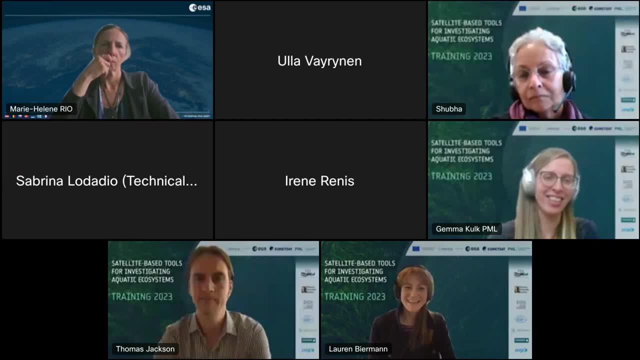 I'm sorry that. obviously, Of course, Lauren. On the ESA data page you can see all of the different CCIs. So it's not just the ocean colour CCI that's there, There's the lakes CCI as well. 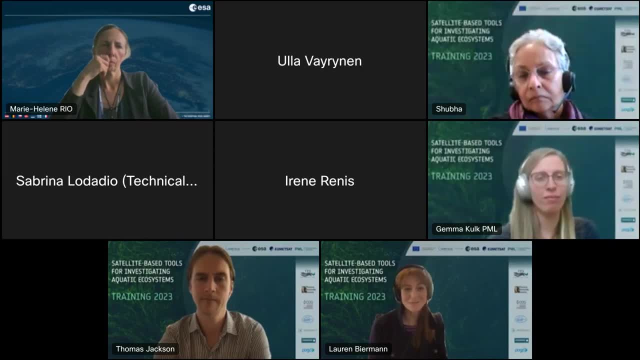 So I know that's not estuaries necessarily, but it is inland waters and that's something to be aware of as well. So all the CCIs there for you to look at, And because one of the requirements for a climate record is that it has uncertainties per pixel. 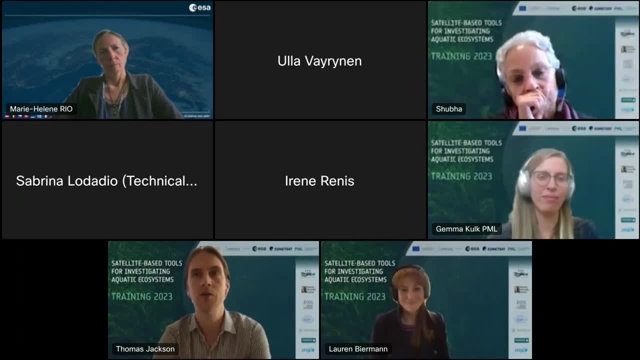 associated with the data. you can use the uncertainty in the variables to look at your confidence intervals on any results you've got. So where we know we don't do very well, we tell you we know we don't do very well. So 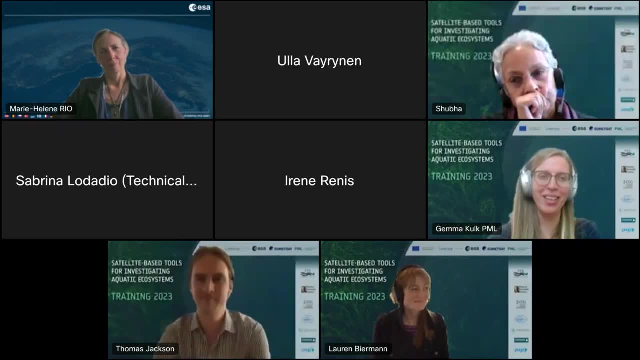 Thank you, TJ. That's an important point. I think it's important to look at the data as well, so users can make an informed decision about the data they use. A question actually from our side: Why did you pick MERIS as your reference sensor? 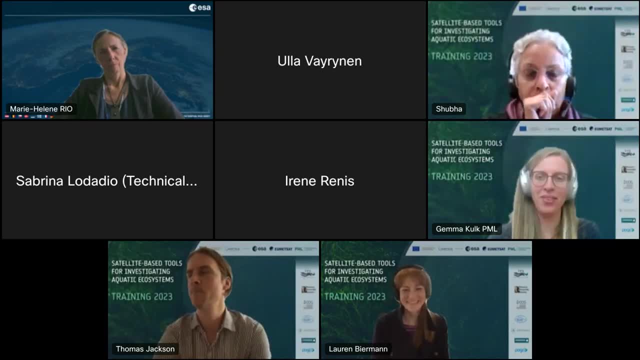 in the OC CCI time series. Okay, In the first four versions of the CCI datasets, CEWIS was the reference And that was because it was a sensor that was well known, well understood. There was a lot of studies done on it. 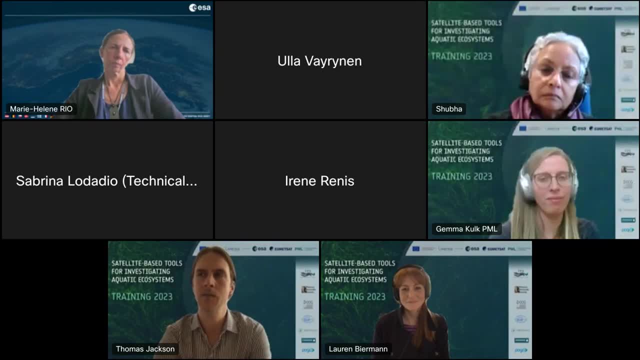 Then the goal longer term, because the ALCI's have that unique property of being effectively the same sensor across AB and what will be C and D. we would envisage that ALCI will become the reference record, So MERIS, because it has the same wavelengths. 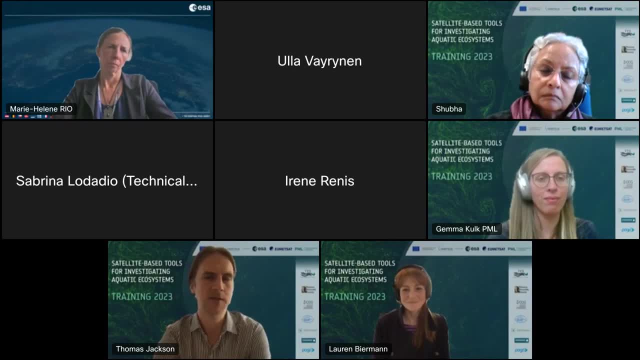 as ALCI and is an ALCI-like sensor, was basically an interim reference. So we switched to MERIS as the reference and we will switch eventually to ALCI as the reference. But MERIS was a kind of halfway between the two. 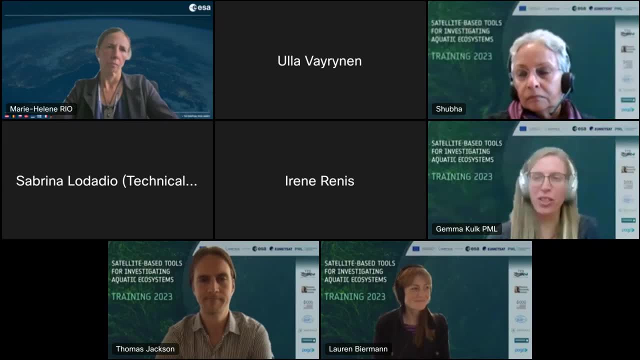 Thank you, TJ. There's a question related to this, and that is: why is the design of the OC sensors different? Are these related to improvements over time in the sensors? I think largely yes, So there is a push for increased resolution. 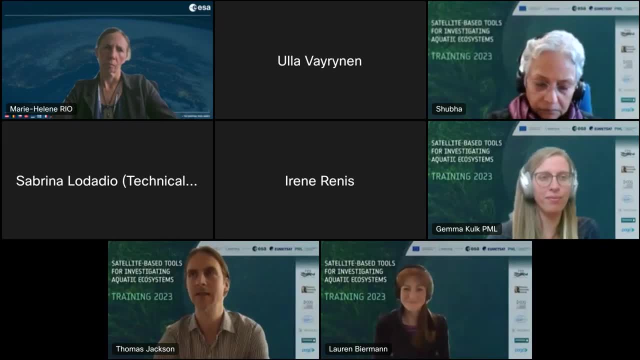 both spatial, spectral and these sorts of things, I mean the fundamental bands that we know are important for ocean colour. you know, if you could only pick six or if you could only pick eight. a lot of that was laid down in the work. 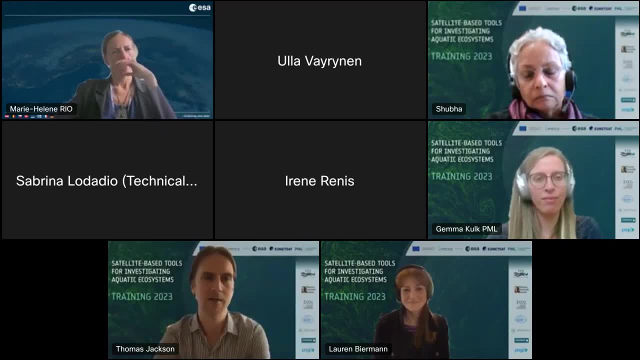 by the IACCG, Schuber and others laid that out very clearly. So, basically, as we've been able to capture and record more data, we've added bands to the primary set, But as to why, you know, VIIRS doesn't have some of these bands. 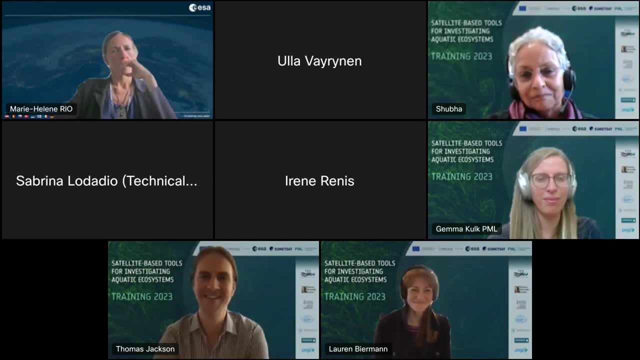 I'm not going to speculate on the other space agencies' priorities, But yes, it can be frustrating when that changes. Thank you. There's another question related to the CCI data set. You mentioned that you do your band shifting process by using a forward model. 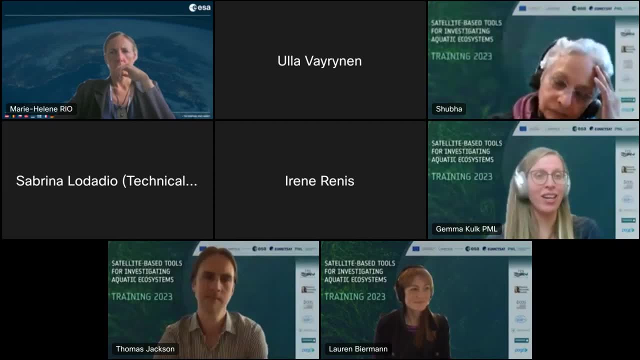 And so the question is related to that. So, in essence, you would have a hyperspectral data set. Is it then easier to merge the hyperspectral satellite data with that of OCCCI data? So I guess that's imagining if we had PACE. 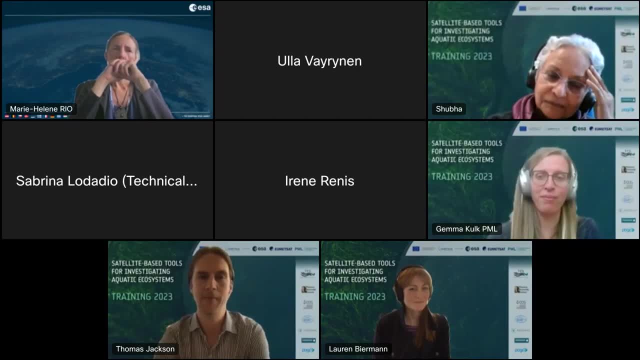 or something like that. Yeah, in some ways we wouldn't have to band shift PACE, We would just pick the wavelengths that we wanted. We would still definitely have to do a bias correction, because even if you're looking at the same wavelength- 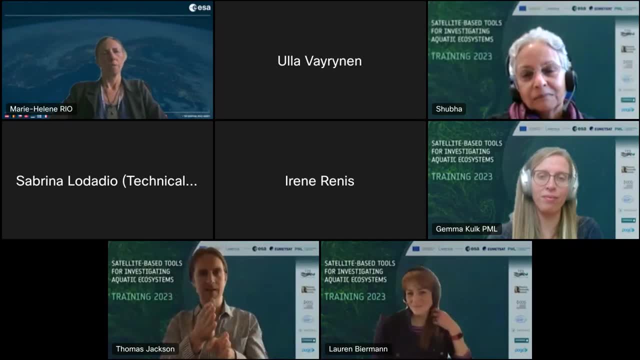 if you picked 510 or 443 nanometers. the response function of different sensors is different. The viewing angles will be different, So there will still be some need for an intersensor bias correction, but the band shifting itself wouldn't be required. 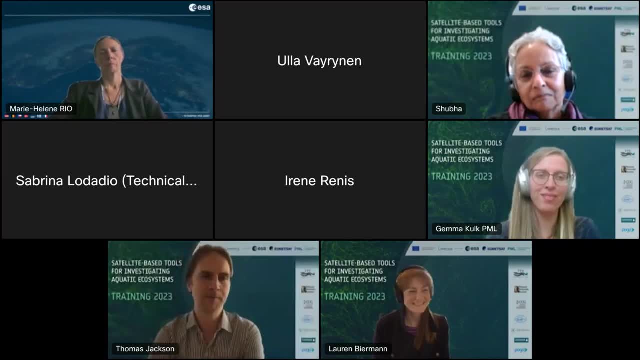 Yeah, so that's something to look forward to with PACE. I mean we could, if you imagine going, if data volumes were no problem and we wanted to, you could effectively provide a synthetic- you know- sensor from that forward model. 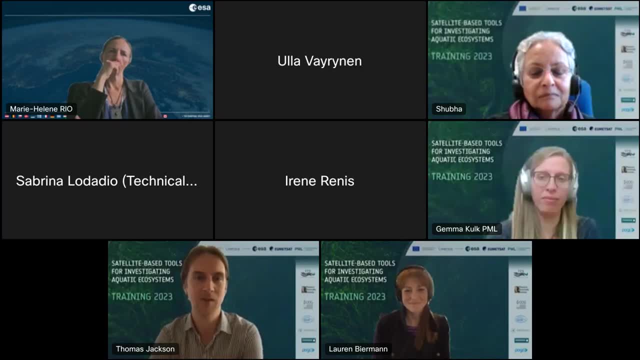 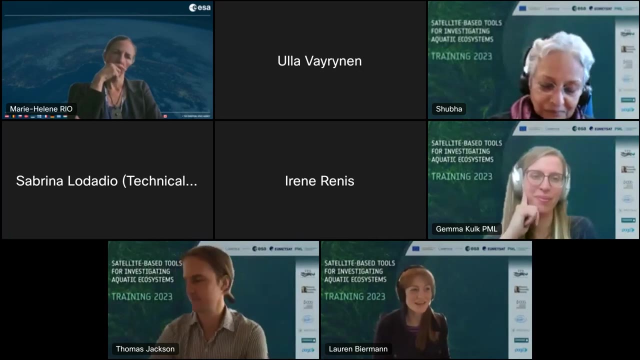 from all the sensors, But that would require bias correcting all those wavelengths, which is a lot to do. Yeah, Thank you, Go ahead. Yeah, If I can just add a little bit to that. Okay, So I think there's a lot of excitement. 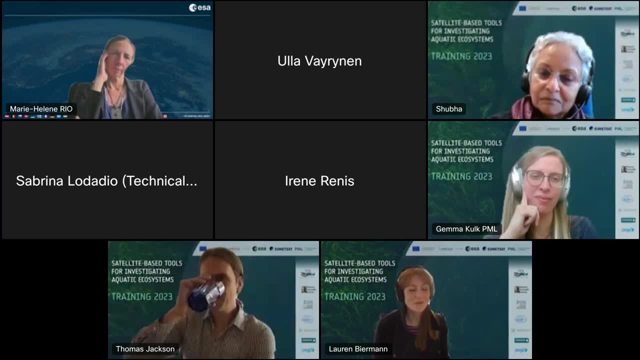 about the hyperspectral emissions for very good reason, But of course, as TJ has shown, you know, one of the benefits of using the multispectral sensors that we've been using is that we've studied them extensively since the 70s and 80s, right. 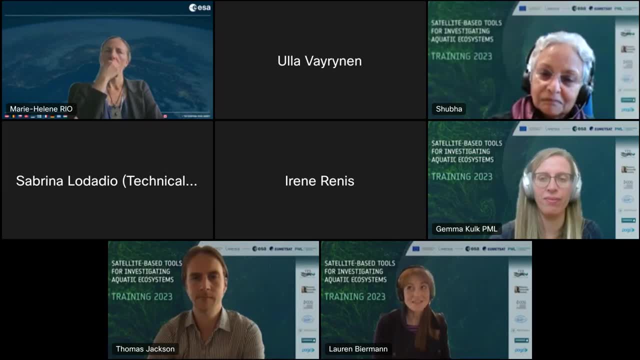 The new emissions. as much as it is very exciting, the data are new and they are. I mean. and Candice's question is: do new issues arise? Yes, they do. It's a new sensor. It has its own limitations. 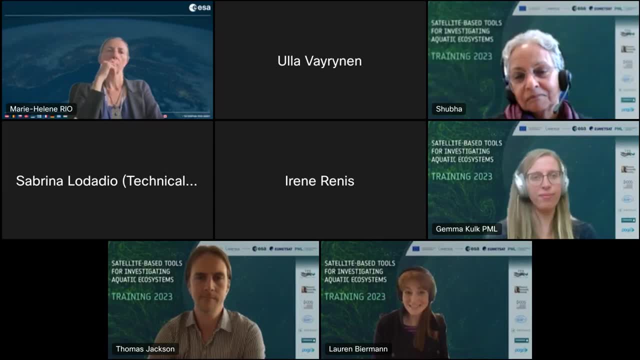 We're finding that some of the bands that are key are quite noisy when they shouldn't be, And so it's not again the silver bullet that will solve ocean colour. There is no such thing as the perfect instrument. It is very exciting. 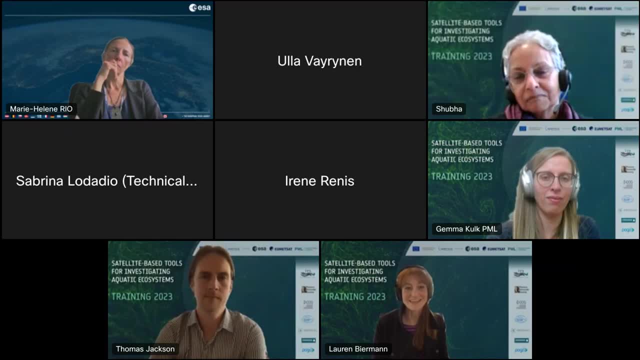 but it's going to come with time and study to get to a point where we can be as confident as we are for sensors like Olchi, for example, And those that, let's say, the properties of each sensor have to be monitored through the lifetime as well. 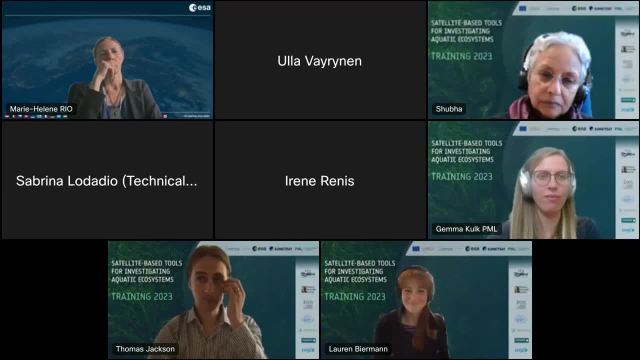 So in that plot I had, where I showed the pre and post band shifting, you may have noticed that the VIIRS record you know is terminated before now, even though VIIRS is still running. Well, that's VIIRS on SNPP. 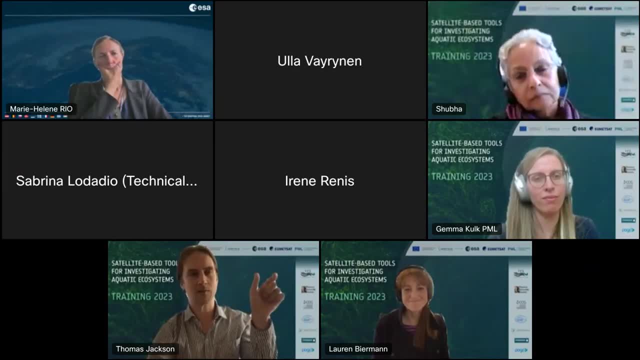 And that's because we saw that some of the bands were dropping where others weren't, and it was disagreeing with other sensors And there was this odd, you know, shift in the last few years. So we basically made a call that we couldn't guarantee. 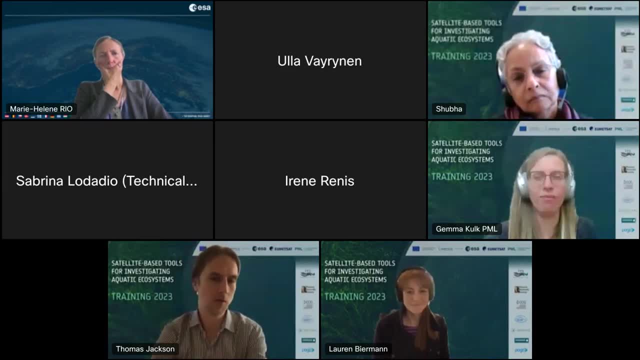 that that was climate quality And that wasn't a fault of the sensor on launch. It wasn't a property that was known. It was just something that we got through regular monitoring of the input data streams. So, yeah, you have to keep checking everything all the time. 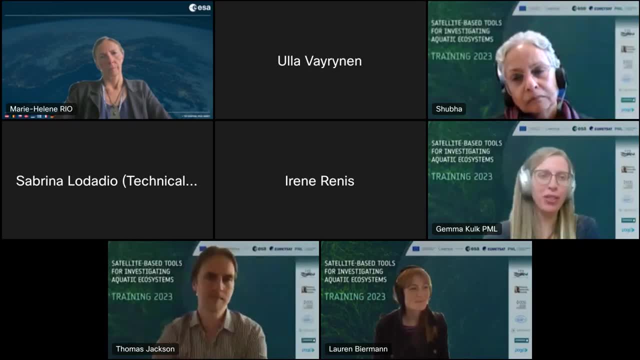 Thank you, TJ and Lauren. There's a question about the uncertainties required for the ECVs. You mentioned that the uncertainty for chlorophyll A from satellite observations is 30%, And one of the participants actually commented that that seems quite a lot. 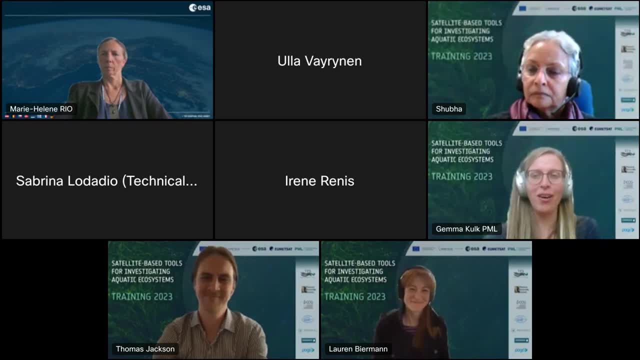 Is that only for complex waters, And do you think that's an acceptable uncertainty? 30%? So that's not. sometimes we do better than that. That is the requirement that we should. basically that should be our maximum. So definitely, I would say that the accuracy 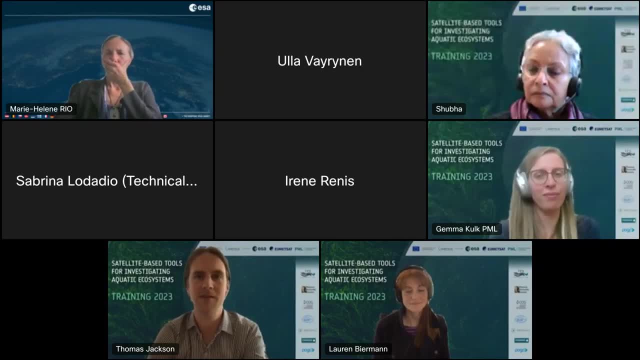 I think is in some cases is better than 30%. Yes, it gets trickier in complex waters, but also the tricky element can come in very clear waters where your signal to noise becomes very low. So if your absolute chlorophyll concentration 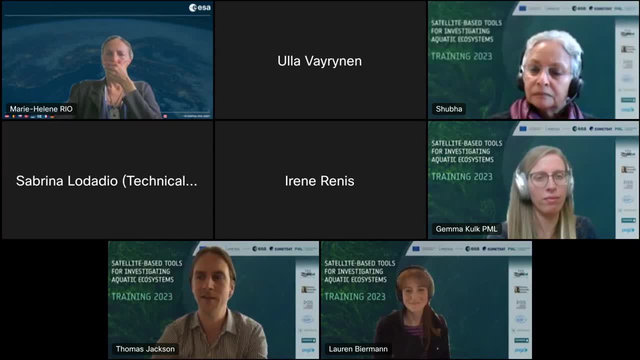 when you go out and measure it with an in situ sensor is 0.01,. you know, a 30% difference is not a lot In absolute terms, So that requires a very high level of sensitivity. So yeah, the 30% value was agreed by the community. 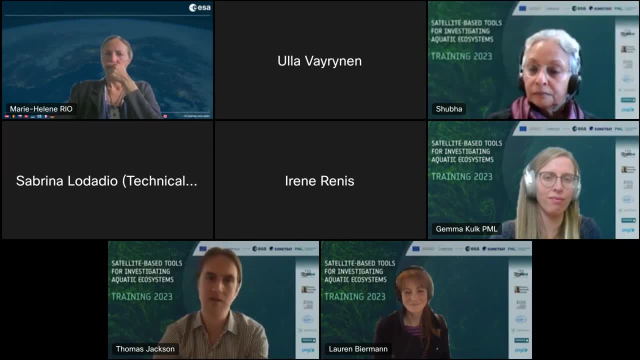 There are definitely places where we I think we do better. There are some places where we still aren't meeting that requirement in very complex waters. But yeah, it's something we strive to keep improving. Thank you, TJ. There's also a question about what ocean colour. 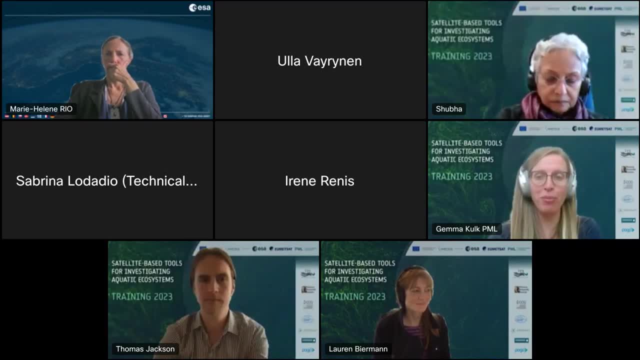 satellites can observe and what the future might bring. So the question, one of the questions was whether we can measure subsurface chlorophyll maxima, And a question related to that is: what do we need to measure that using satellite observations? That's a tricky, I mean. it depends on what you mean by subsurface. So the satellites are integrating most of their signal over the first optical depth. in some waters that can be tens of metres. So if you had a peak that was at 20 metres you might see some of that signal. 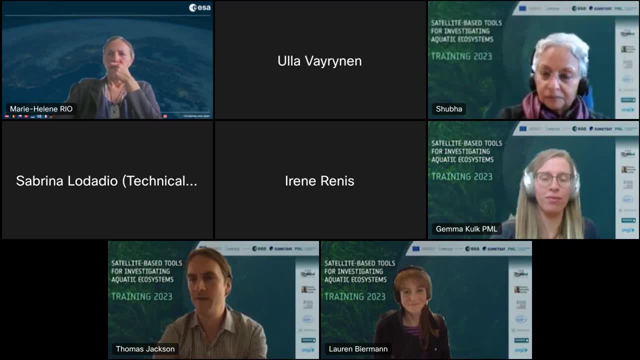 if the waters above it are very clear. And in terms of actually locating a subsurface peak, that's going to require something like lidar, which there are plans for and will be very interesting, But, yeah, resolving the actual vertical structure from the existing ocean colour record. 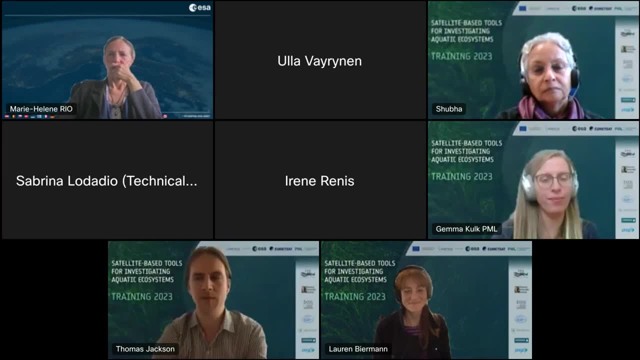 there have been some attempts. Often it comes down to some assumptions or statistical relationships between measured profiles at given locations and surface concentrations. So normally it's kind of a modelled output. But for direct measurement lidar would be the best tool, Also combined with BioArgo. 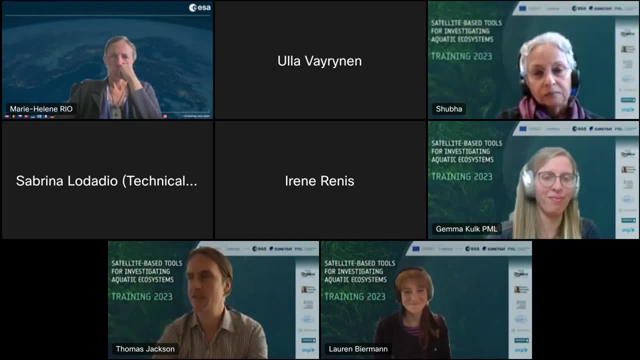 Yeah, so there's a 4D dataset. So there's a dataset that's been produced called- Maria Lem will know the name. I think she helped produce it- MultiObs. There's a MultiObs dataset which they have taken: satellite chlorophyll. 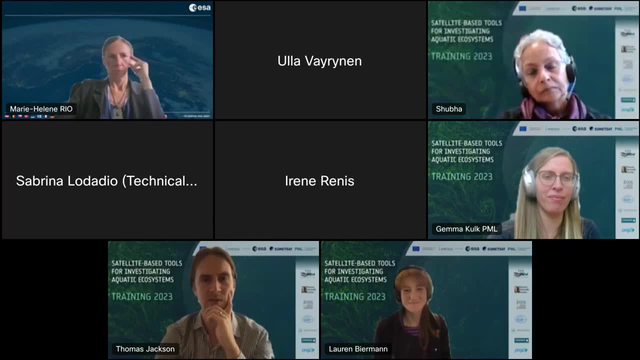 and tried to combine that with BioArgo floats, which have measurements of the vertical profile, to create a 3D dataset. What I think I and a few others would like to see in the future is potentially combining the BioArgo with the climate merge dataset. 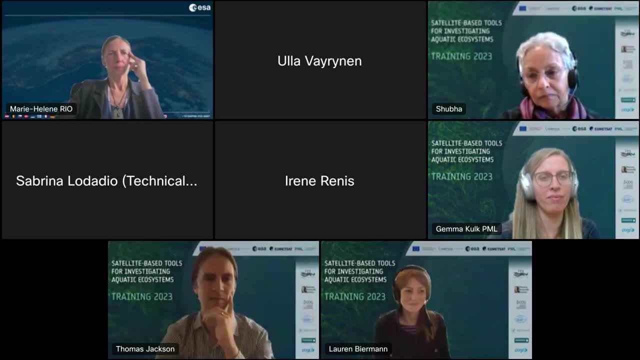 to get a merged input to the top of that surface field. Thank you, TJ. There are two more questions left over. I am also aware that it's almost the end of our Q&A session lecture for today, So one of the questions is whether we'll find places. 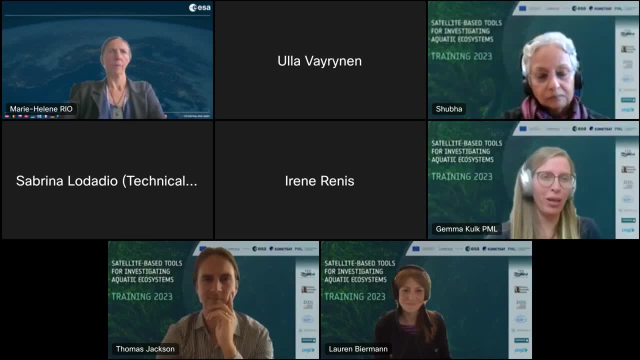 in the near future where phytoplankton will no longer be able to grow, and whether there is research in this or publications in this- I mean no phytoplankton at all- is quite a bold statement. They are remarkably diverse in their ability to deal with salinity. And I mean you know you go to everything, from a horrible looking pond in a garden through to the super saline lakes. you know there's stuff growing in most of these things. I mean the salt evaporation ponds that they use to create things like potash. 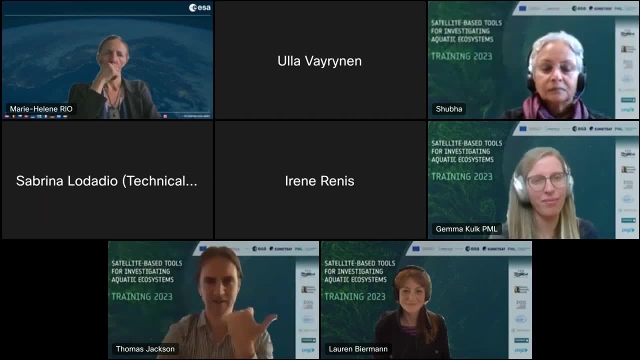 they have to put copper in them exclusively to make sure that they don't go green. They want them to be not populated. So I don't know if saying there are places, through climate change, that will be completely absent, but I think there could be such significant changes. 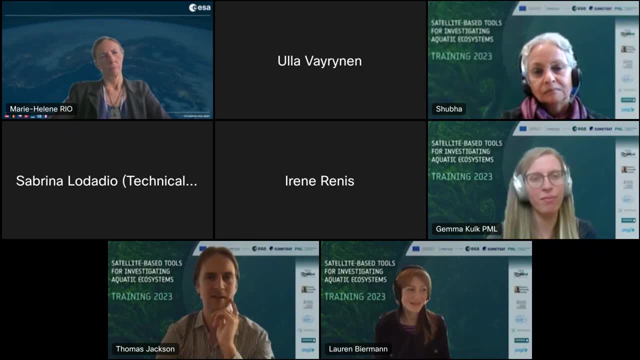 that the whole ecosystem has to shift, And that's the important bit. I think this relates to the last question as well, whether you can mention some negative impacts on marine ecosystems and if there are any measures in place to control them. I mean, yeah, negative, a lot of. 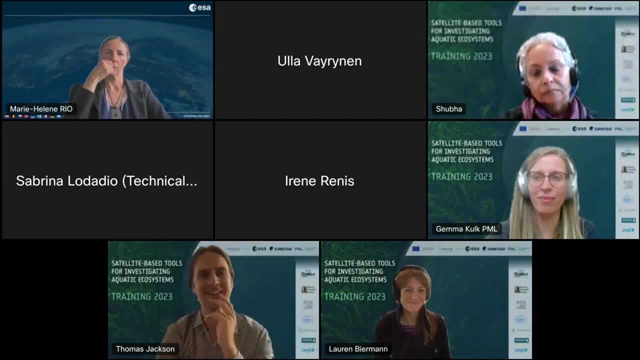 A lot of changes are negative or people view change as negative. It might be that in some cases you know an area is going to become more productive and the fisheries might boom, But in terms of negative impacts, definitely key, I think, or prominent ones. 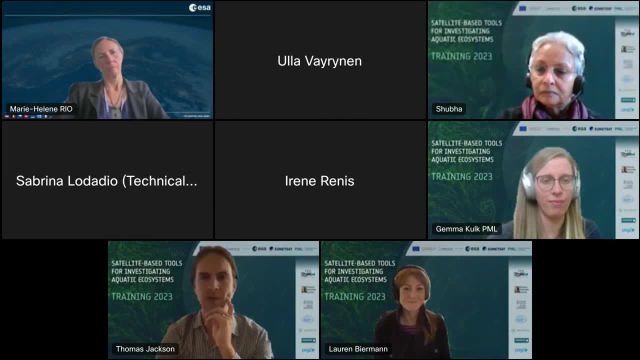 might be changes in harmful algal blooms, changes in stratification leading to, you know, changes in the amount of food available at trophic levels. You can have things like cyanobacterial maps, which can be toxic, all sorts of things. 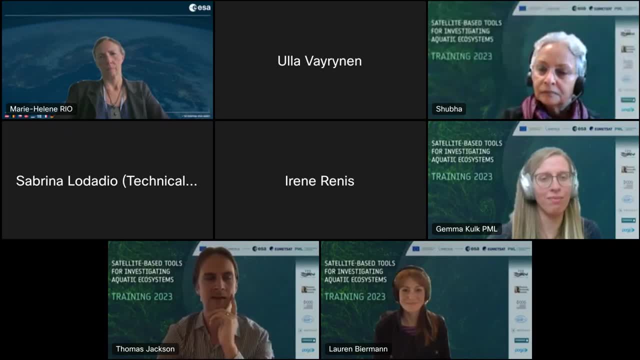 So I think really I'd wait for maybe Heather's lecture on community structure and you'll start to see how important those shifts could be. That's where we'll probably see that. Thank you, Teejay. That's what our questions are for today. 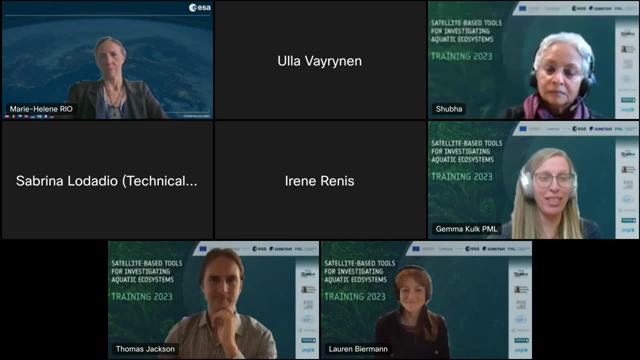 So thanks a lot again for both Teejay and Marie-Helene for presenting their work, their work. Shubha, do you want to say something? I would like to add a point, if I may. It is related to a question that Tom. oh sorry, am I muted? Can you hear me? I can hear you, Okay. 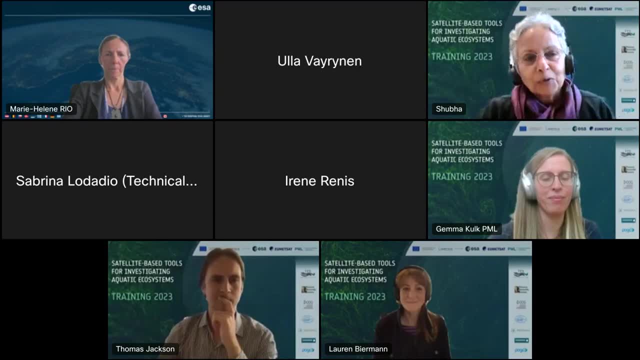 good. There was a question about whether we are all parochial in our attitude to which data we will use. Tom has already replied to that, but I would like to emphasize that the climate problem is too big for us to be possessive about which data was produced by whom. 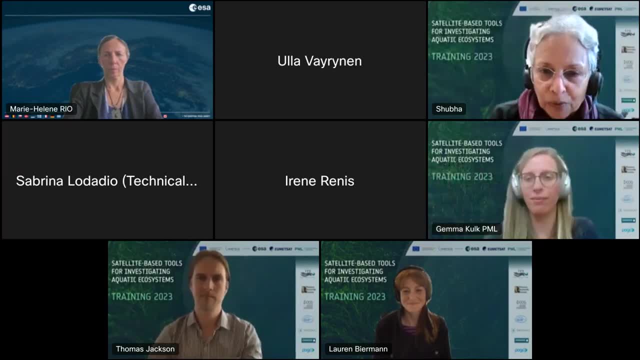 As Tom has mentioned, we go all the way out to make sure that we use all the data available that have the right quality. NASA does the same. If you go to the NASA website, you will see that you can find ESA data and data from other space agencies. As Tom said, we are all parochial in our attitude to which data we will use. If you go to the NASA website, you will see that you can find ESA data and data from other space agencies. As Tom said, we are all parochial in our attitude to which data was produced by whom. And remember too. 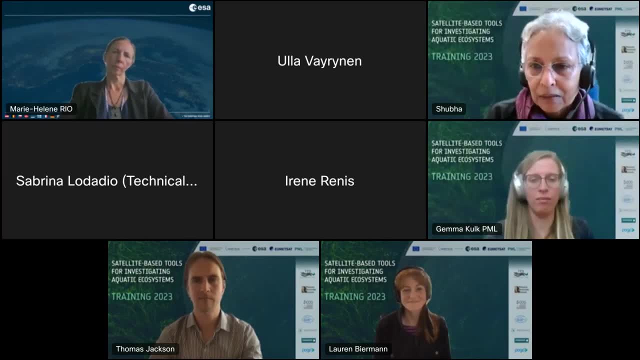 that ESA and NASA are not the only players in this field. There are a lot of valuable data coming from other space agencies, including China, Japan, India and I'm probably forgetting some others. Actually, there are also European countries that have their own satellite sensors. 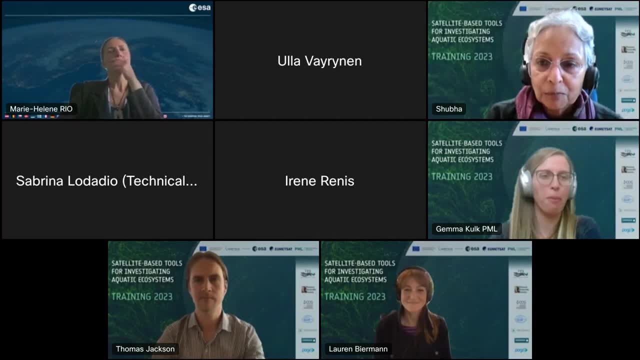 So if you are serious about the big questions of the day, you can't afford to ignore any good quality data. I just wanted to really emphasize that point. Thank you, That was my intro. Thank you, Shiva. Thanks again everyone for being here and enjoy the rest of your day.